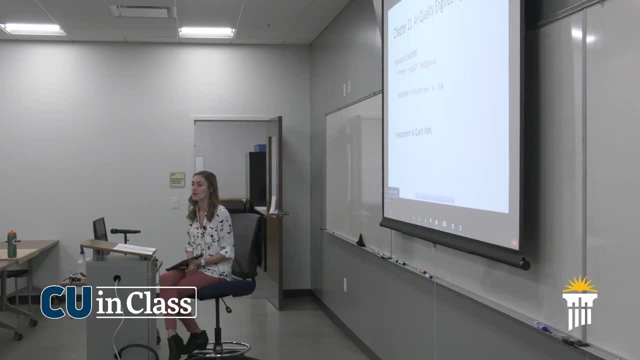 So we'll talk a little bit about ozone- That's one of our major secondary pollutants- And we'll talk about smog. So those are key ones that we actually tend to be pretty familiar with when we're talking about air pollution. But overall those are our big secondary pollutants. We still need to have regulations for them, But they're a little bit more difficult to regulate. They aren't immediately emitted into the air like our primary pollutants are, So that tends to cause a little bit sometimes of an issue, Or at least it's a. it just causes a little bit of a challenge for us to be able to regulate and effectively treat those. 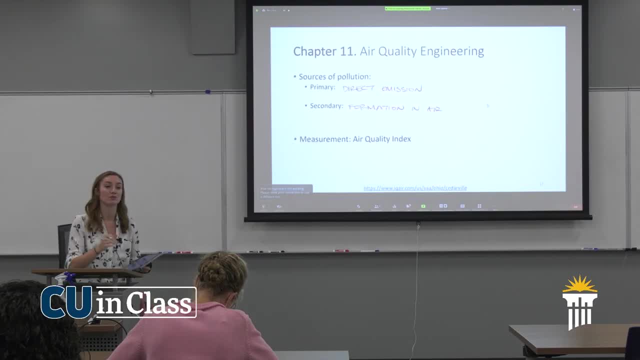 And the next thing is how we do this. We use what's called the Air Quality Index, also known as the AQI. So different companies, the government- keeps track of air quality indexes, So I found a site called iqaircom. 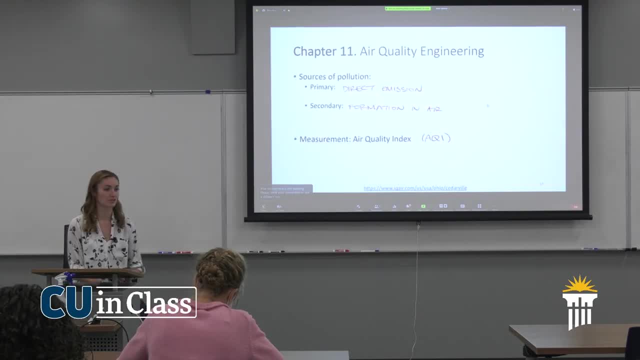 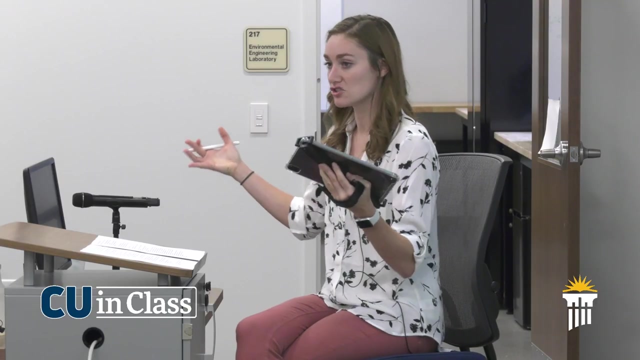 There's also EPA governmental sites. iqaircom actually happens to do global things, So we'll look at that momentarily. But our Air Quality Index is relating our daily air pollution concentrations for our criteria- air pollutants measured in a particular geographical area- to concentrations of our air pollutants overall. 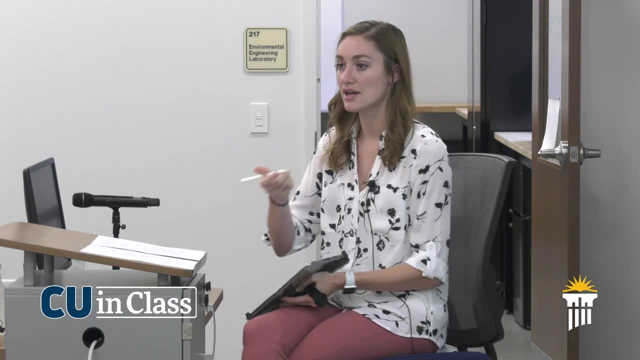 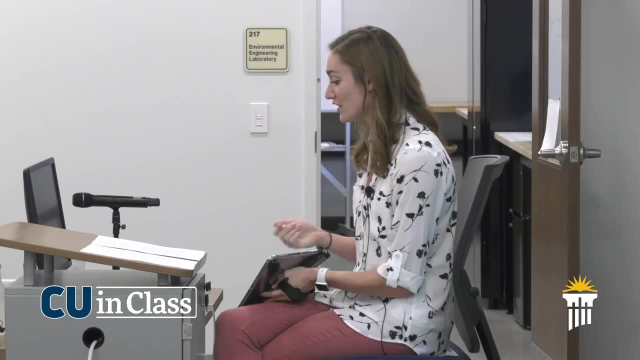 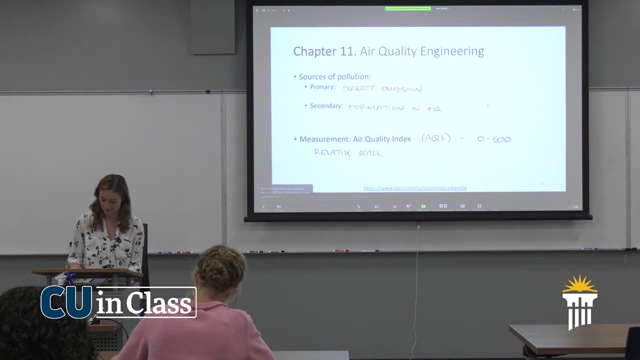 So it's a relative number And the numbers here are just a few. Generally it's 0 to 500.. By generally I mean that is the range. So it's a relative scale. And a key bit of this is it's a number, it's a dimensionless value. 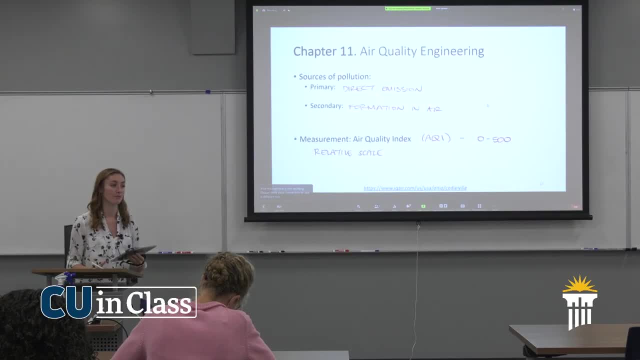 So when we are talking about them as this like combined number, we're not necessarily looking at: how much exact carbon monoxide do we have? how much exact ozone do we have? how much exact particulate matter do we have? Most of the time, that's a combination of all those. So we get this really unhelpful value in one sense because it's like 2.. What does a 2 mean? A 2 is actually really good. Most places don't have an air quality index of a 2.. Most good air qualities hover around like 15 to 30 or so. 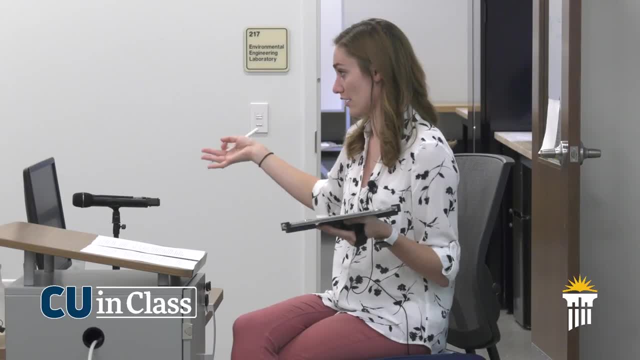 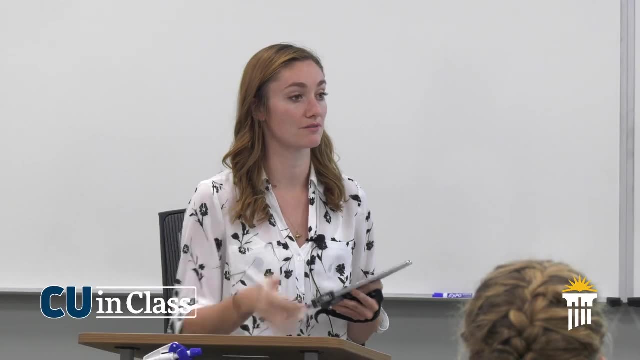 And as you increase in your number, you're getting worse air quality. And it's a combined number, 0 to 500. It's a combined number of all of our criteria. air pollutants that are contributing. Yeah, How do you measure something? 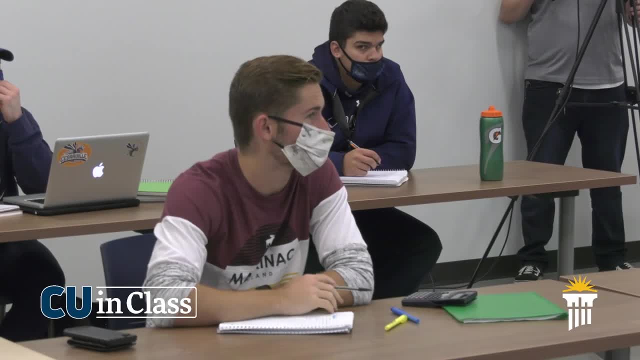 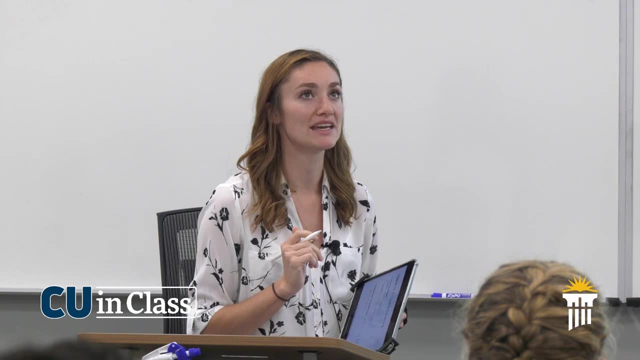 How do you measure something That's like dimensionless? How do you get that number? Other people have done empirical formulas to figure out what this number is and to make it usable. So it's not just a number that sits and is like, okay, well, what does 500 mean? 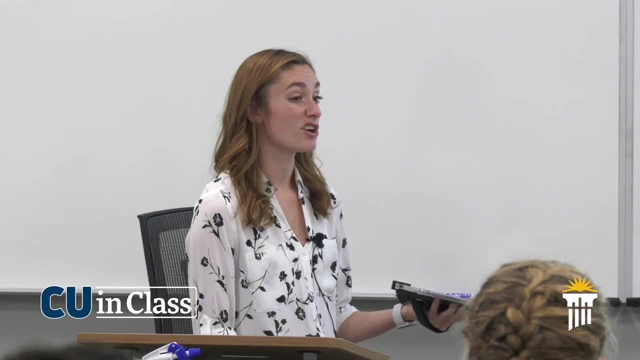 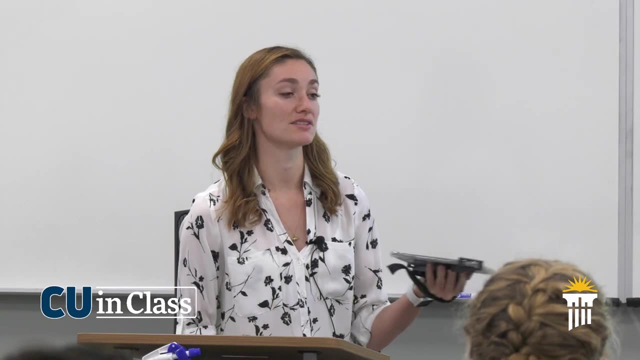 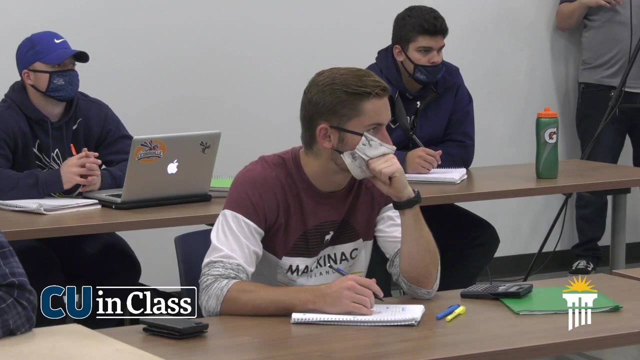 They are considering how much ozone contributes to human health. The tropospheric ozone contributes to human health. How much CO2? How much CO2 contributes to human health? So there's some factors in there that are probably a little bit past this class that actually go into what the real number means. 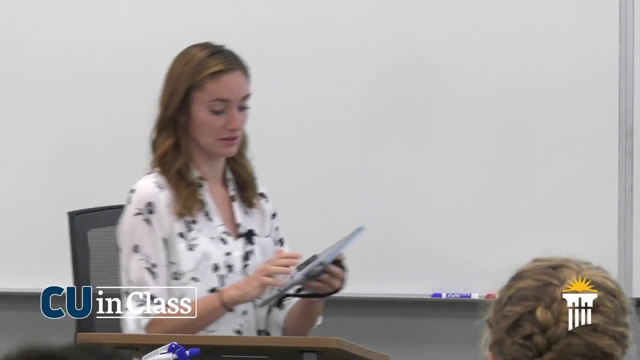 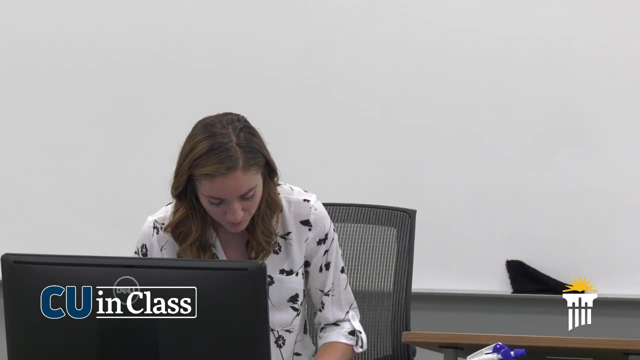 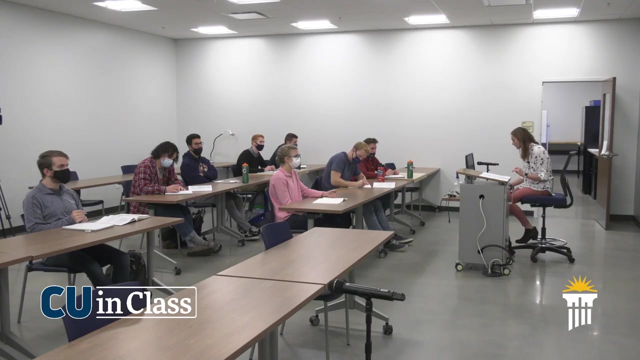 But we are actually going to look at this particular site because it's quite fun, Or I think it's quite fun. You don't have to think it's quite fun, So let's bring us back over here. Okay, We're going to share this one. 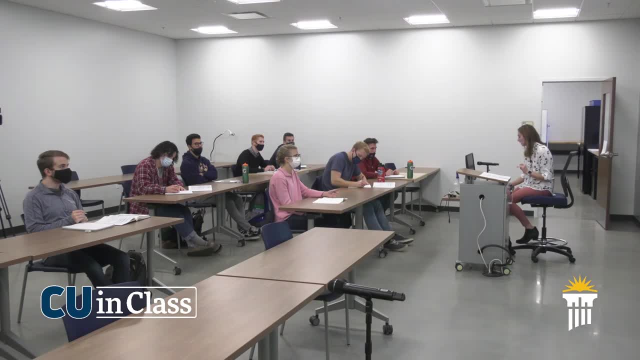 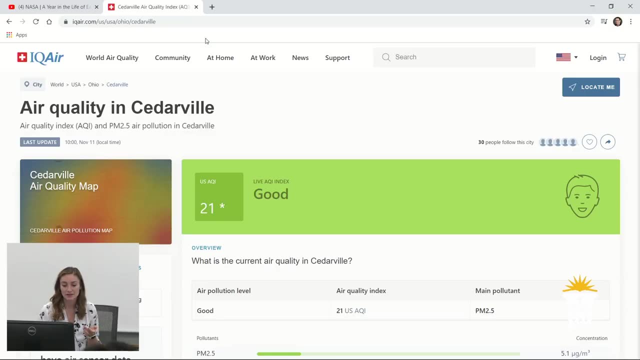 Yes, Awesome, Okay, Okay. So this is Cedarville's. So this is on IQaircom, up at the top. This is our air quality today. It was taken at 10 am, November 11th, And in this particular site we can look at the USAQI, which is how we're measuring it. 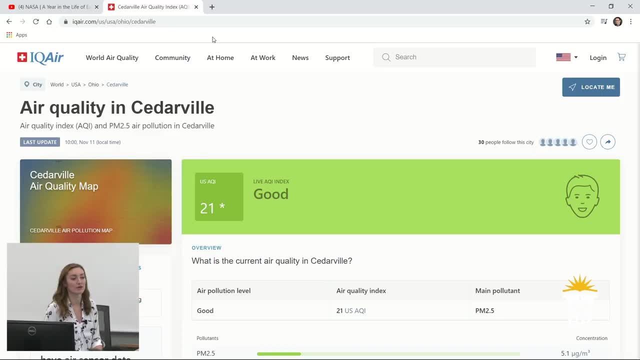 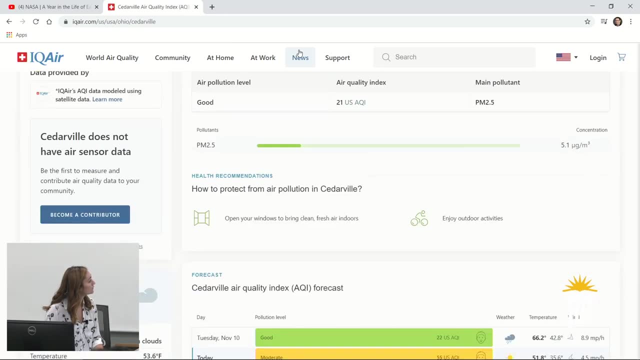 So we're at 21,, which is really good. That's why it's green and it says good. We like that. Green generally means good And you can look at these other factors in here. So the pollutants that are contributing to today's maybe poorer quality of air, but it's not really poor quality. But the things that are basically making it not zero are PM2.5.. So we have some dust particulates in the air. Honestly, it's probably because we're in corn harvesting season And so there's a lot of corn dust that's around. 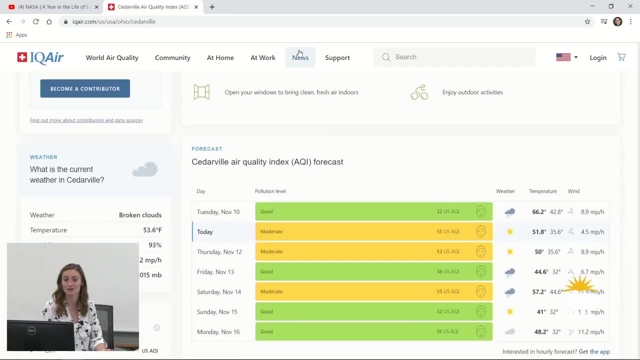 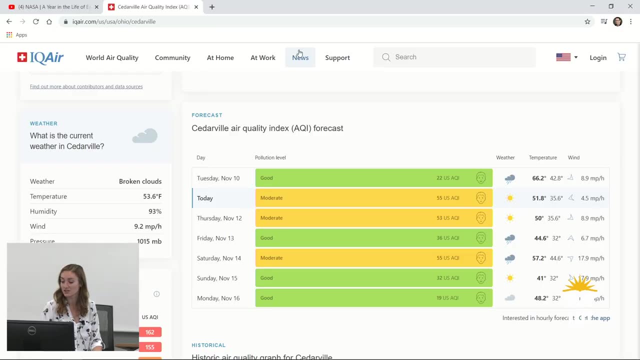 It doesn't look like they're doing a whole lot of corn like removal today. Otherwise our pollutant level might be a little bit higher And it can give us our concentration. So I'm not actually sure where they have measured this specifically from. 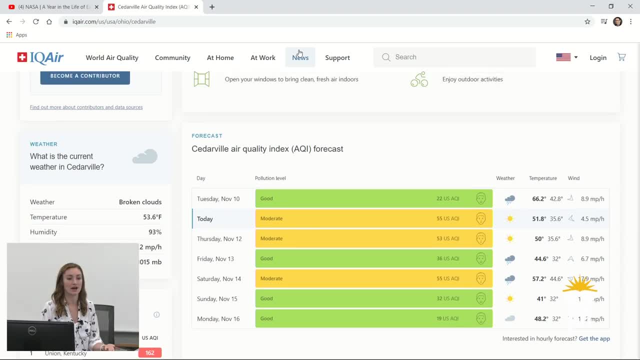 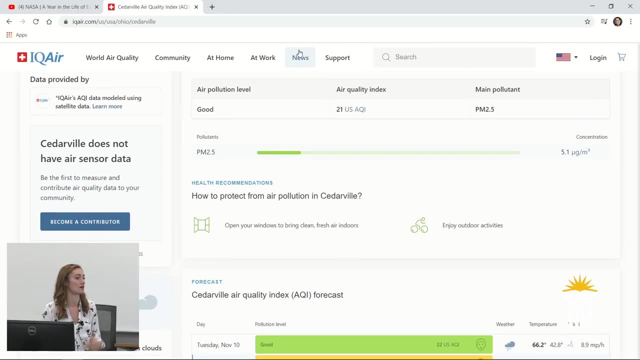 But someone is doing some measurements here, or at least tracking it, maybe in the Dayton area, And then they're projecting it onto, basically based on winds and that kind of thing, from what happens in the Cedarville. But you can look at all these. This has a projection. 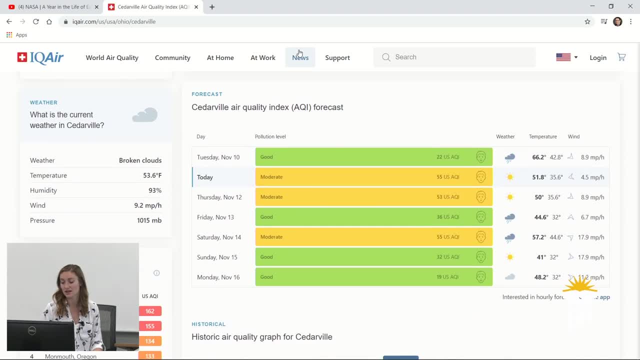 So it has our forecast of what we expect it to be. So today our high is at 55. Tomorrow it will be similar, But we're in pretty reasonably good air quality deals If we come over here to what they're calling the pollution map. 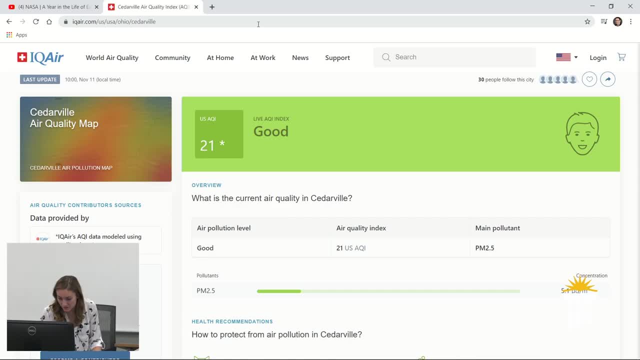 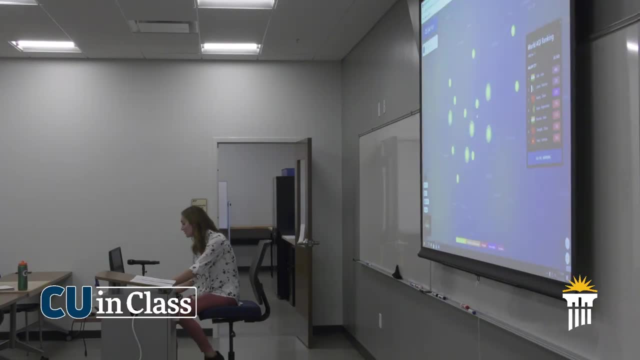 This is showing us all the surrounding area. So here is Xenia. Cedarville is a little too small to actually be on this map at this level, So we're just going to keep zooming out. Find your hometown, Find places that who's from Boston? 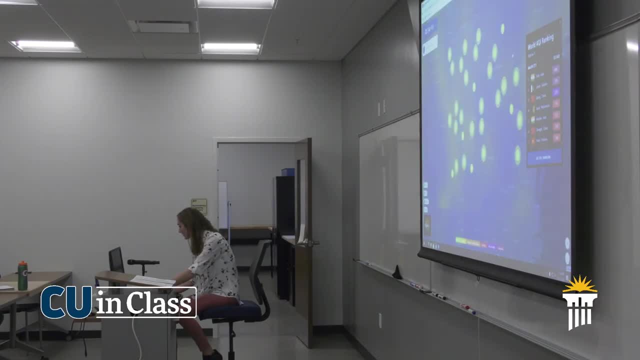 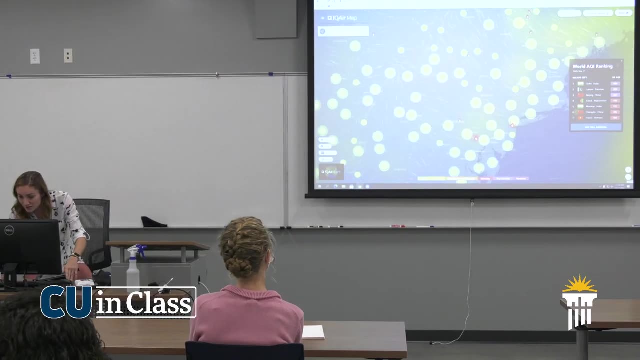 Kai. Yeah, I was looking at Boston the other day. I had higher expectations of Boston. I thought actually that you would have worse air quality than you actually do. Where is it? I'm not actually good at finding things, Sorry. I expected Boston to have worse air because it's a city. 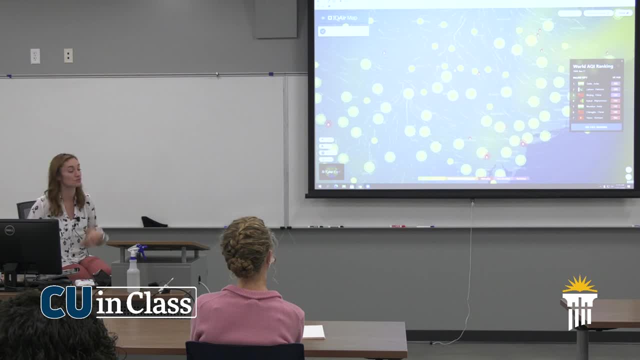 But it actually looked relatively fine. So there's a lot of things going on on this map. So the little white streams are wind. You can see there's fires that are noted, So fires actually significantly contribute to our air quality. If any of you guys have been around fires or been in ashy areas, it's very unpleasant. 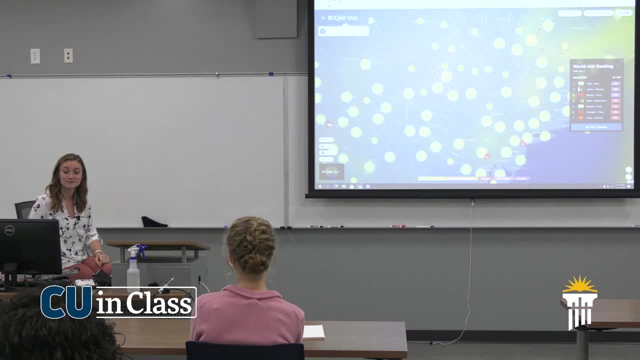 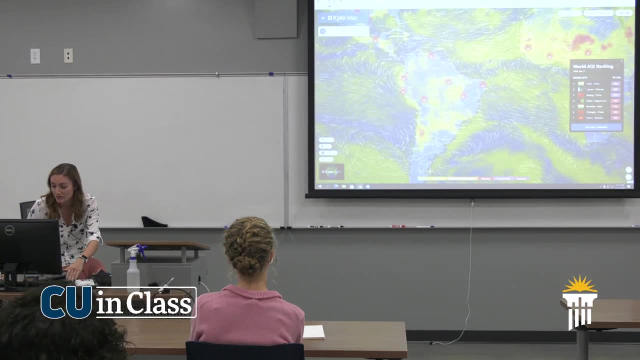 What about the fires that are in the Amazon? Let's go down and see. They actually do the entire world down here. So you mean, like these fires All down in here- I don't know how to say any of these terms- You're going to have to help out with that. 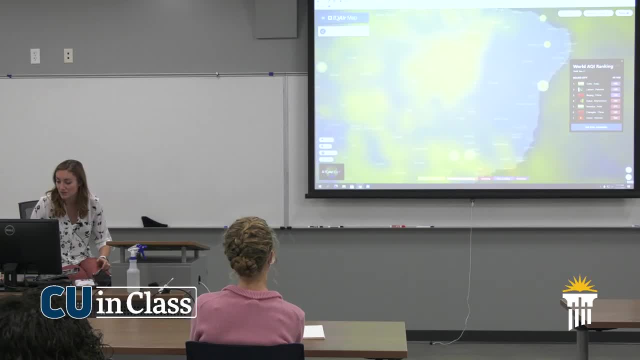 But yeah, So there's a ton of fires down here And actually it doesn't look like they're significantly contributing because our air quality is generally not super terrible. Like we have 12,, 6,, 42. If we're on a scale of 0 to 500, like these are actually pretty solid. 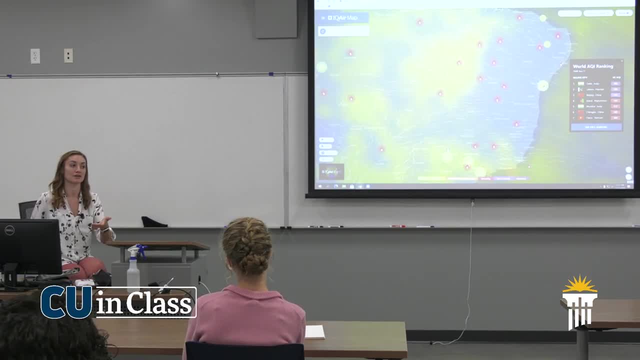 So maybe we aren't measuring it as attentively as we could, But it's not that bad, Because you can see there's lots of fires in here And there's not a lot of station points with 12 and 6 and maybe 15 over here. 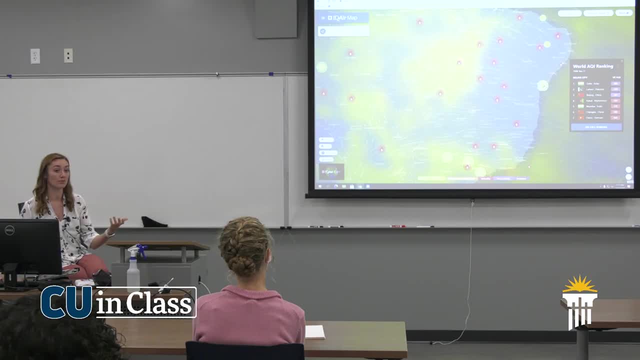 So we don't have a lot of points that we're actually getting, But potentially that means we could do a little bit better job of actually getting those. If we come over to Africa and Europe, especially looking at India, India and China tend to 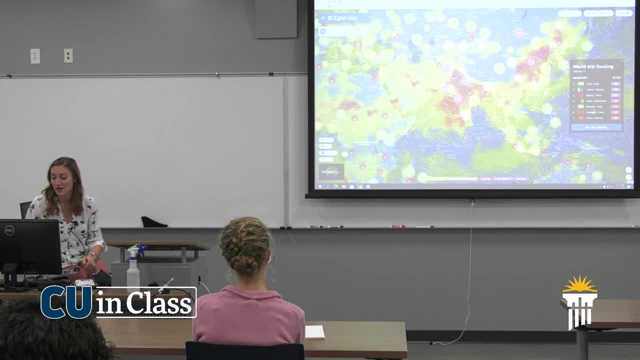 have really really poor air quality, just as a rule. So you can see in here 211, 213.. This is over in our Uzbekistan's area, Uzbekistan, Afghanistan, all those. So those tend to have really poor air quality, in part because they have different regulations. 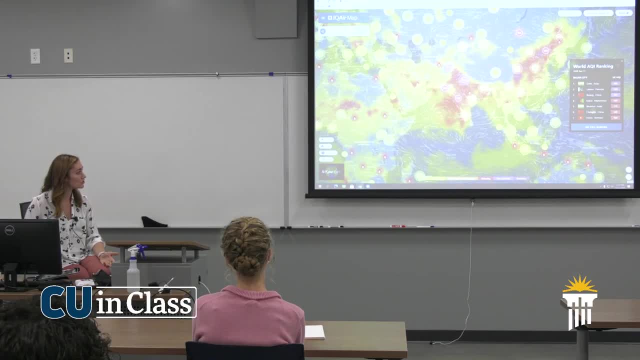 than like what the US has, And they also. they have different geography, So how the wind moves along the land over there looks a little bit different. Therefore, when it has poor air quality, some of it sits a lot longer than it does in the 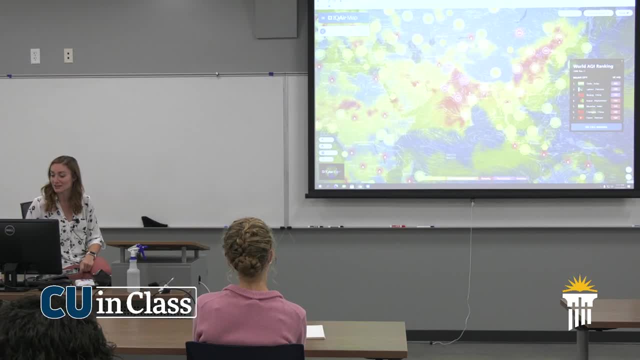 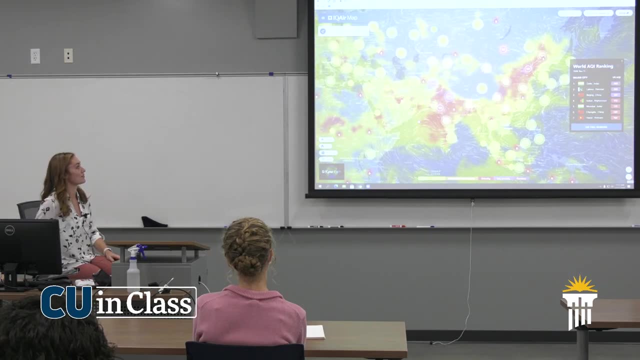 US, where we have a lot of really open plains, China looks a lot different. China looks a lot different too. They definitely have some different regulations, But you can see, this is a. I actually really liked this resource. It was better than what I thought some of the government resources were, because it does. 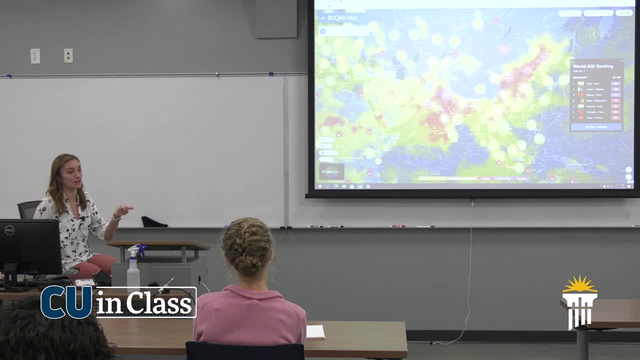 the whole world, But so this will be online if you guys just want to check it out afterwards. But this is kind of an example of what our air quality index looks like worldwide, internationally, overall, all of those things. Yeah, Can you explain again how to get that number? 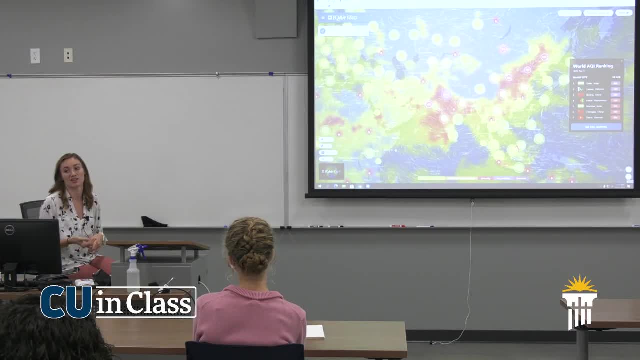 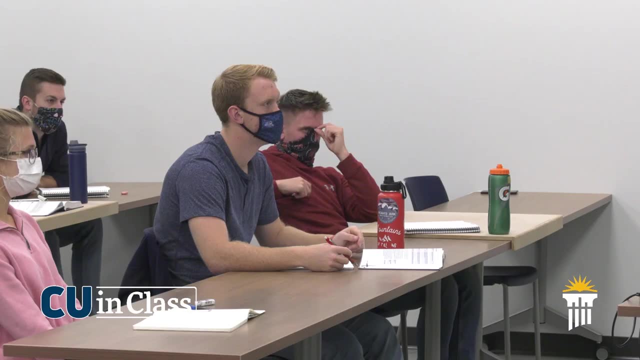 So it's a conglomeration of all of our criteria: air pollutants. So we're looking at ozone, we're looking at CO2, we're looking at methane- all of those that are contributing to what especially particulate matter, what contributes? 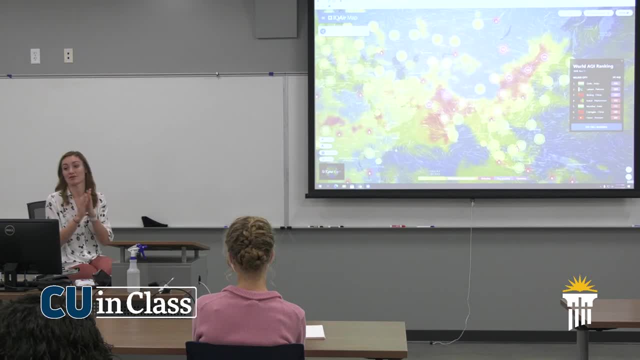 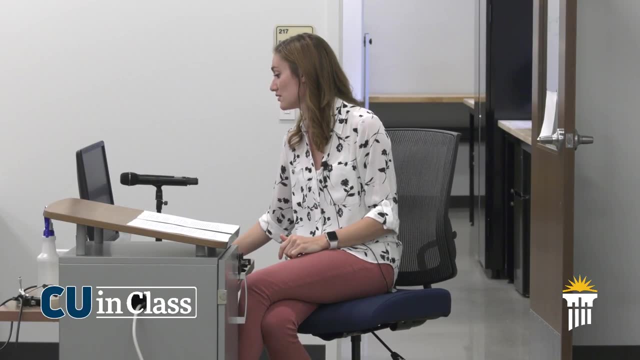 So I don't have the empirical formulas for how we're going from 0 to 500 and the exact number there, But someone has come up with an empirical formula that relates those concentrations. If you want to come over to somewhere in India, 262.. 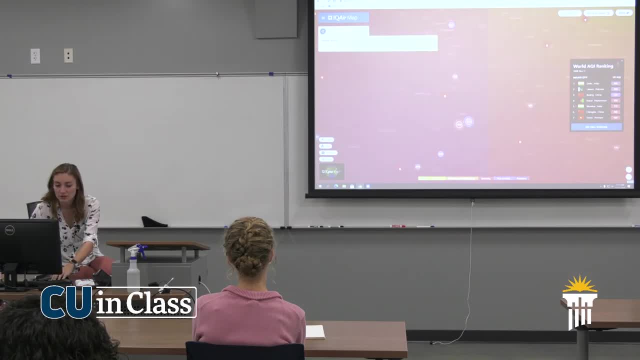 Let's see. I'll actually want to go back to. let's find in India, oh, Pakistan, my bad. So they're at level hazardous over here. That's the city we were just looking at. So their big pollutants that they have. their concentration of PM2.5 is 255.2.. 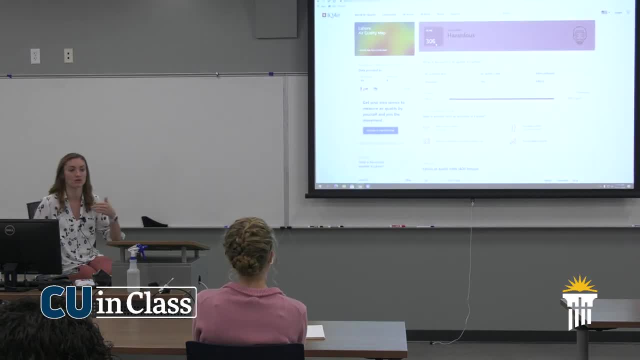 That's not the exact same number as our 306 over here, But there's some correlating factor between their amount of particulate matter that's significantly contributing to their health And the hazardous level of our air quality index. It's really just a helpful value so that we don't have to look at all the individual. 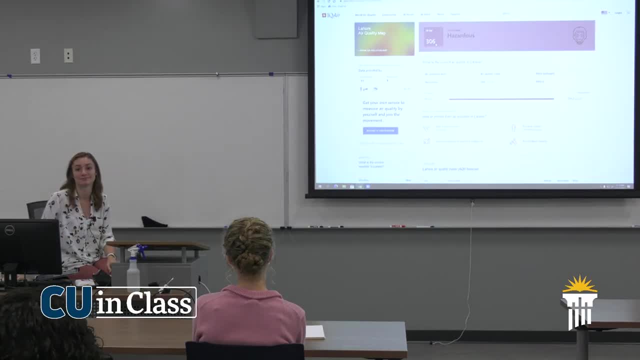 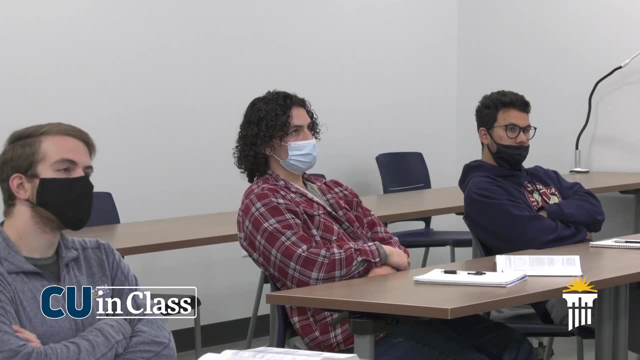 concentrations. Yeah, So like if methane is worse for you, even if there's a smaller amount of it, it could bump the number up. Mm-hmm, Oh, okay, Mm-hmm, Absolutely, Yep, Cool stuff. 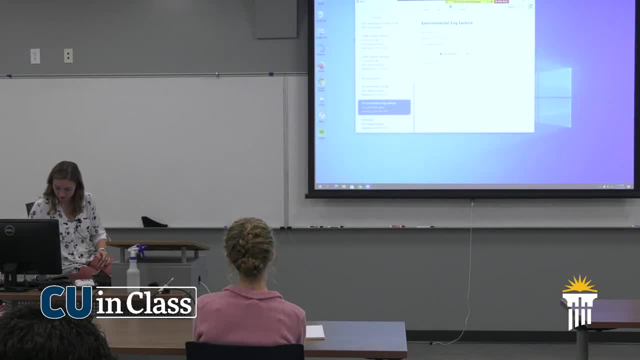 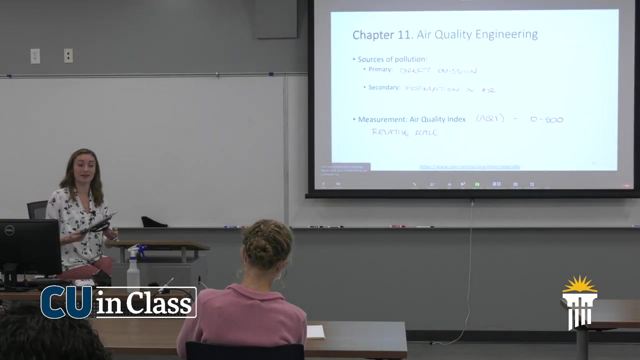 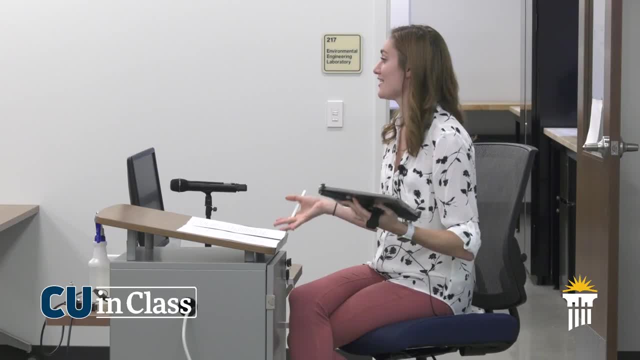 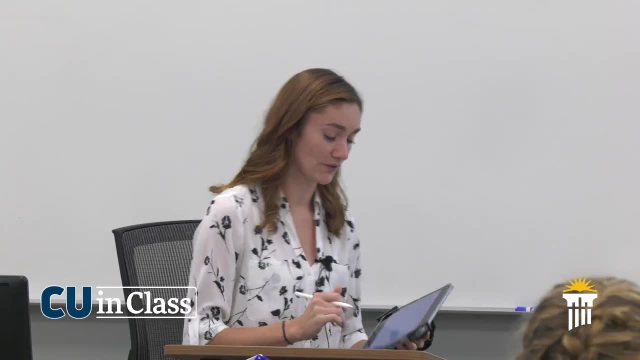 Cedarville probably not as regulated, to be reporting its air quality index or specific values, but Dayton or industries around Dayton definitely would be Okay. So in this, one of our big sources of pollution has to do with photochemical smog. 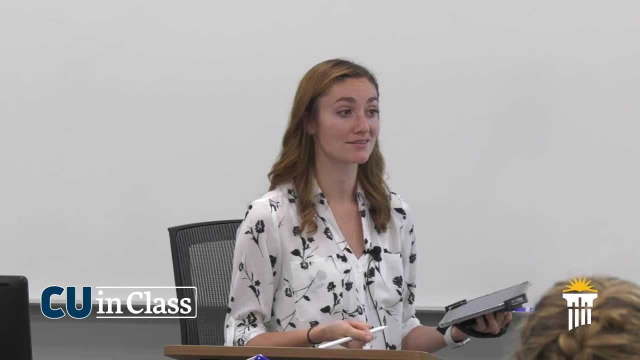 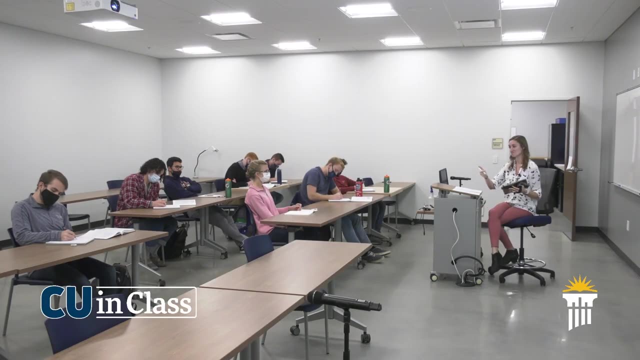 So we don't really call it photochemical smog most of the time, but that's what it is. So the photo portion is talking about photosynthesis and the chemical means. we have a chemical reaction Smog. we'll get to what smog is. 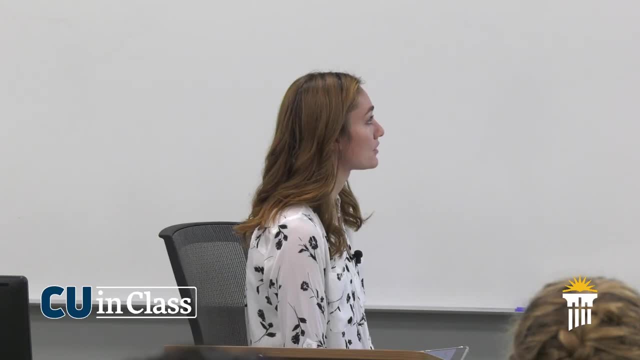 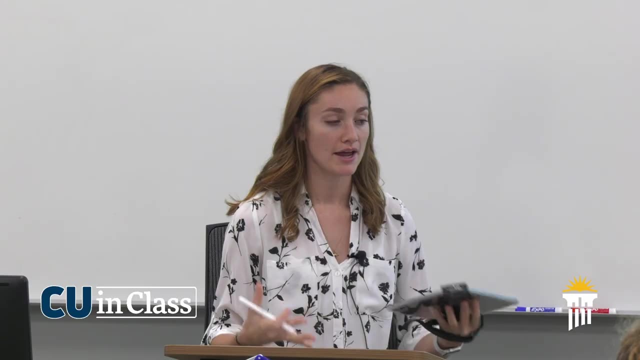 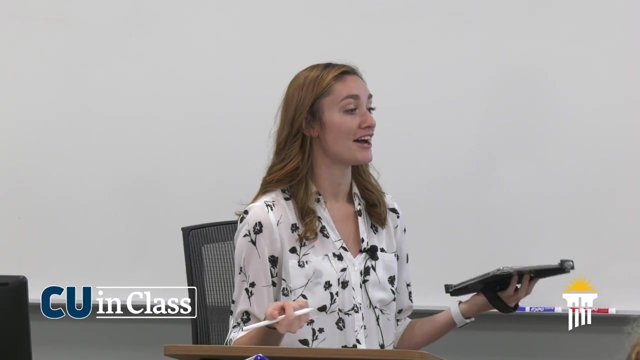 But our ozone is a precursor to the formation of smog, Which is most of what contributes to our overall air quality. when we think about air quality, It doesn't necessarily mean that you're right in your thinking, because there's a lot of particulate matter. there's a lot of nitrous oxides and sulfuric oxides that actually contribute. 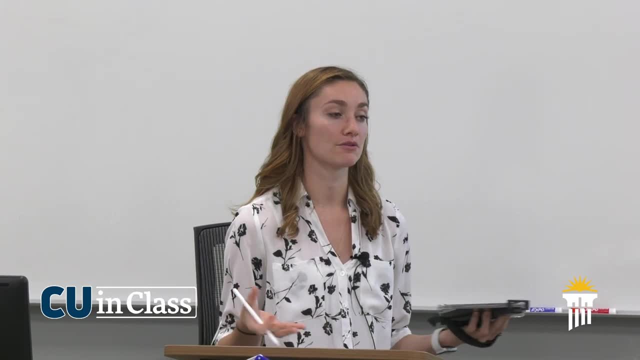 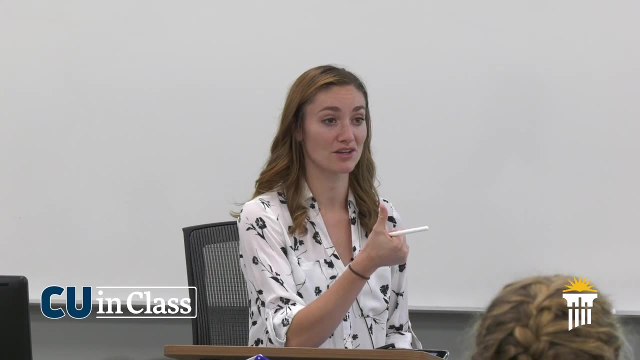 to our air quality as well, But smog does play a really big role, especially in our larger cities. So we're talking about formation of smog, Photochemical, we need to have photo part which is going to be our sun, and we need 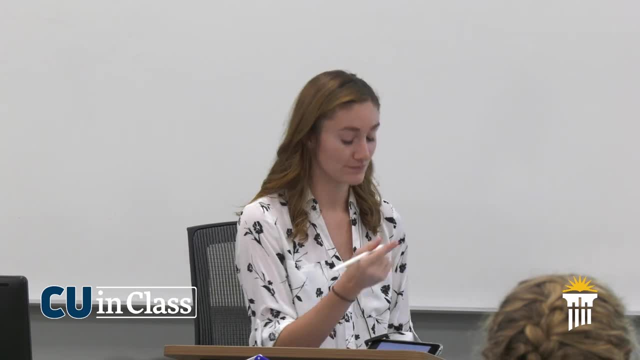 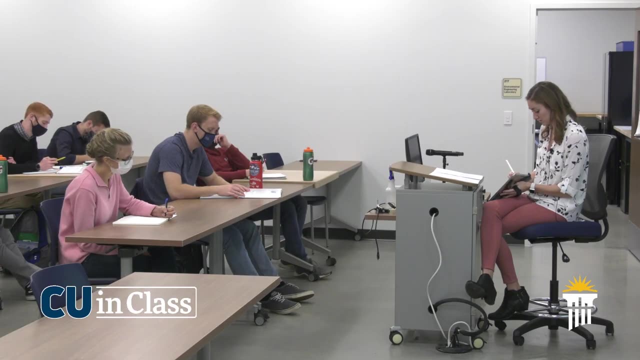 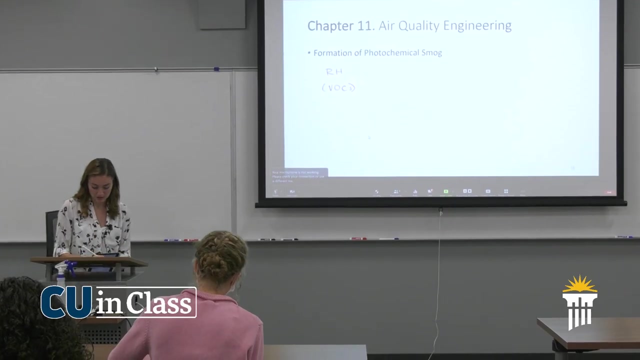 to have the chemical part, Which means we're going to have a chemical reaction. So when we have reactive hydrocarbons, which we talked about these as volatile organic compounds or volatile organic matter, so our VOCs. But reactive hydrocarbons when they add with our NOx, so this is our nitrous oxides in. 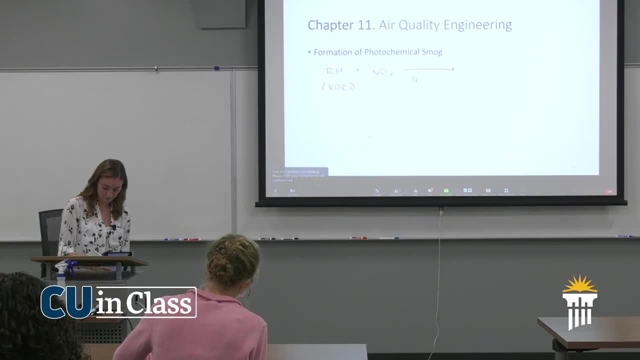 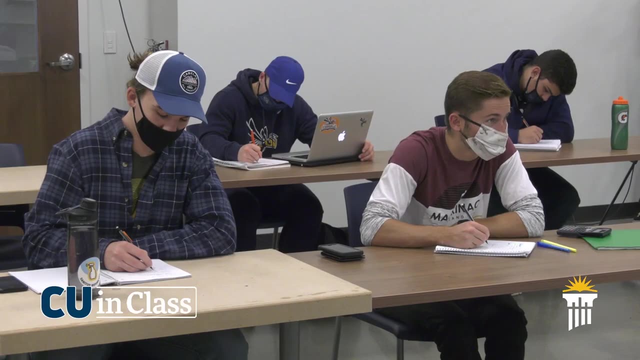 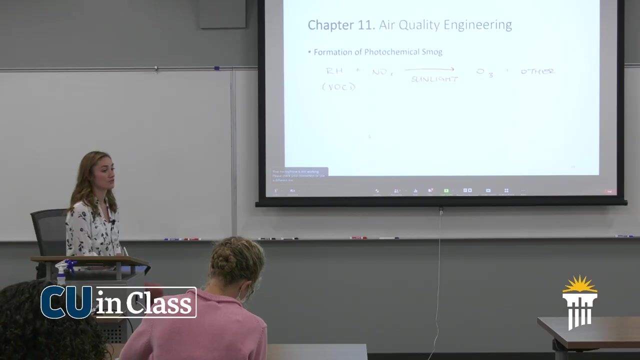 the presence of sunlight they can form ozone and some other things That are important but not quite important enough for our analysis in this class. But the main thing that they're forming over there is our ozone, And we talked about the difference between stratospheric and tropospheric ozone. the other 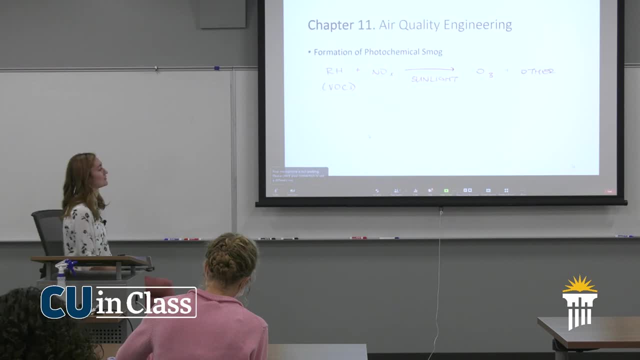 day. So when we look on, this isn't a map but a graph of- maybe I changed the page. there it goes, So the height, basically from the Earth. So down here is our Earth's crust. The troposphere is comprised of, really the first, like 10 or maybe 15 kilometers above the Earth's crust, And then past. that is the stratosphere Past, that we have, mesosphere, thermosphere. We have other things that go up above that. 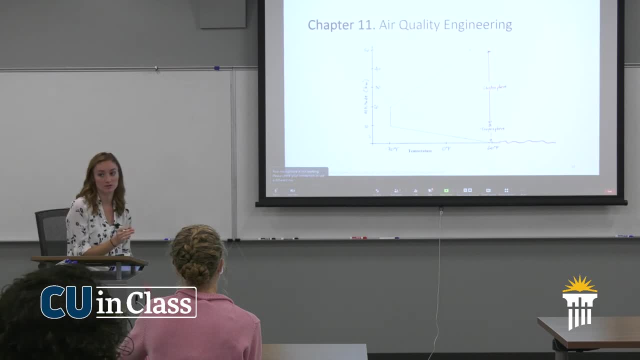 But the tropospheric ozone is really what we're concerned about. We don't really like it to be in the troposphere. That means you're breathing in ozone versus the ozone is contributing to our good ozone layer. So when we have stratospheric ozone, that is very positive. We like that. That contributes to the ozone layer that limits the amount of UV radiation that comes into the Earth. So when we're like there's holes in the ozone layer, it means we don't have enough ozone in the stratosphere. 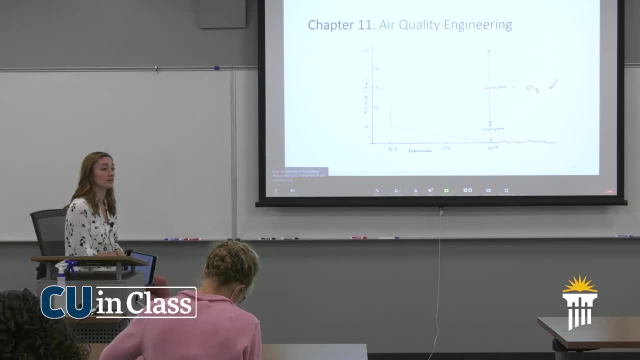 But when we're talking about photochemical smog, it's because we have formation of ozone in the troposphere. We do not like this. This is bad overall. One of the major ways that- and I'm going to go back here- one of the major ways that. 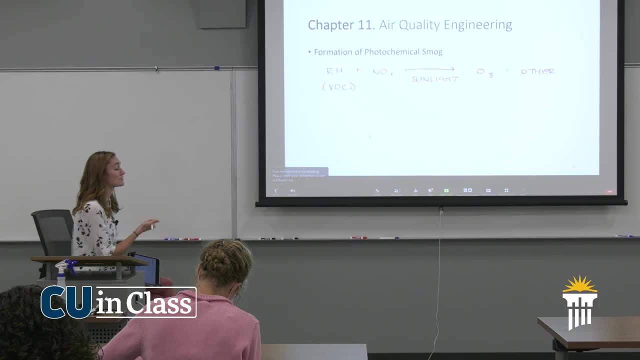 we get our formation of photochemical smog. our VOCs and our NOCs are from incomplete combustion, which we talked a little bit about last class, But that's when we don't have enough oxygen or fuel inside like cars. Cars do incomplete combustion all the time. 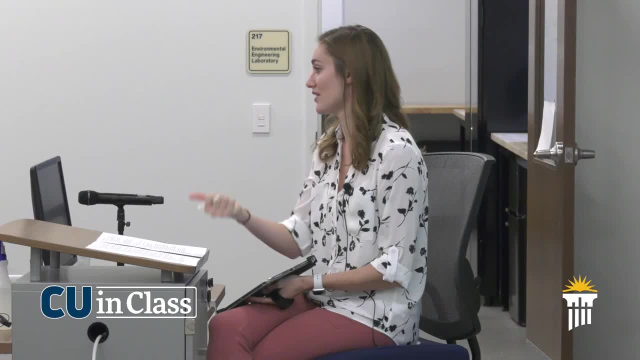 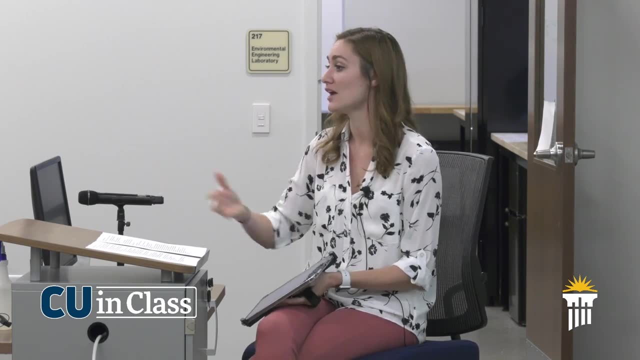 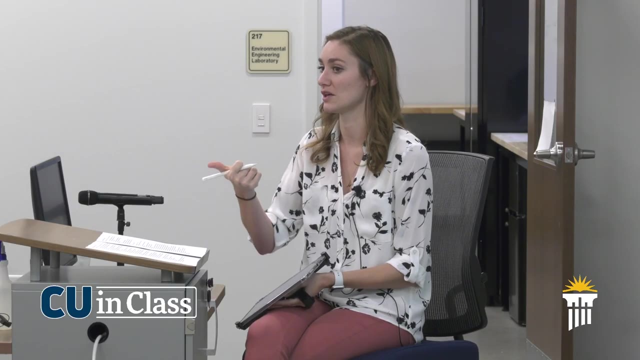 They are designed to do complete combustion, but they can do incomplete combustion. So when they do incomplete combustion, we end up getting these extra volatile organic compounds that shouldn't be there. So for your homework, you guys are reading about the Volkswagen emissions scandal. that happened. Yes, I think so. You should be reading about that. And so that talks a little bit more also about the nitrous oxides that are emitted from cars. So we do emissions controls, especially in cars, because there's so many, especially. in the US We do a lot of emissions controls. Car companies are heavily regulated so that the emissions from cars do not have as much nitrous oxides and other particulate matters, or VOCs. Basically they're engineered to do well environmentally, but sometimes that doesn't happen. So when that doesn't happen and we're in the presence of sunlight- which happens in a lot of our warmer climates- or during our summer months, when we have longer days, we get increased amounts of ozone overall. Generally, that's a problem. 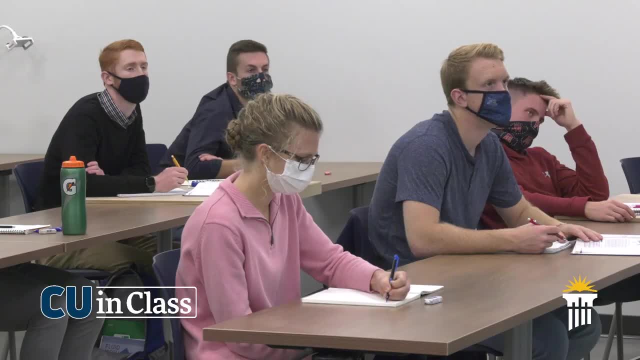 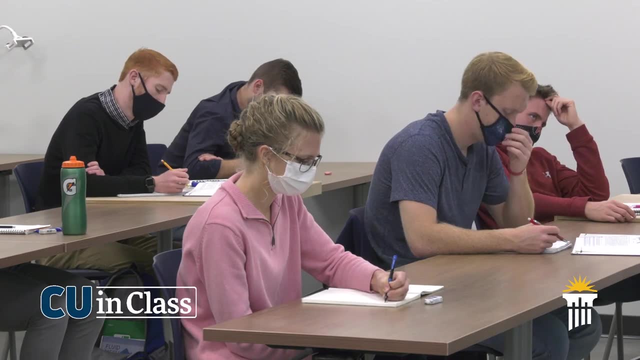 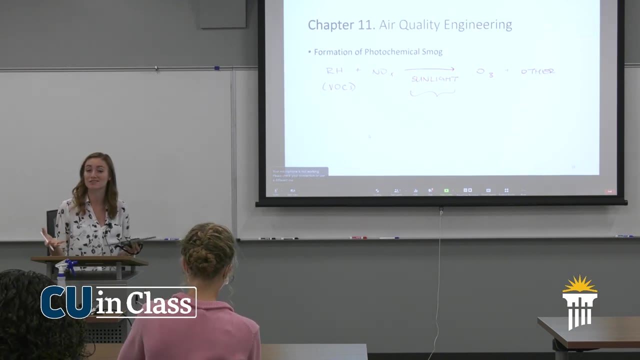 Okay. So we like to avoid that overall, But that's generally when we're forming it In big cities with lots of people, when we have sun, so summer months, or our states that are lower to the equator- Texas, California, Arizona- those ones tend to have heavily smogged. 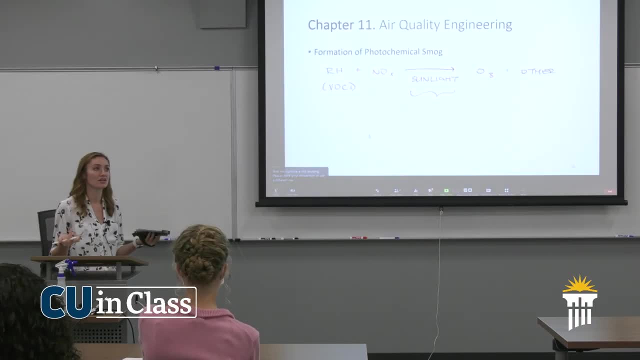 areas, But we also see smog in places like in the Northeast, And so it's not just that you have to have a warm climate in order to form this. You just need these particular parts, which are sunlight, Reactive hydrocarbons and our NOx. 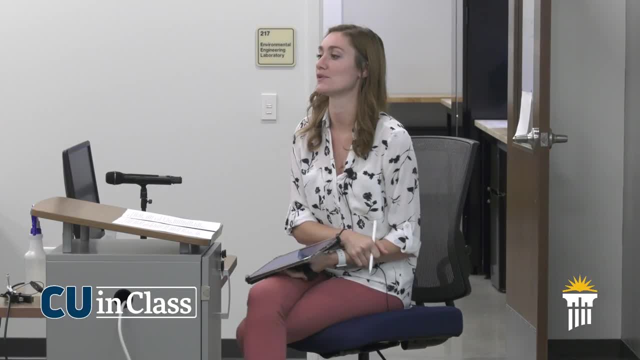 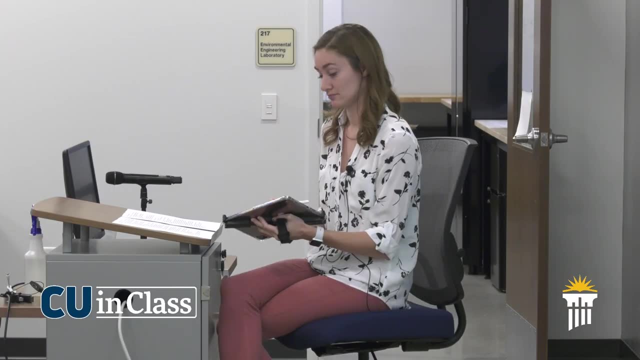 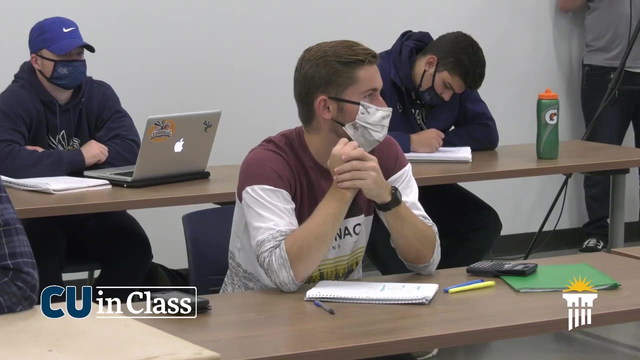 So those form ozone pretty exclusively and potentially to really dangerous levels as well. Speaker 2 Speaker 3 Speaker 4 Speaker 5 Speaker 6 Speaker 6 Speaker 7 Speaker 8 Speaker 9 Speaker 10 Speaker, 11 Speaker 12. 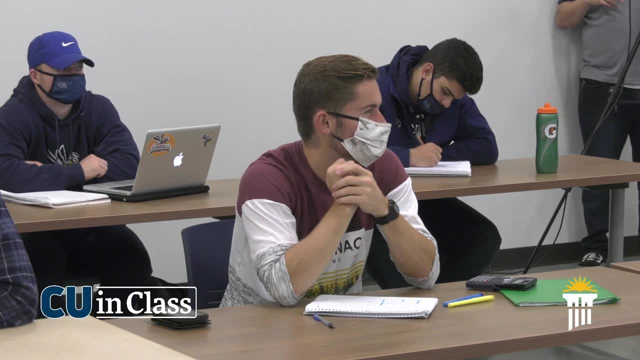 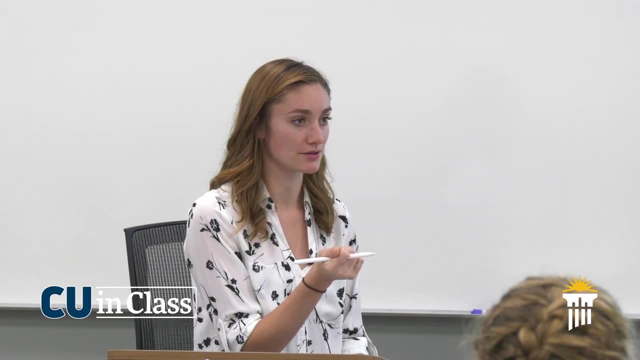 Speaker: 13 Speaker, 14 Speaker, 15 Speaker, 16 Speaker, 17 Speaker, 18 Speaker, 19 Speaker, 20 Speaker, 21 Speaker, 22 Speaker, 23 Speaker, 24 Speaker, 25 Speaker, 26 Speaker, 27 Speaker, 28 Speaker 29. 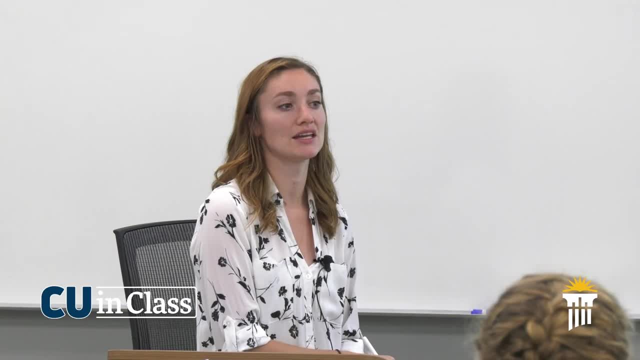 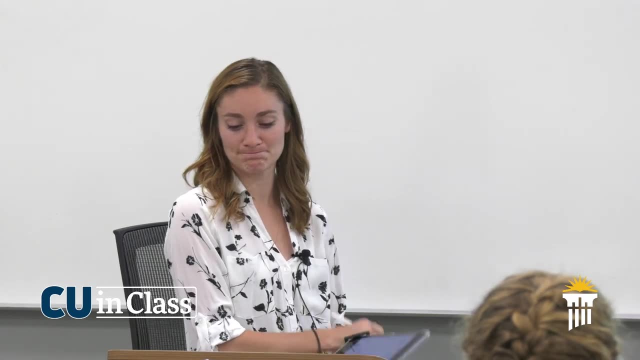 Speaker: 30 Speaker, 31 Speaker, 32 Speaker, 33 Speaker, 34 Speaker, 35 Speaker, 36 Speaker, 37 Speaker, 38 Speaker, 39 Speaker, 40 Speaker, 41 Speaker, 42 Speaker, 43 Speaker, 44 Speaker, 45 Speaker 47. 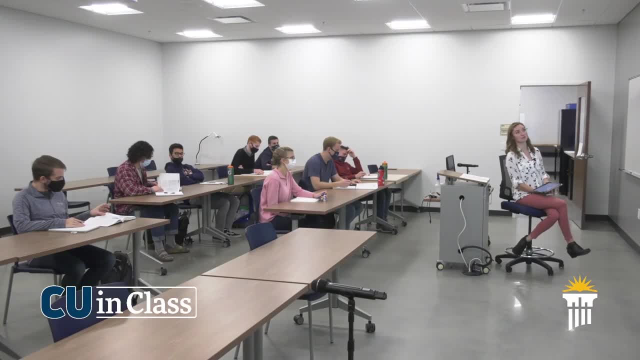 Speaker: 48 Speaker 49 Speaker, 50 Speaker, 51 Speaker, 52 Speaker, 53 Speaker, 54 Speaker, 55 Speaker, 56 Speaker, 57 Speaker, 58 Speaker, 51 Speaker, 52 Speaker, 53 Speaker, 54 Speaker, 55 Speaker 56. 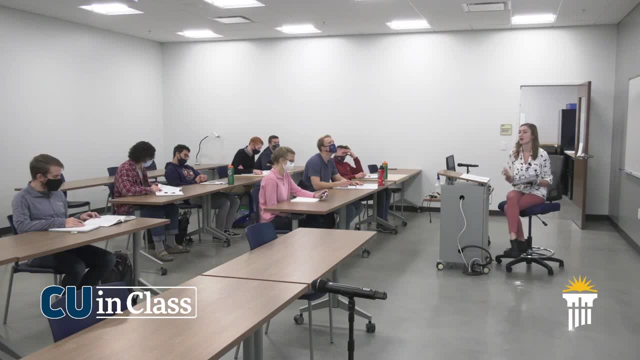 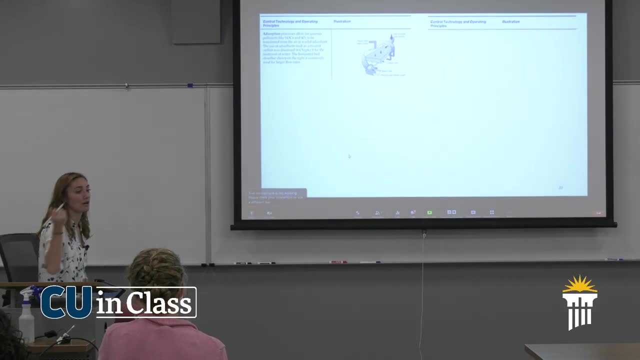 Speaker: 57 Speaker 58 Speaker, 51 Speaker, 52 Speaker, 53 Speaker, 54 Speaker, 56 Speaker, 57 Speaker. 58 Speaker 51 Speaker, 52 Speaker, 53 Speaker, 53 Speaker, 54 Speaker, 56 Speaker, 57 Speaker 58. 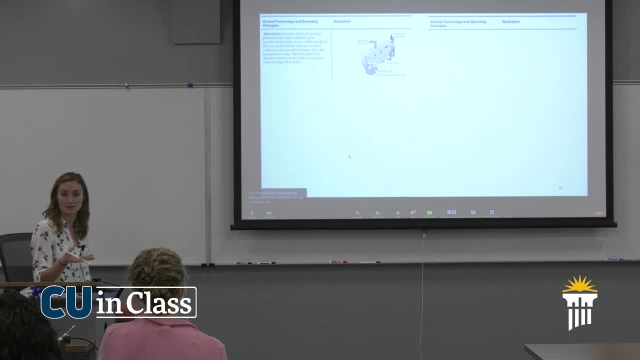 Speaker: 58 Speaker 59 Speaker, 51 Speaker, 52 Speaker, 53 Speaker, 53 Speaker, 54 Speaker, 53 Speaker, 54 Speaker, 55 Speaker, 56 Speaker, 56 Speaker, 57 Speaker, 56 Speaker, 57 Speaker, 58 Speaker 58. 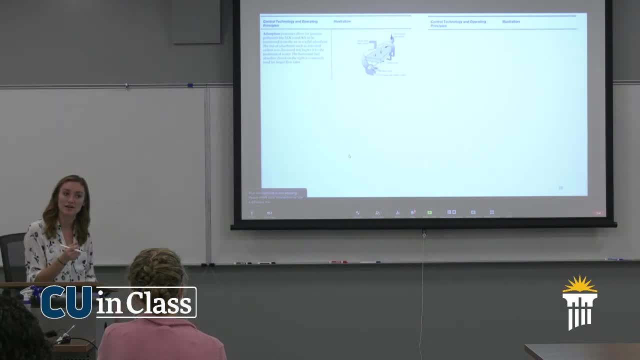 Speaker: 51 Speaker 52 Speaker, 53 Speaker, 53 Speaker, 53 Speaker, 54 Speaker, 54 Speaker, 56 Speaker, 56 Speaker, 57 Speaker, 58 Speaker 58 Speaker 58 Speaker 59 Speaker 51 Speaker, 52 Speaker 53. 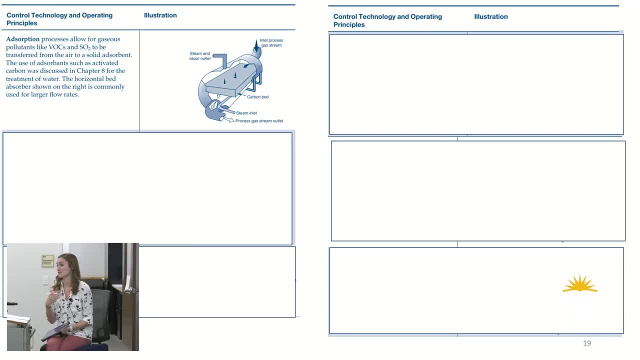 Speaker 53 Speaker 53 Speaker 54 Speaker 53 Speaker 54 Speaker, 55 Speaker, 56 Speaker, 56 Speaker, 56 Speaker 57 Speaker 57 Speaker 58 Speaker 58 Speaker 58 Speaker 59 Speaker, 51 Speaker 52. 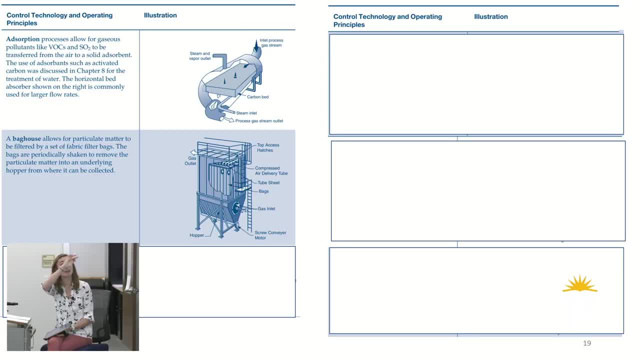 Speaker 53 Speaker 53 Speaker 53 Speaker 54 Speaker 53 Speaker 54 Speaker, 55 Speaker, 56 Speaker. 56 Speaker 56 Speaker 57 Speaker 58 Speaker 58 Speaker 58 Speaker 59 Speaker, 51 Speaker 52. 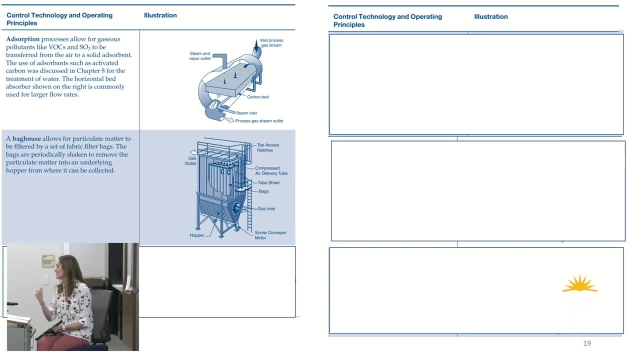 Speaker: 53 Speaker 53 Speaker 53 Speaker. 54 Speaker 53 Speaker 53 Speaker. 54 Speaker 53 Speaker 54 Speaker 55 Speaker 56 Speaker 56 Speaker 56 Speaker 57 Speaker 57 Speaker 58 Speaker 58. 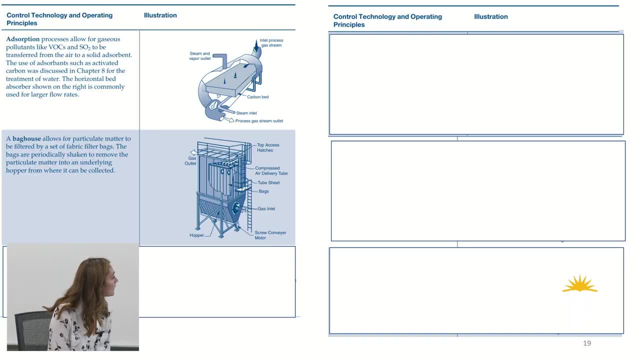 Speaker: 58 Speaker, 59 Speaker, 60 Speaker, 61 Speaker, 62 Speaker, 63 Speaker, 64 Speaker, 65 Speaker, 67 Speaker, 68 Speaker, 68 Speaker, 69 Speaker, 70 Speaker, 71 Speaker, 72 Speaker, 73 Speaker 74. 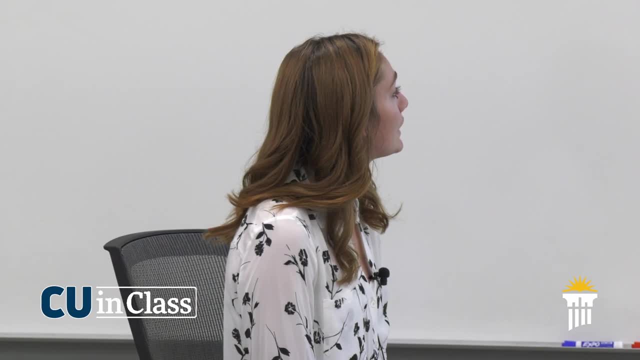 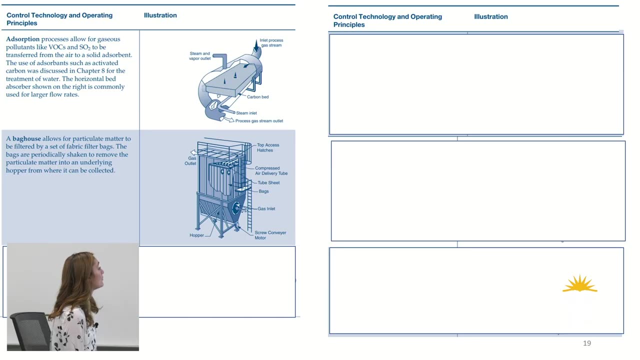 Speaker 75 Speaker 76 Speaker 76 Speaker 77 Speaker 78 Speaker 78 Speaker 79 Speaker 79 Speaker 90 Speaker 92 Speaker 93 Speaker 93 Speaker 94 Speaker 94 Speaker 95 Speaker 96 Speaker 96. 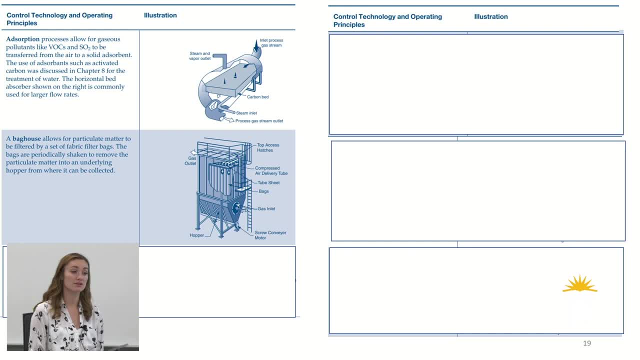 Speaker 97 Speaker 98 Speaker, 99 Speaker, 100 Speaker, 100 Speaker, 11 Speaker, 11 Speaker, 12 Speaker, 13 Speaker, 14 Speaker, 15 Speaker, 16 Speaker, 17 Speaker, 18 Speaker, 19 Speaker, 21 Speaker 22. 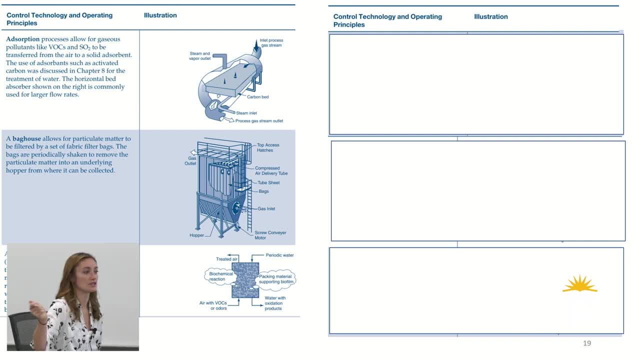 Speaker 23 Speaker 24 Speaker 25 Speaker, 26 Speaker, 27 Speaker, 27 Speaker, 28 Speaker, 29 Speaker, 30 Speaker, 31 Speaker, 32 Speaker, 33 Speaker, 34 Speaker, 35 Speaker, 36 Speaker, 37 Speaker 38. 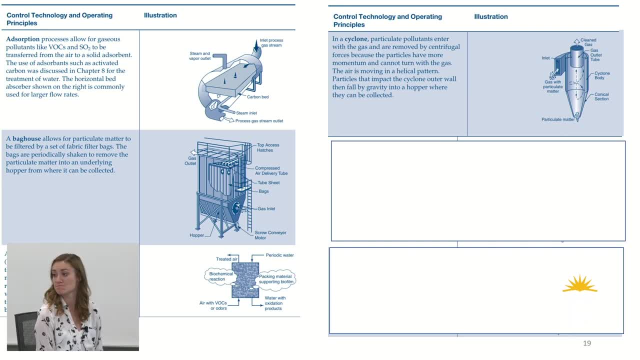 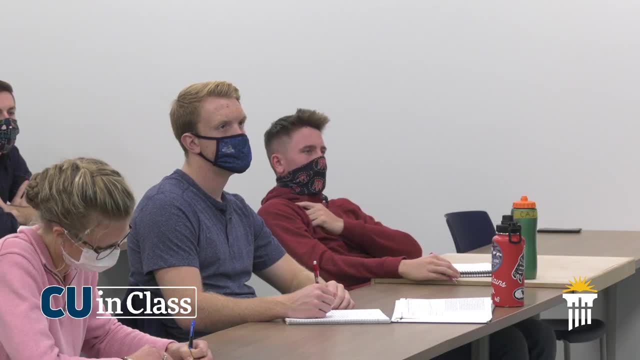 Speaker: 39 Speaker, 40 Speaker, 41 Speaker, 42 Speaker, 43 Speaker, 44 Speaker, 45 Speaker, 45 Speaker, 46 Speaker, 47 Speaker, 48 Speaker, 49 Speaker, 50 Speaker, 51 Speaker, 52 Speaker, 53 Speaker 53. 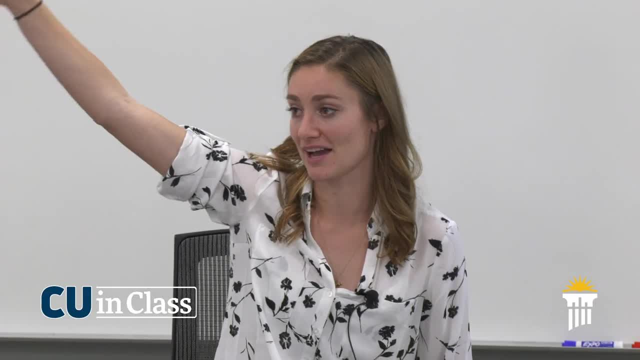 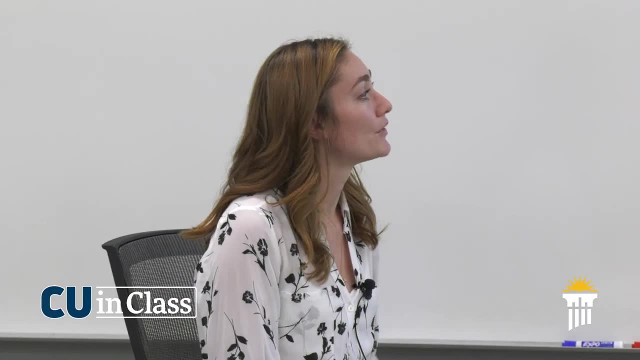 Speaker: 54 Speaker 56 Speaker, 57 Speaker, 57 Speaker, 58 Speaker, 58 Speaker, 59 Speaker, 51 Speaker. 52 Speaker 53 Speaker 54 Speaker, 55 Speaker, 56 Speaker, 57 Speaker, 58 Speaker, 58 Speaker 49. 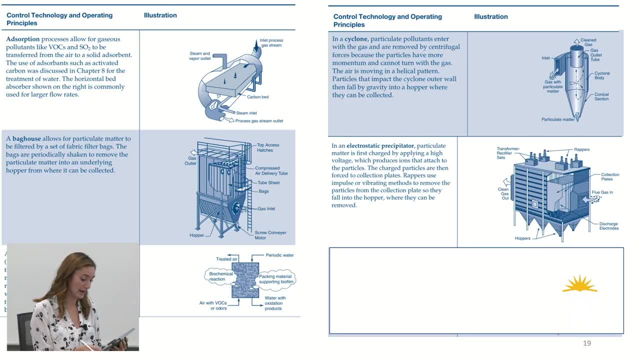 Speaker: 50 Speaker, 51 Speaker, 52 Speaker, 53 Speaker, 53 Speaker, 54 Speaker, 54 Speaker, 55 Speaker, 56 Speaker, 56 Speaker, 57 Speaker, 56 Speaker, 57 Speaker, 58 Speaker, 58 Speaker, 51 Speaker 52. 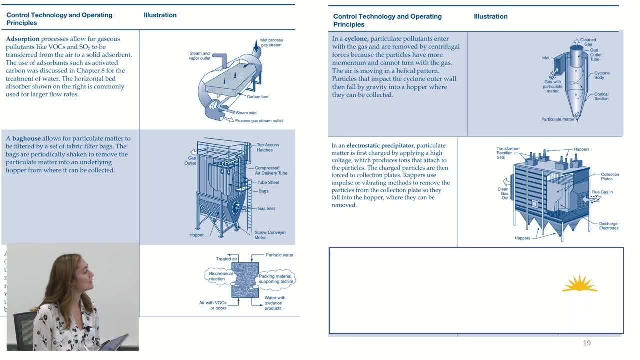 Speaker: 53 Speaker, 54 Speaker, 55 Speaker, 56 Speaker, 56 Speaker, 57 Speaker, 58 Speaker, 58 Speaker, 59 Speaker, 51 Speaker, 52 Speaker, 53 Speaker, 53 Speaker. 54 Speaker 53 Speaker, 54 Speaker 55. 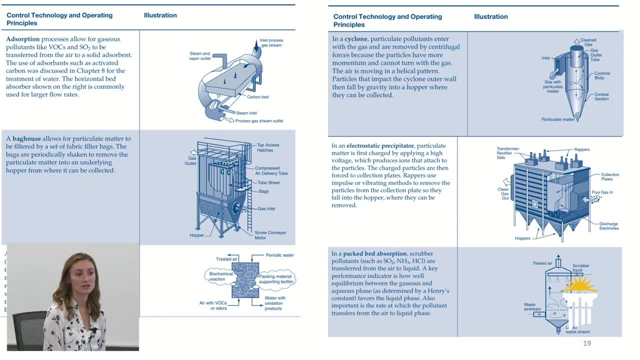 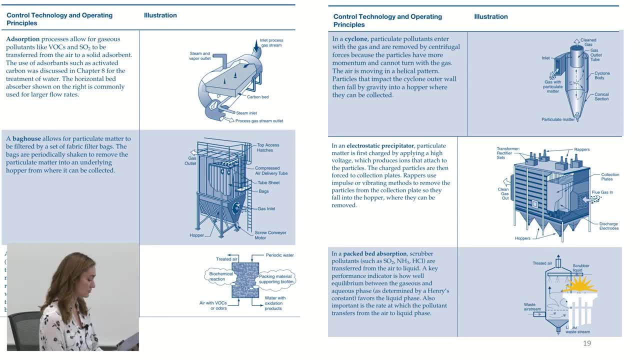 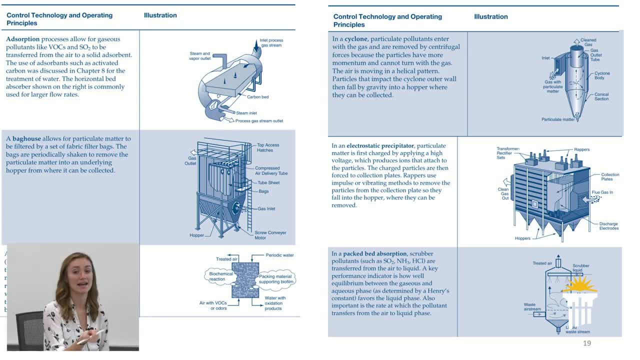 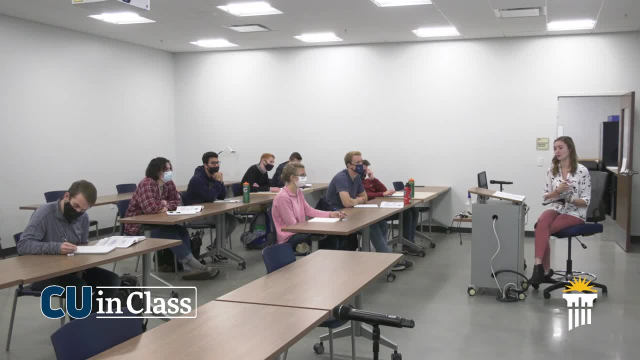 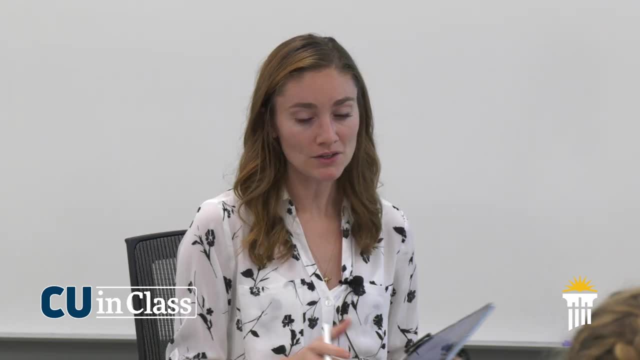 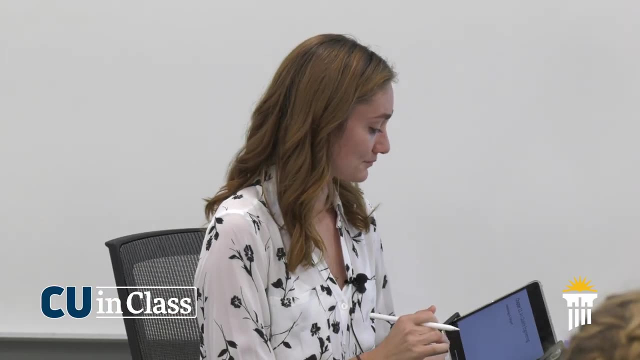 Speaker: 57 Speaker, 58 Speaker, 58 Speaker, 58 Speaker, 59 Speaker, 60 Speaker, 61 Speaker, 62 Speaker, 63 Speaker, 64 Speaker, 65 Speaker, 67 Speaker, 68 Speaker, 68 Speaker, 69 Speaker, 69 Speaker 70. 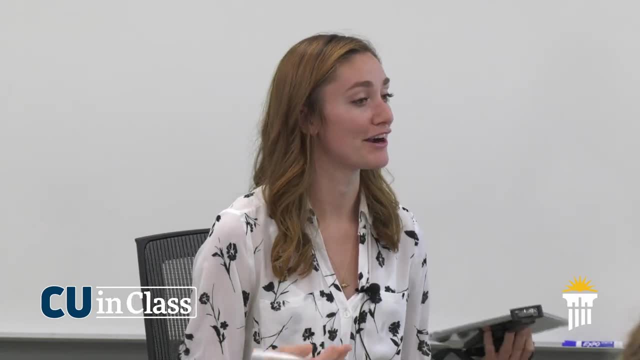 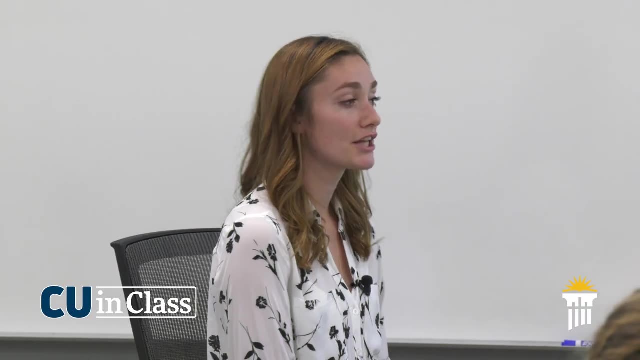 Speaker 71 Speaker, 72 Speaker, 73 Speaker, 74 Speaker, 75 Speaker, 76 Speaker, 76 Speaker, 77 Speaker, 78 Speaker, 79 Speaker, 79 Speaker, 80 Speaker, 92 Speaker, 93 Speaker, 93 Speaker, 94 Speaker 94. 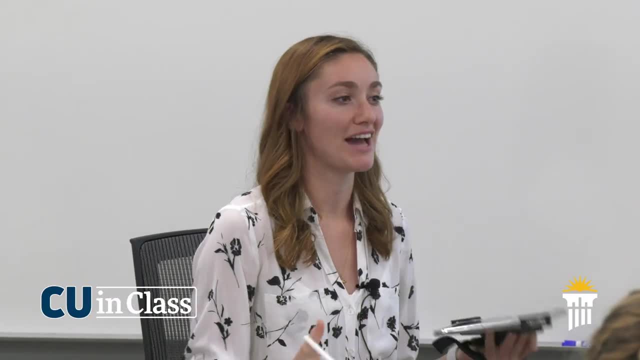 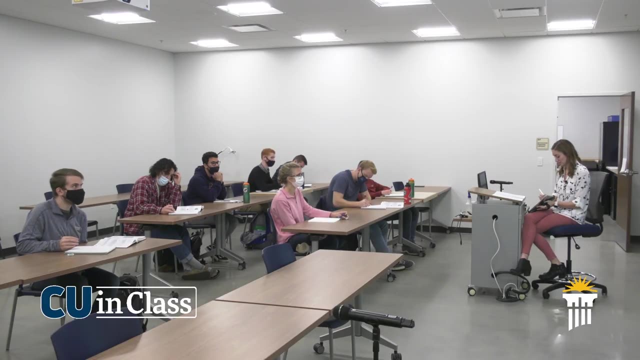 Speaker 95 Speaker 96 Speaker 96 Speaker 97 Speaker 98 Speaker 99 Speaker 100 Speaker 100 Speaker 11 Speaker 11 Speaker 12 Speaker 13 Speaker 14 Speaker 15 Speaker 16 Speaker 17 Speaker 18. 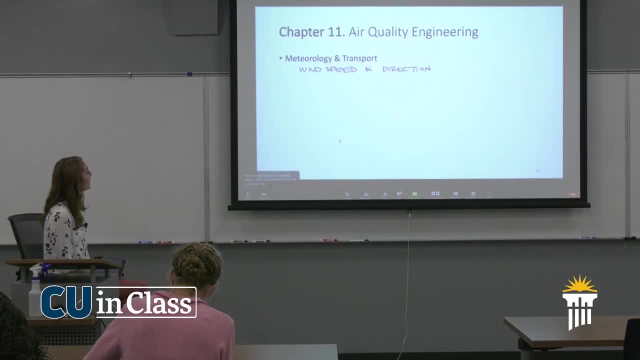 Speaker: 19 Speaker 21 Speaker 22 Speaker 23 Speaker 24 Speaker, 25 Speaker, 26 Speaker, 27 Speaker, 27 Speaker, 28 Speaker, 29 Speaker, 30 Speaker, 31 Speaker, 32 Speaker, 33 Speaker, 34 Speaker 35. 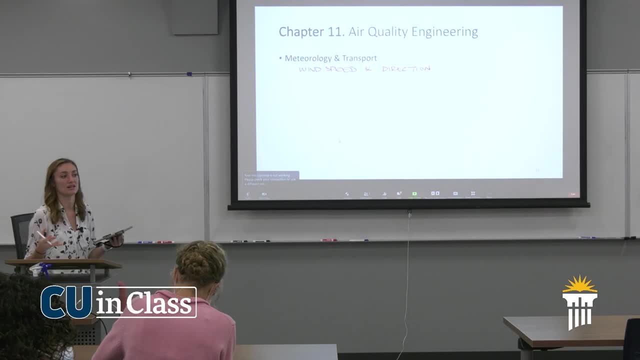 Speaker: 36 Speaker, 37 Speaker, 38 Speaker, 39 Speaker, 40 Speaker, 41 Speaker, 42 Speaker, 43 Speaker, 44 Speaker, 45 Speaker, 45 Speaker, 46 Speaker, 47 Speaker, 48 Speaker, 49 Speaker, 50 Speaker 51. 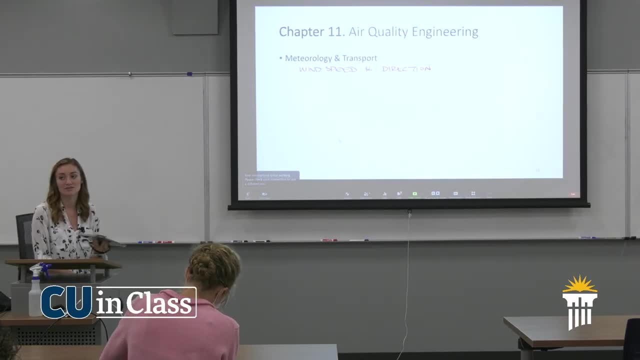 Speaker: 52 Speaker, 53 Speaker, 54 Speaker, 55 Speaker, 56 Speaker, 56 Speaker, 57 Speaker, 58 Speaker, 58 Speaker. 51 Speaker. 52 Speaker, 53 Speaker, 54 Speaker, 55 Speaker, 56 Speaker, 56 Speaker 57. 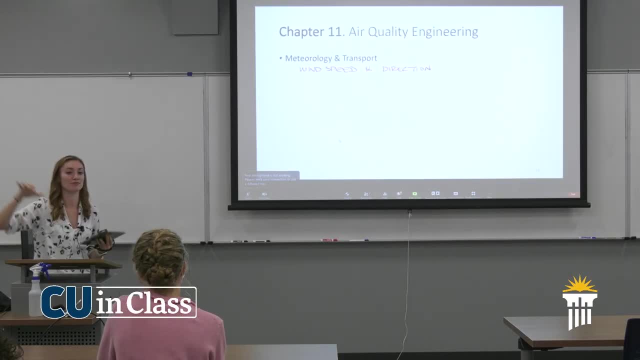 Speaker: 58 Speaker 51 Speaker, 52 Speaker, 53 Speaker, 53 Speaker, 54 Speaker, 55 Speaker, 56 Speaker. 56 Speaker 56 Speaker 57 Speaker 58 Speaker 58 Speaker 51 Speaker 52 Speaker, 53 Speaker 53. 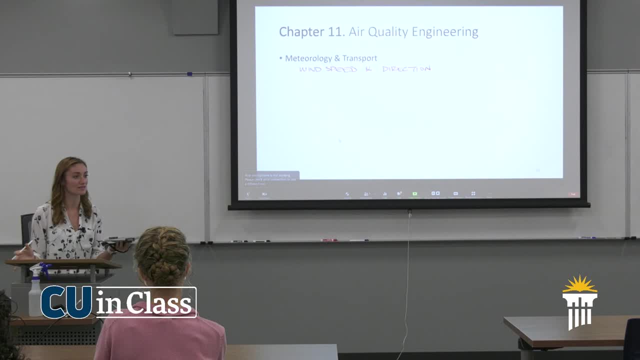 Speaker: 54 Speaker, 54 Speaker, 56 Speaker, 56 Speaker, 57 Speaker, 58 Speaker, 58 Speaker, 59 Speaker, 51 Speaker, 52 Speaker, 53 Speaker, 53 Speaker, 53 Speaker, 54 Speaker, 54 Speaker, 55 Speaker 56. 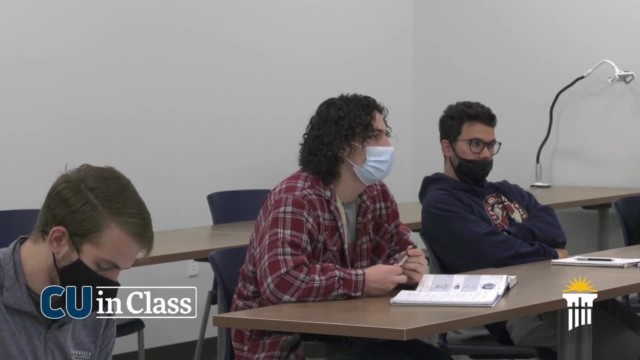 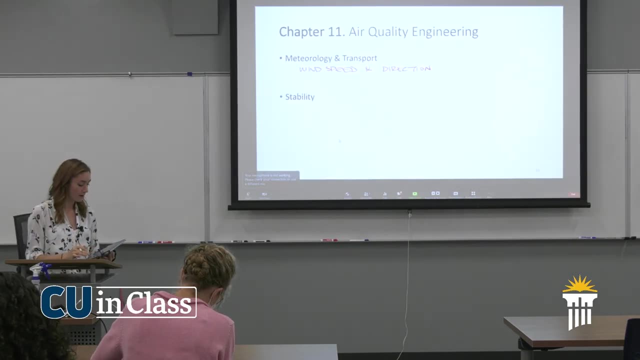 Speaker 56 Speaker 57 Speaker, 58 Speaker, 58 Speaker, 59 Speaker, 51 Speaker, 52 Speaker, 53 Speaker. 53 Speaker. 53 Speaker. 54 Speaker, 55 Speaker, 56 Speaker, 56 Speaker, 57 Speaker, 58 Speaker 58. 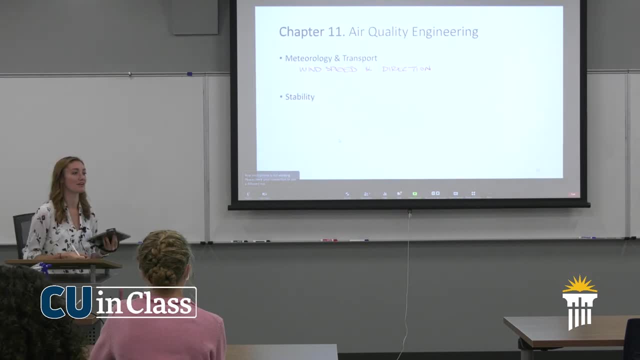 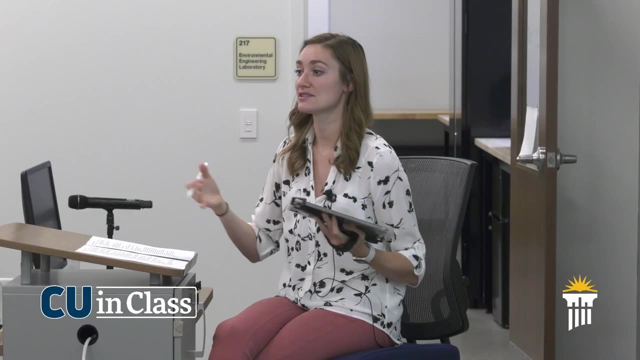 Speaker: 58 Speaker 59 Speaker, 50 Speaker, 51 Speaker, 52 Speaker, 53 Speaker, 53 Speaker, 54 Speaker, 53 Speaker, 54 Speaker, 55 Speaker, 56 Speaker, 56 Speaker, 56 Speaker, 57 Speaker, 57 Speaker 58. 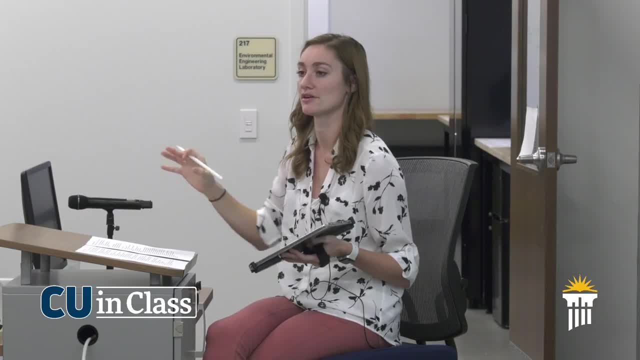 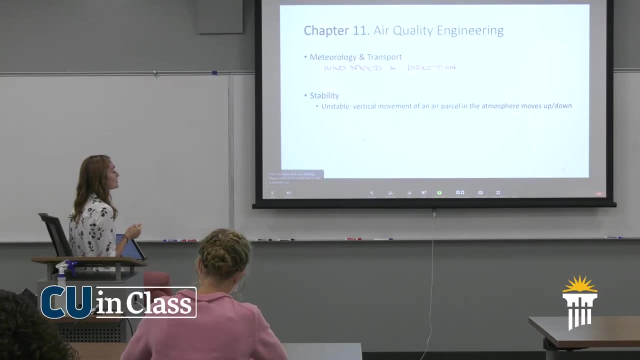 Speaker: 58 Speaker 58 Speaker, 59 Speaker, 51 Speaker, 52 Speaker, 53 Speaker, 53 Speaker, 53 Speaker, 54 Speaker, 54 Speaker, 56 Speaker, 56 Speaker, 57 Speaker, 58 Speaker, 58 Speaker, 58 Speaker 59. 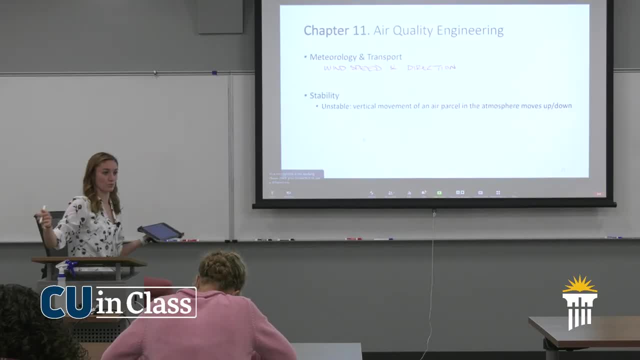 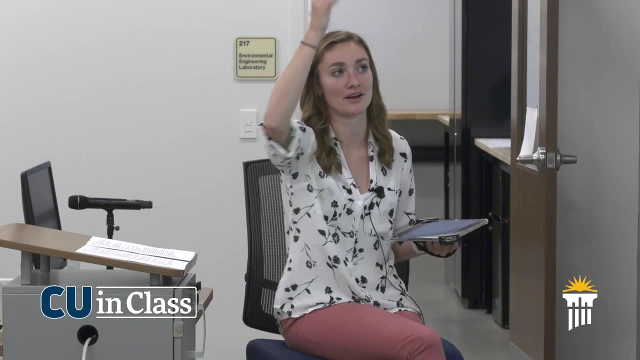 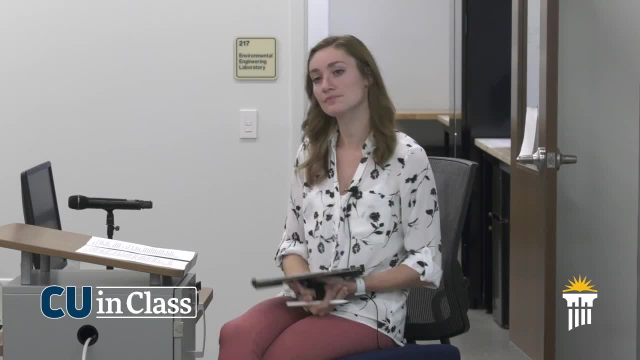 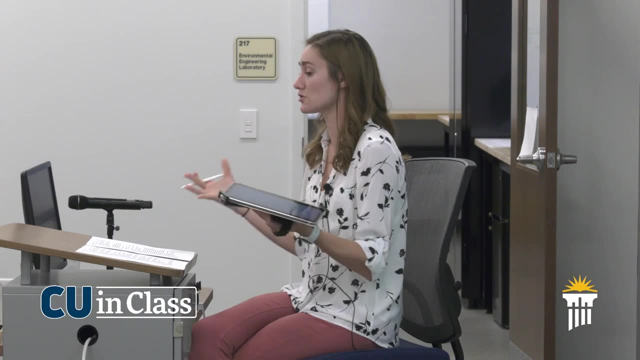 Speaker 59 Speaker 51 Speaker, 52 Speaker, 53 Speaker, 53 Speaker, 54 Speaker, 54 Speaker, 55 Speaker. 56 Speaker 56 Speaker 56 Speaker 57 Speaker 58 Speaker 58 Speaker 58 Speaker, 59 Speaker 51. 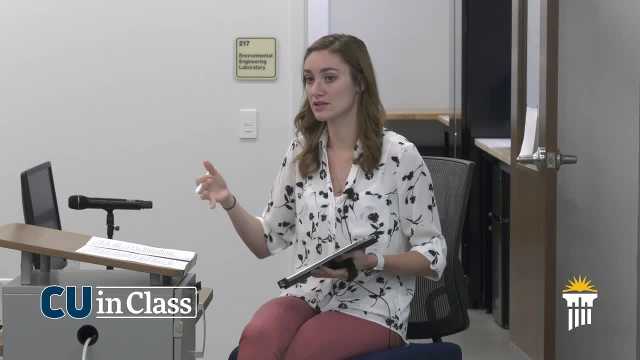 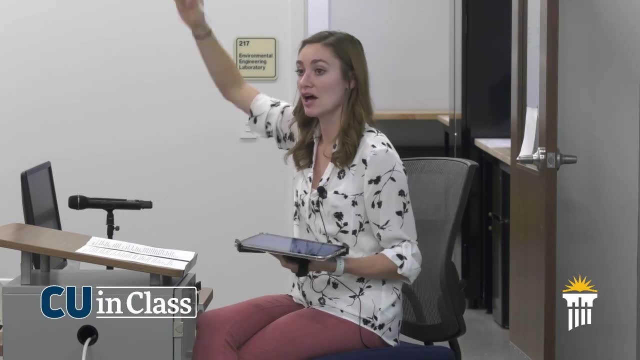 Speaker: 52 Speaker 53 Speaker, 53 Speaker, 54 Speaker, 54 Speaker, 55 Speaker, 56 Speaker, 56 Speaker, 56 Speaker 57 Speaker, 58 Speaker, 58 Speaker 58 Speaker 59 Speaker, 51 Speaker, 53 Speaker 54. 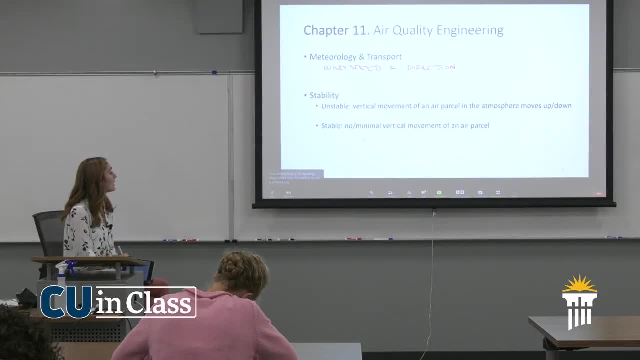 Speaker 56 Speaker 57 Speaker, 57 Speaker, 58 Speaker, 58 Speaker, 58 Speaker, 59 Speaker, 51 Speaker, 52 Speaker, 53 Speaker, 53 Speaker, 54 Speaker, 53 Speaker, 54 Speaker, 55 Speaker, 56 Speaker 56. 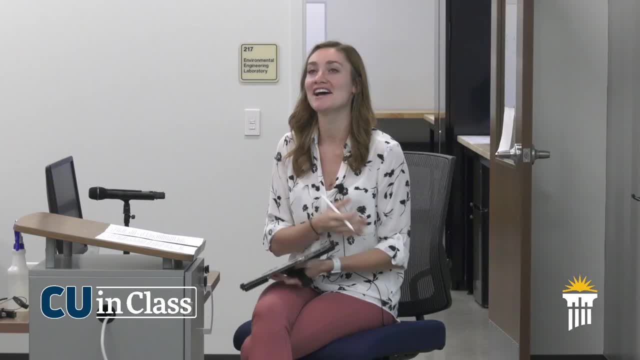 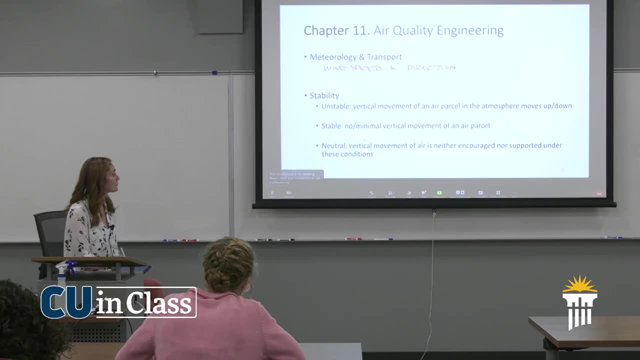 Speaker: 57 Speaker 56 Speaker, 57 Speaker, 58 Speaker, 58 Speaker, 59 Speaker, 51 Speaker, 52 Speaker, 53 Speaker, 53 Speaker, 54 Speaker, 54 Speaker, 55 Speaker, 56 Speaker, 56 Speaker, 57 Speaker 58. 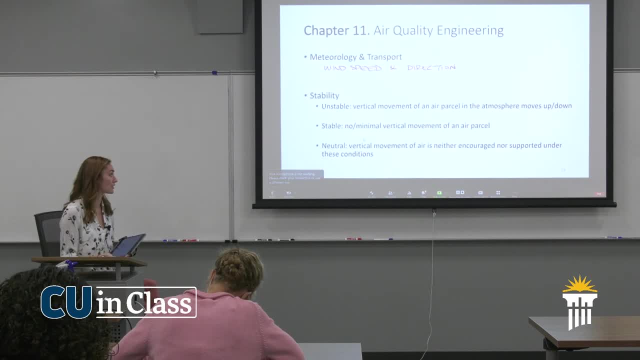 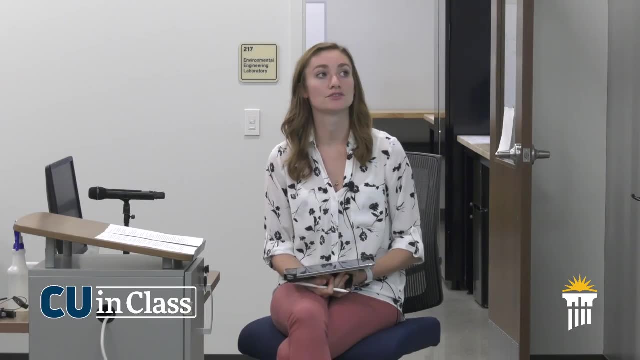 Speaker: 58 Speaker 58 Speaker, 59 Speaker, 51 Speaker, 52 Speaker, 53 Speaker, 53 Speaker, 54 Speaker, 53 Speaker, 54 Speaker, 55 Speaker, 56 Speaker, 56 Speaker, 56 Speaker, 57 Speaker, 57 Speaker 58. 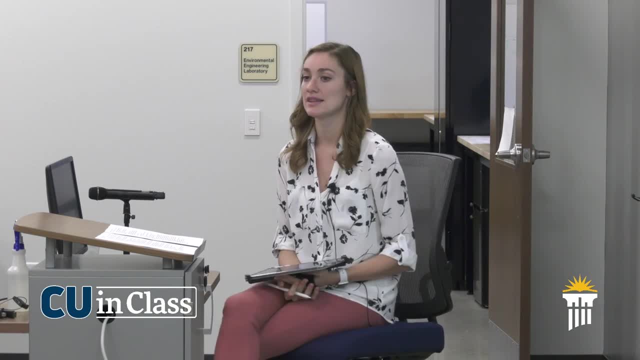 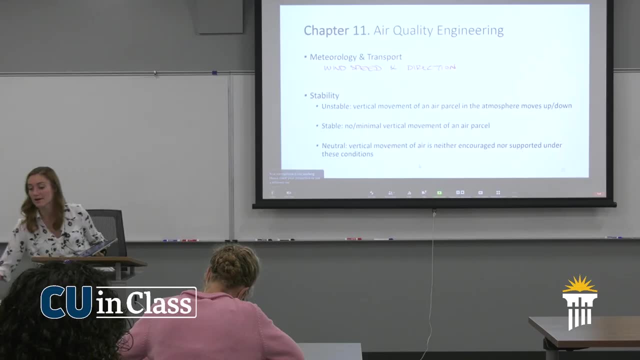 Speaker: 58 Speaker 59 Speaker, 51 Speaker, 52 Speaker, 53 Speaker, 53 Speaker, 53 Speaker, 54 Speaker, 54 Speaker, 55 Speaker, 56 Speaker, 56 Speaker, 57 Speaker, 58 Speaker, 58 Speaker, 59 Speaker 51. 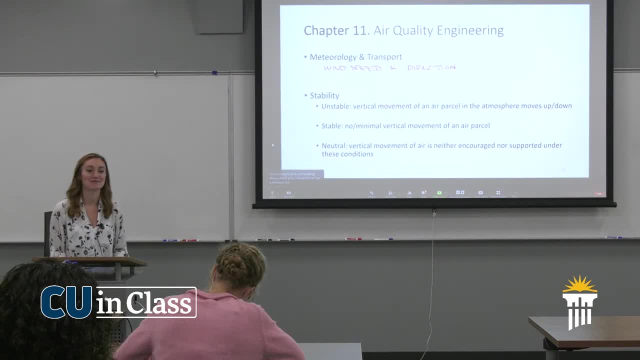 Speaker: 52 Speaker 53 Speaker, 53 Speaker. 54 Speaker. 53 Speaker, 53 Speaker, 54 Speaker, 54 Speaker, 55 Speaker, 56 Speaker, 56 Speaker 56 Speaker, 57 Speaker 58 Speaker 58 Speaker, 59 Speaker 51. 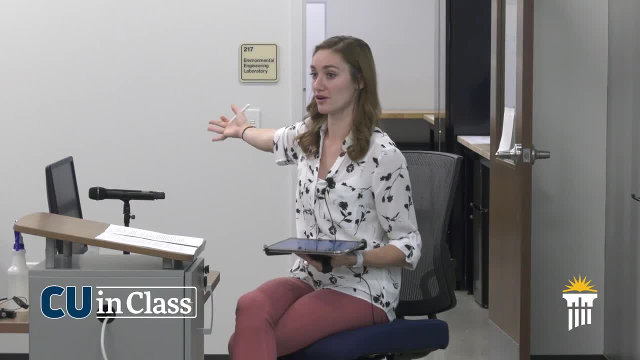 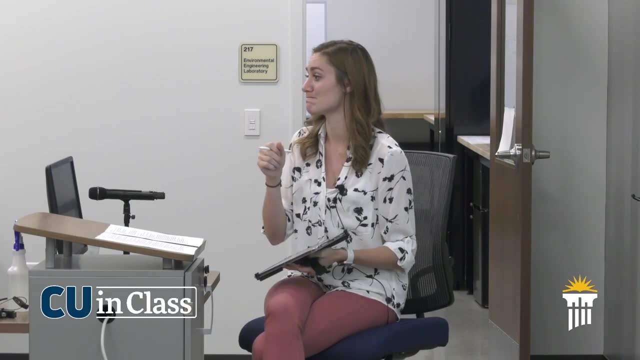 Speaker: 52 Speaker 53 Speaker. 53 Speaker. 53 Speaker 54 Speaker, 54 Speaker. 55 Speaker. 56 Speaker. 56 Speaker 56 Speaker 57 Speaker 58 Speaker 58 Speaker 59 Speaker 51 Speaker. 52 Speaker 53. 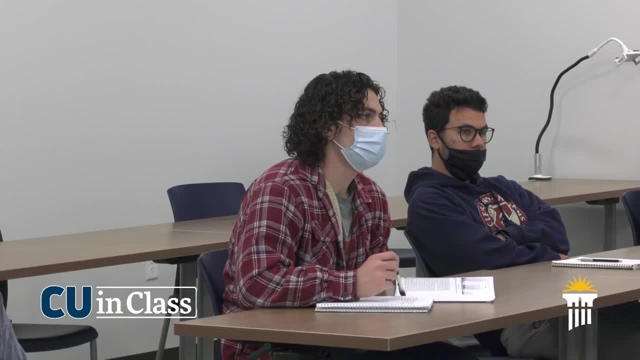 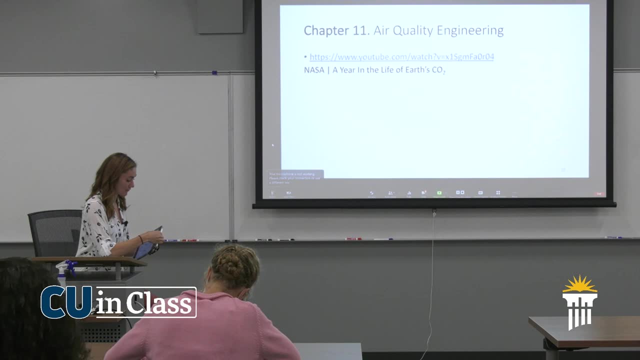 Speaker: 53 Speaker 53 Speaker, 54 Speaker, 54 Speaker, 55 Speaker, 56 Speaker, 56 Speaker, 56 Speaker, 57 Speaker, 58 Speaker, 58 Speaker, 59 Speaker, 51 Speaker, 52 Speaker 53 Speaker, 53 Speaker 53. 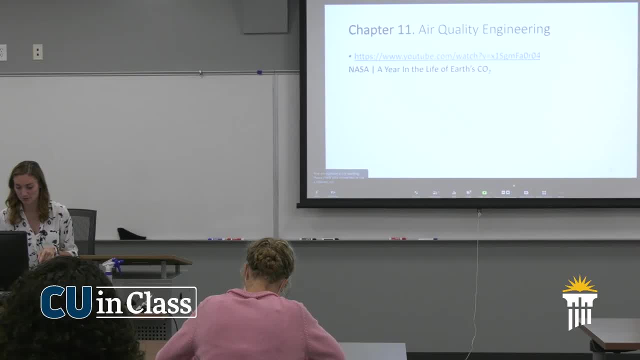 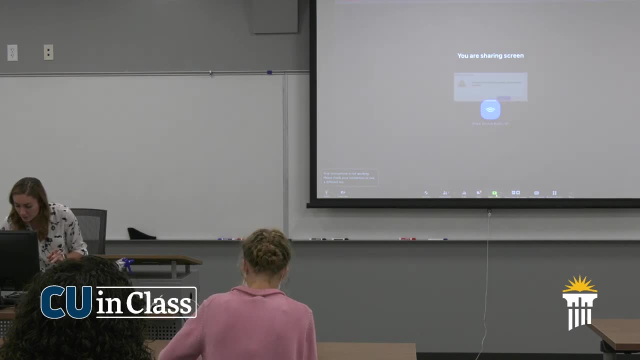 Speaker: 54 Speaker 54 Speaker, 55 Speaker, 56 Speaker, 56 Speaker, 56 Speaker, 57 Speaker, 58 Speaker, 58 Speaker, 59 Speaker, 51 Speaker, 52 Speaker, 53 Speaker, 53 Speaker, 54 Speaker, 53 Speaker 54. 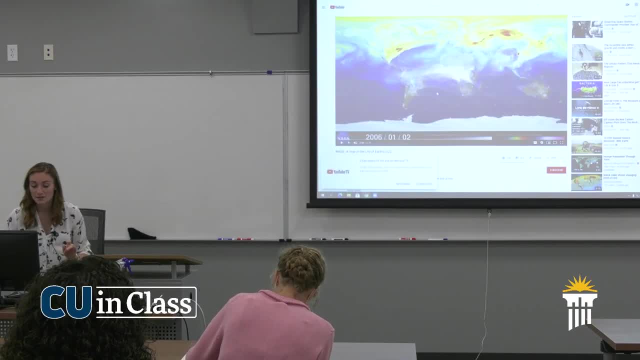 Speaker: 55 Speaker 56 Speaker, 56 Speaker, 56 Speaker, 57 Speaker, 58 Speaker, 58 Speaker, 58 Speaker, 59 Speaker 51 Speaker, 52 Speaker, 53 Speaker, 53 Speaker, 54 Speaker, 54 Speaker, 55 Speaker 56. 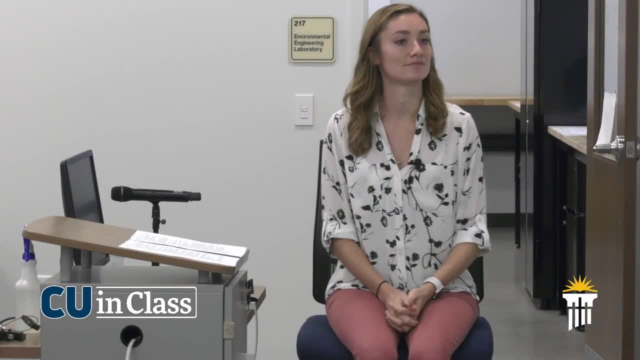 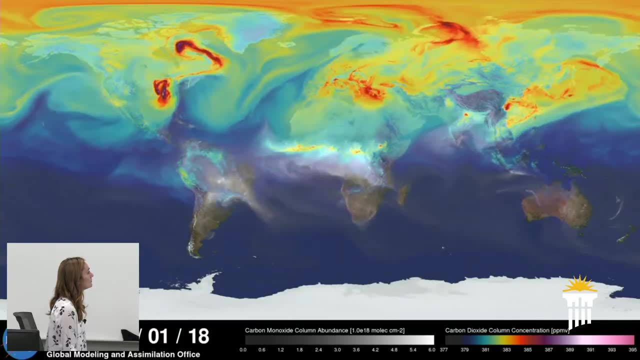 Speaker: 56 Speaker, 57 Speaker, 58 Speaker, 58 Speaker, 59 Speaker, 51 Speaker, 52 Speaker, 53 Speaker, 53 Speaker. 54 Speaker, 53 Speaker, 54 Speaker, 55 Speaker, 56 Speaker, 56 Speaker, 57 Speaker 58. 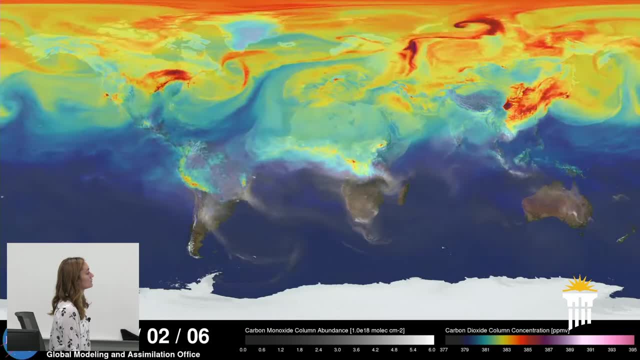 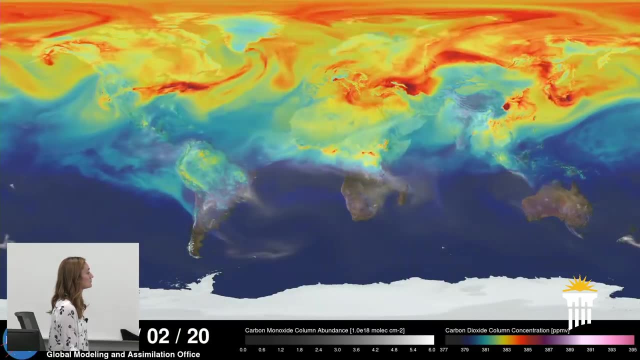 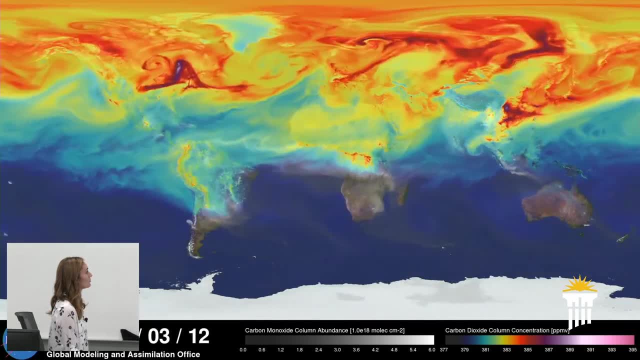 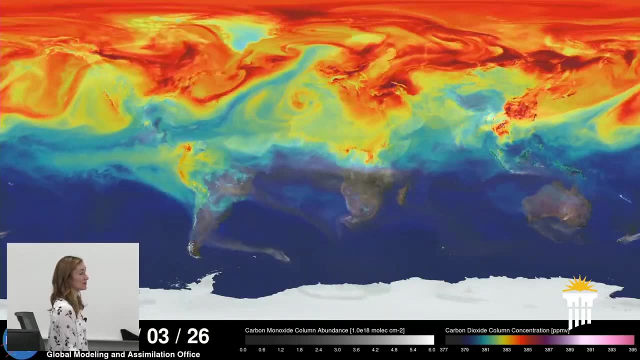 Speaker: 58 Speaker 58 Speaker, 59 Speaker, 51 Speaker, 52 Speaker, 53 Speaker, 53 Speaker, 54 Speaker, 53 Speaker 53 Speaker, 54 Speaker, 54 Speaker, 55 Speaker, 56 Speaker, 56 Speaker, 56 Speaker 57. 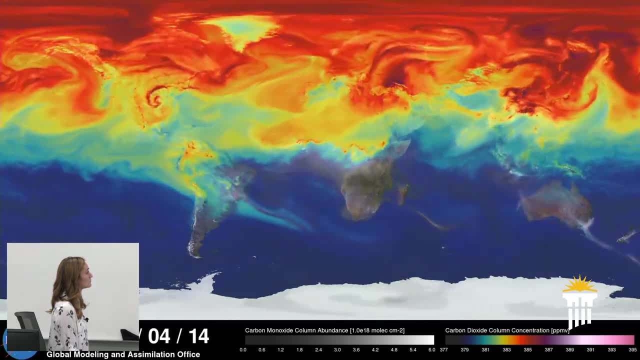 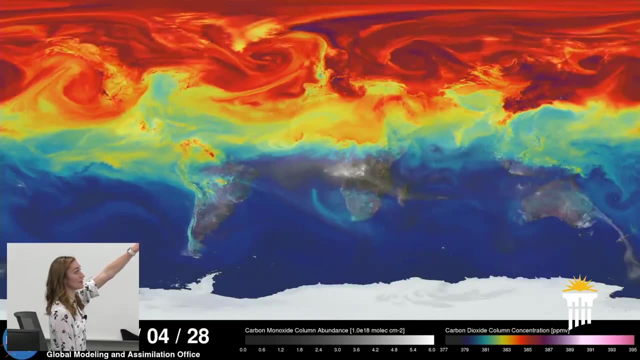 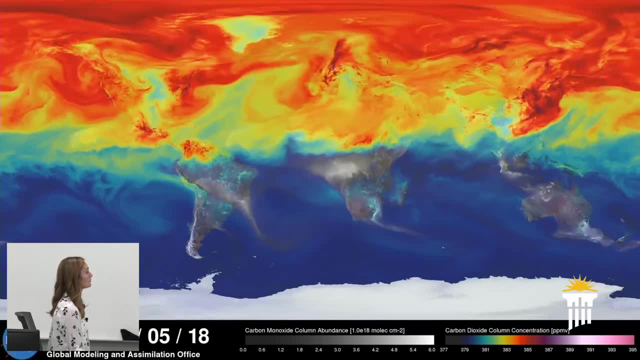 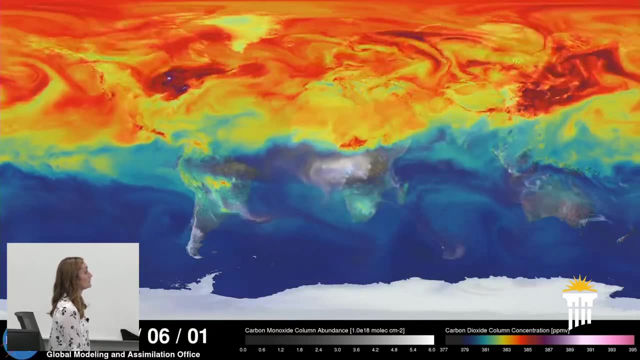 Speaker 71 Speaker 72 Speaker, 73 Speaker, 74 Speaker, 75 Speaker, 76 Speaker, 76 Speaker, 78 Speaker, 79 Speaker 79 Speaker, 80 Speaker, 92 Speaker, 93 Speaker, 93 Speaker 94 Speaker, 94 Speaker 95. 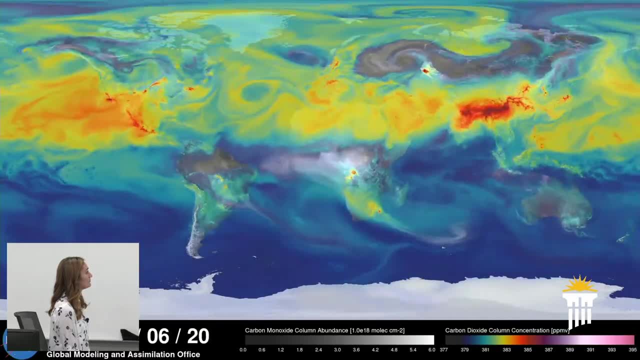 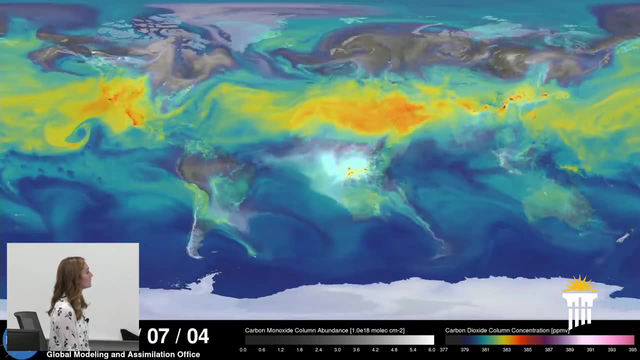 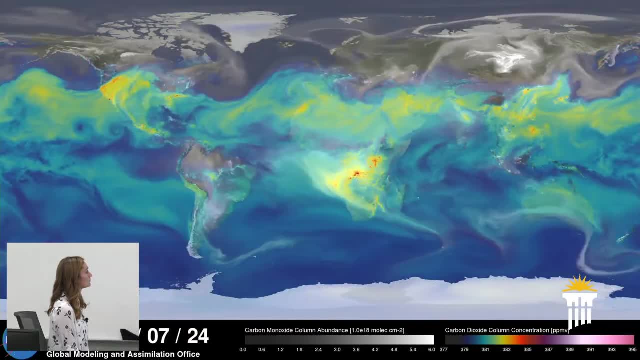 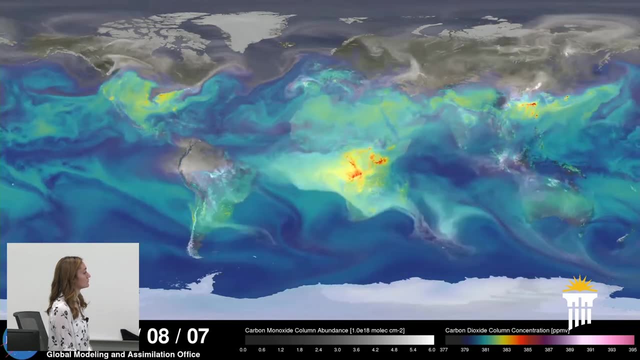 Speaker 21 Speaker 22 Speaker 23 Speaker 24 Speaker, 25 Speaker, 26 Speaker, 27 Speaker, 28 Speaker, 29 Speaker 31 Speaker 32 Speaker, 33 Speaker, 34 Speaker, 35 Speaker, 36 Speaker, 37 Speaker 38. 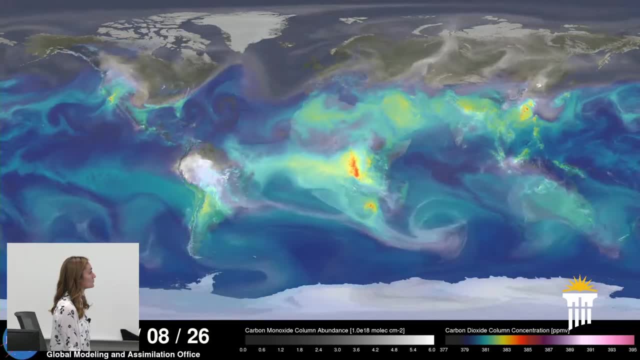 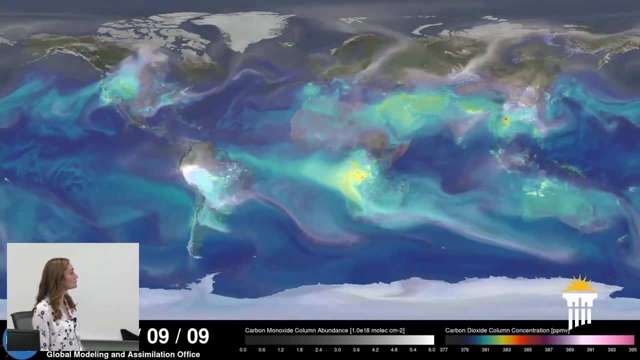 Speaker: 39 Speaker, 40 Speaker, 41 Speaker, 42 Speaker, 43 Speaker, 44 Speaker, 45 Speaker, 47 Speaker, 48 Speaker, 49 Speaker, 50 Speaker, 51 Speaker, 52 Speaker, 53 Speaker, 54 Speaker, 56 Speaker 56. 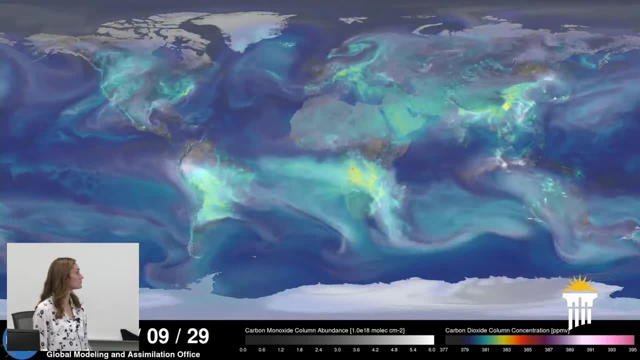 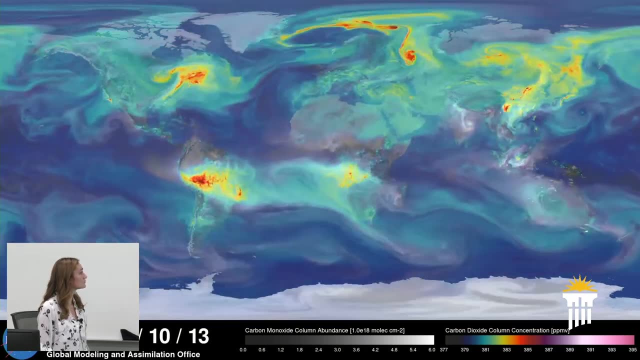 Speaker: 57 Speaker 58 Speaker, 51 Speaker, 52 Speaker, 53 Speaker, 53 Speaker. 54 Speaker. 56 Speaker. 56 Speaker. 57 Speaker. 58 Speaker. 58 Speaker, 59 Speaker. 51 Speaker, 52 Speaker, 53 Speaker 54. 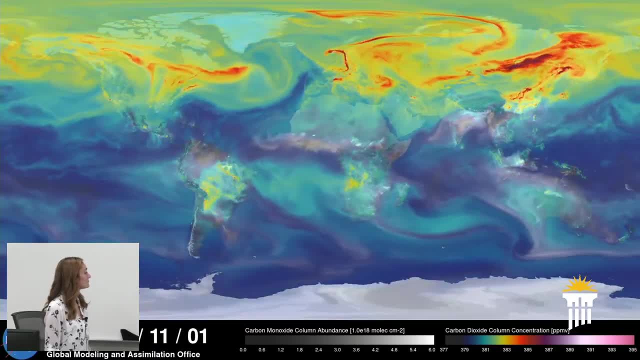 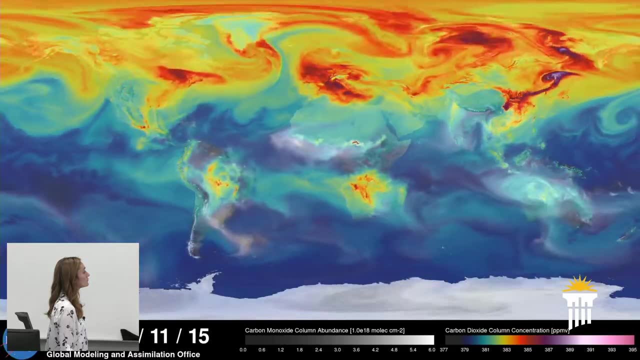 Speaker: 54 Speaker, 55 Speaker, 56 Speaker, 57 Speaker, 58 Speaker, 58 Speaker, 59 Speaker, 51 Speaker, 52 Speaker, 53 Speaker, 53 Speaker, 54 Speaker, 55 Speaker, 56 Speaker, 57 Speaker, 58 Speaker 58. 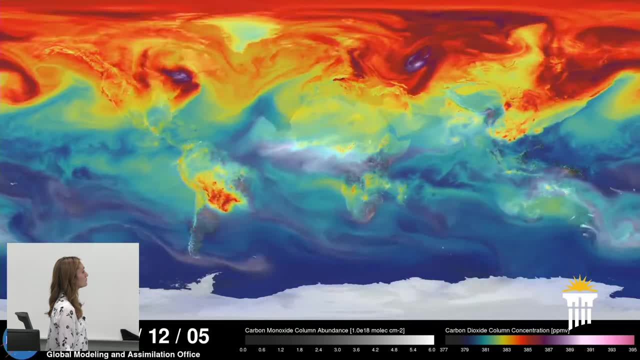 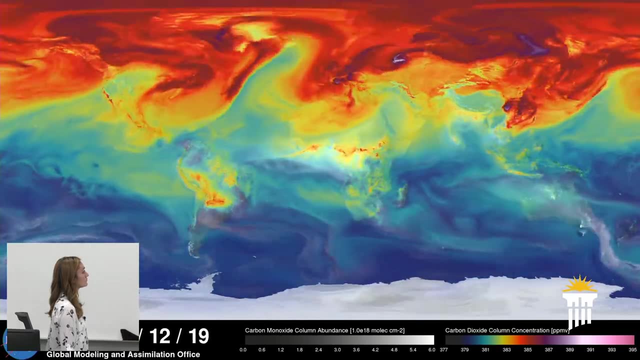 Speaker: 51 Speaker, 52 Speaker, 53 Speaker, 54 Speaker, 54 Speaker, 55 Speaker, 56 Speaker, 56 Speaker, 57 Speaker, 58 Speaker, 58 Speaker, 59 Speaker, 51 Speaker, 52 Speaker, 53 Speaker, 53 Speaker 54. 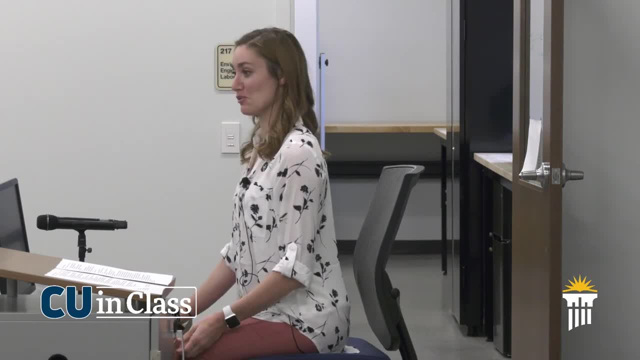 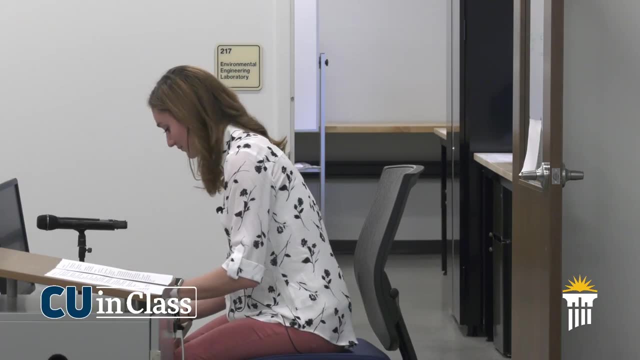 Speaker: 53 Speaker, 54 Speaker, 55 Speaker, 56 Speaker, 56 Speaker, 57 Speaker, 57 Speaker, 58 Speaker, 58 Speaker, 59 Speaker, 51 Speaker, 52 Speaker, 53 Speaker, 53 Speaker, 54 Speaker, 54 Speaker 55. 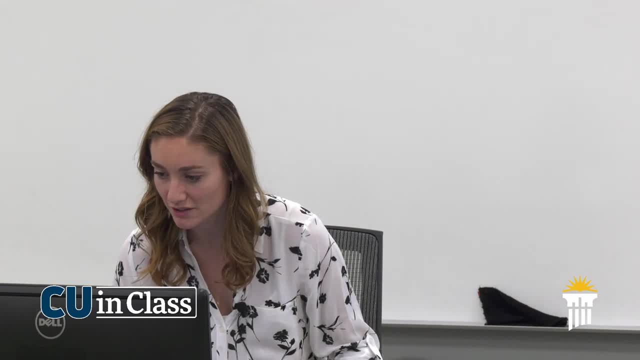 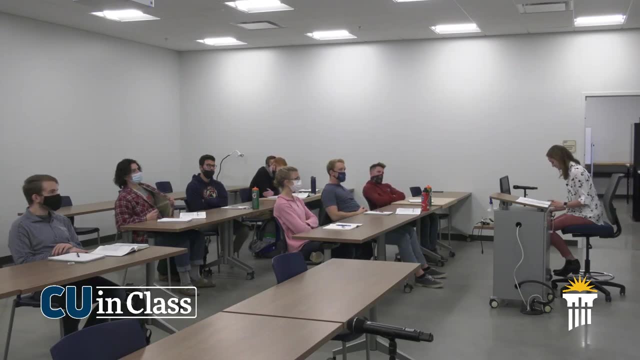 Speaker 56 Speaker 57 Speaker, 58 Speaker, 58 Speaker 58 Speaker, 59 Speaker, 51 Speaker, 52 Speaker, 53 Speaker 53 Speaker 54 Speaker 53 Speaker, 54 Speaker, 55 Speaker, 56 Speaker, 56 Speaker 57. 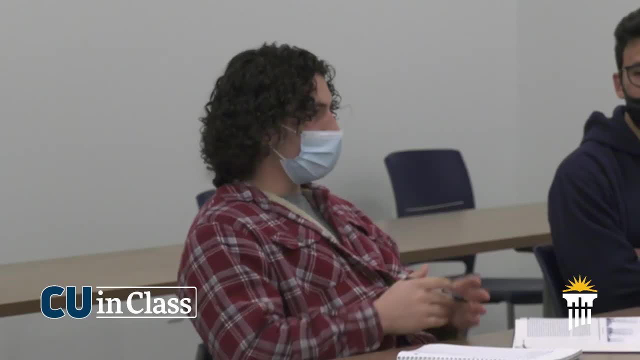 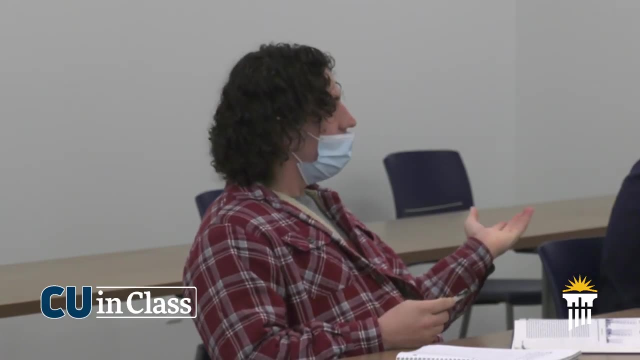 Speaker: 58 Speaker 58 Speaker 58 Speaker, 59 Speaker, 51 Speaker, 52 Speaker, 53 Speaker, 53 Speaker, 53 Speaker 54 Speaker 53 Speaker, 54 Speaker, 53 Speaker, 54 Speaker, 55 Speaker, 56 Speaker 56. 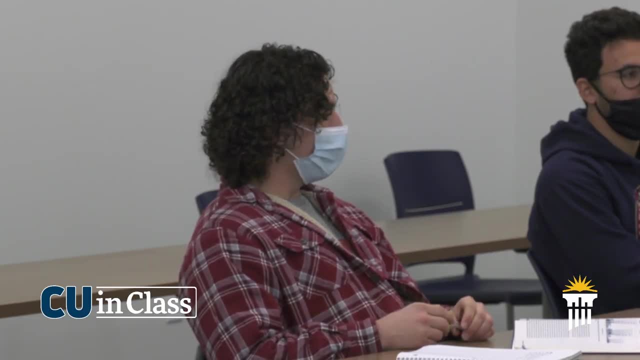 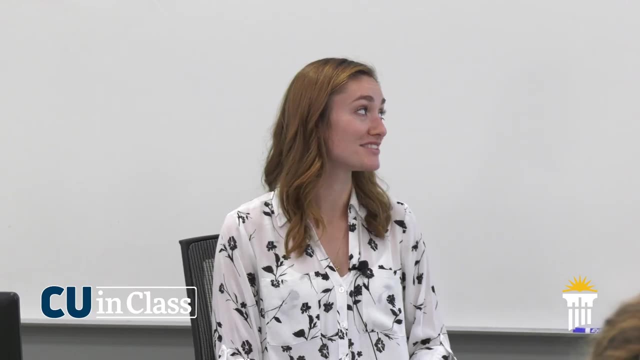 Speaker: 57 Speaker 58 Speaker, 58 Speaker, 59 Speaker, 51 Speaker, 52 Speaker, 53 Speaker, 53 Speaker. 53 Speaker. 54 Speaker, 53 Speaker, 54 Speaker, 55 Speaker, 56 Speaker, 56 Speaker, 56 Speaker 57. 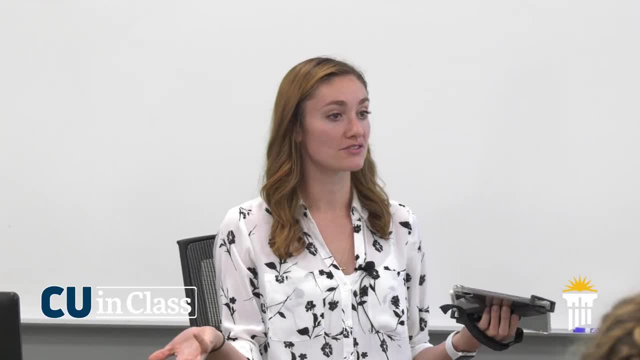 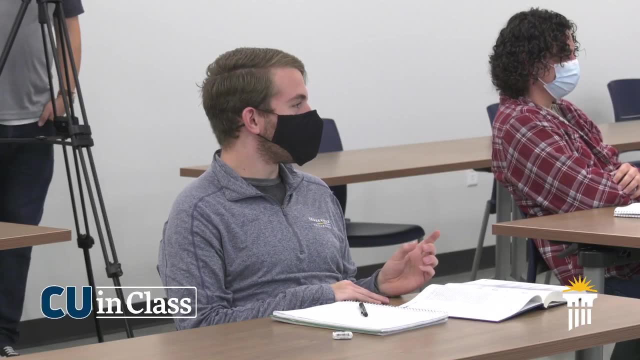 Speaker: 58 Speaker 58 Speaker 58 Speaker, 59 Speaker, 51 Speaker, 52 Speaker, 53 Speaker. 53 Speaker. 54 Speaker 55 Speaker 56 Speaker. 56 Speaker 56 Speaker 57 Speaker 58 Speaker, 58 Speaker 59. 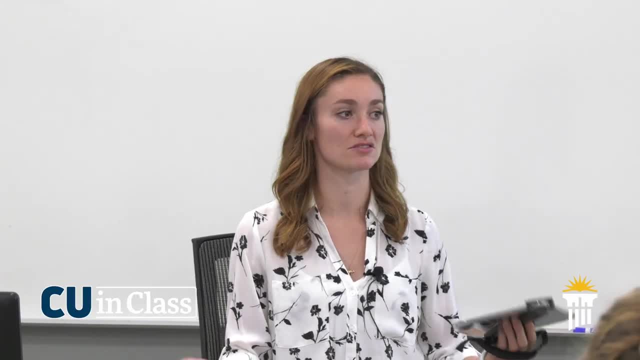 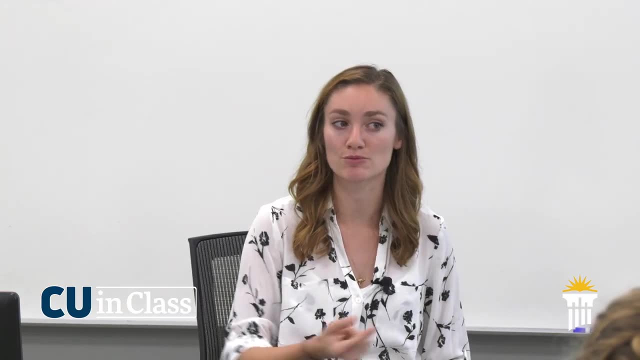 Speaker: 51 Speaker 52 Speaker, 53 Speaker, 53 Speaker, 53 Speaker, 54 Speaker, 54 Speaker, 55 Speaker, 56 Speaker. 56 Speaker, 56 Speaker, 57 Speaker, 58 Speaker, 58 Speaker, 59 Speaker, 51 Speaker 52. 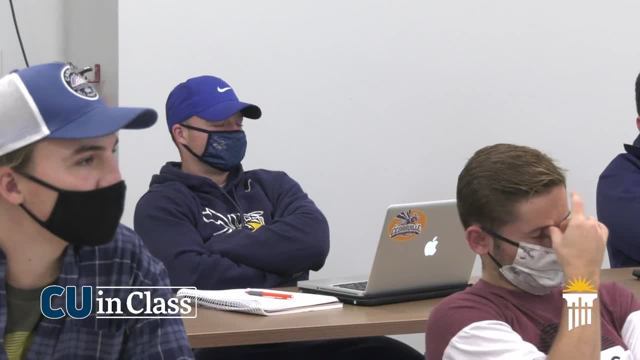 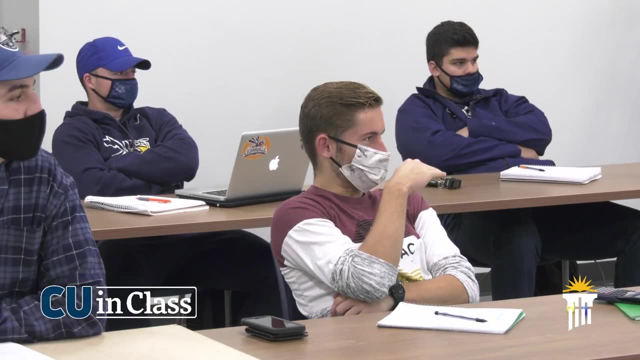 Speaker 53 Speaker 53 Speaker 53 Speaker, 54 Speaker, 54 Speaker, 55 Speaker, 55 Speaker, 56 Speaker, 56 Speaker 57 Speaker 58 Speaker 58 Speaker 58 Speaker 59 Speaker 51 Speaker, 52 Speaker 53. 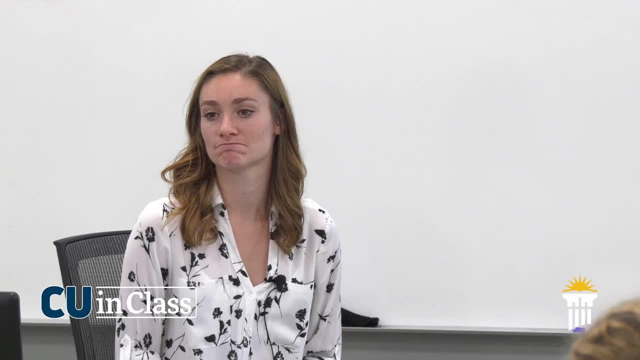 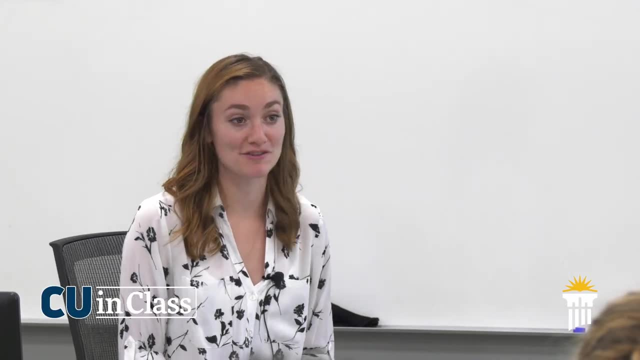 Speaker: 53 Speaker 54 Speaker. 53 Speaker, 54 Speaker, 55 Speaker, 56 Speaker, 56 Speaker, 57 Speaker, 58 Speaker, 58 Speaker, 58 Speaker, 59 Speaker, 51 Speaker, 52 Speaker, 53 Speaker, 53 Speaker 54. 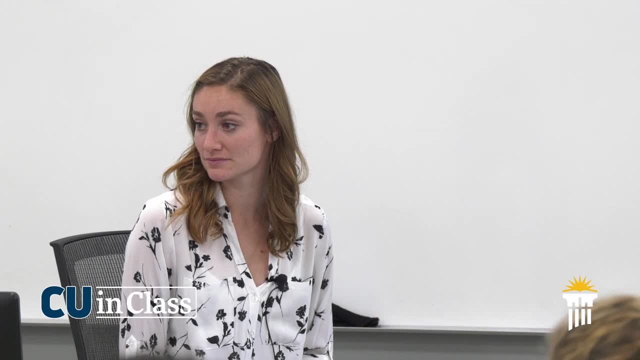 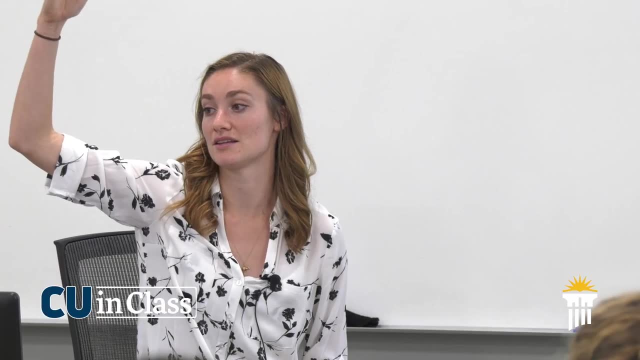 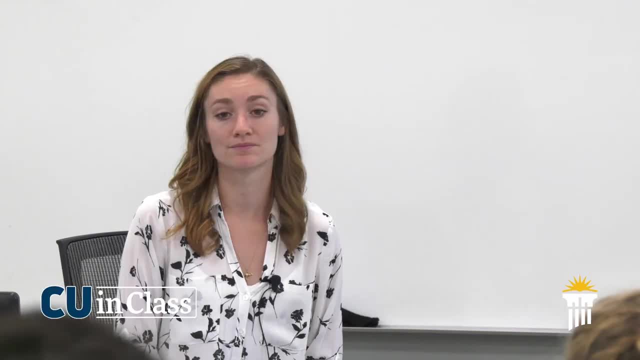 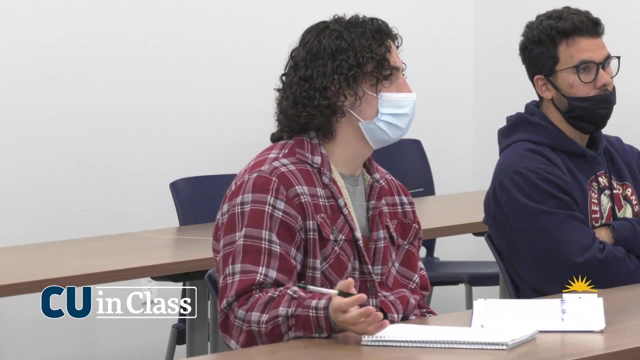 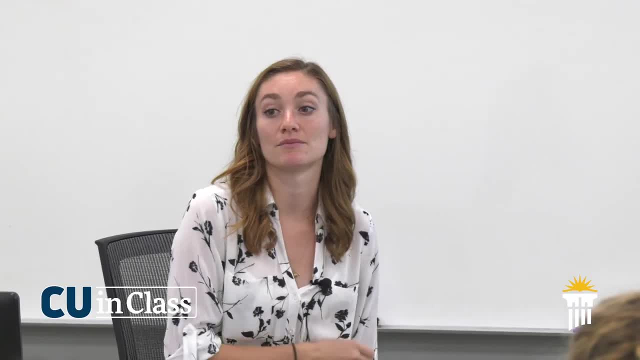 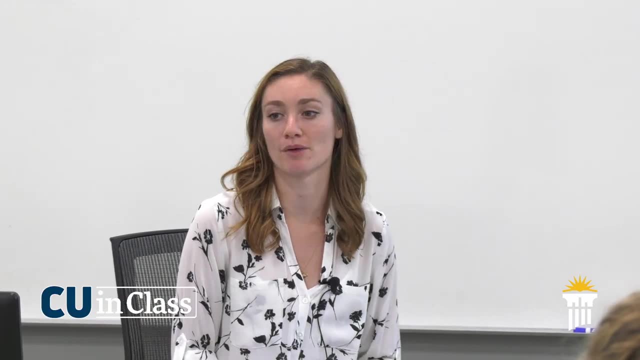 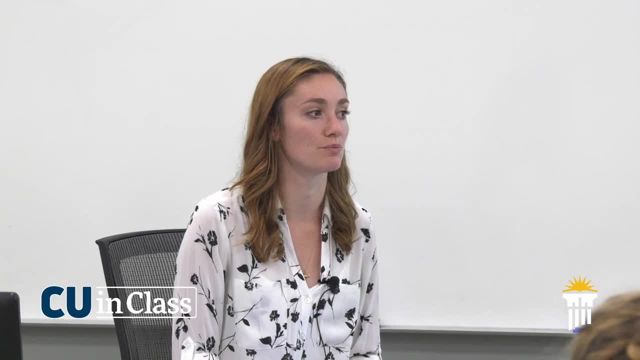 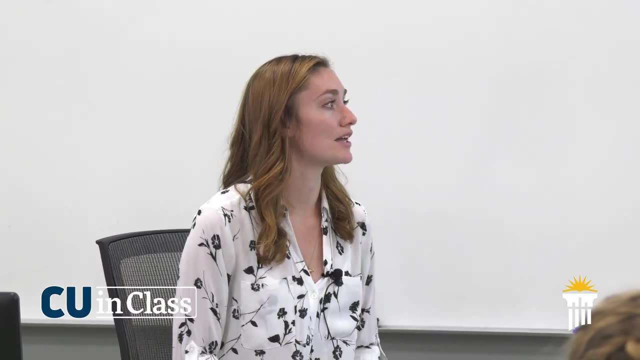 Speaker: 59 Speaker 51 Speaker, 52 Speaker, 53 Speaker, 53 Speaker, 54 Speaker, 53 Speaker, 54 Speaker, 55 Speaker, 56 Speaker, 56 Speaker, 56 Speaker, 57 Speaker, 58 Speaker, 58 Speaker, 59 Speaker 51. 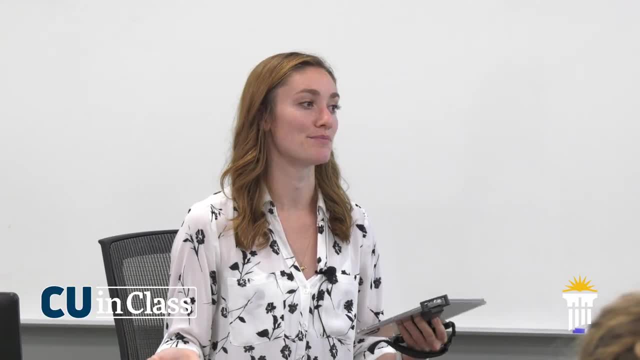 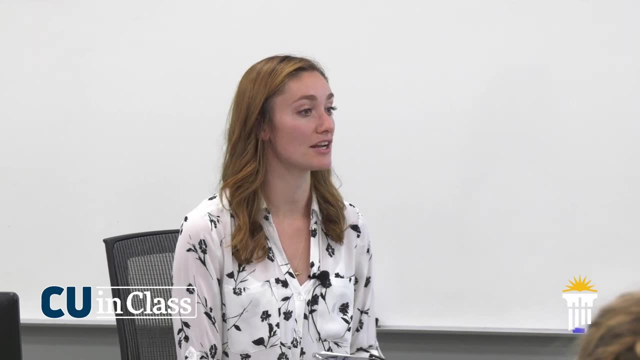 Speaker: 53 Speaker 53 Speaker. 54 Speaker. 53 Speaker, 54 Speaker, 54 Speaker, 56 Speaker, 56 Speaker, 57 Speaker, 58 Speaker, 58 Speaker, 59 Speaker, 51 Speaker, 52 Speaker, 53 Speaker, 53 Speaker 54. 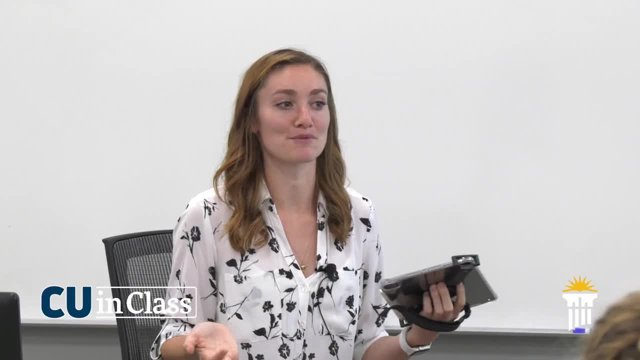 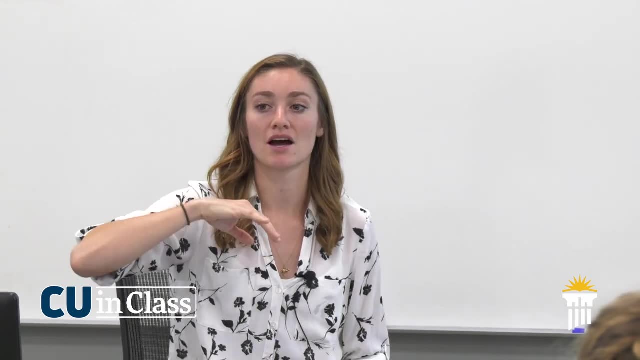 Speaker: 54 Speaker 53 Speaker 54 Speaker, 54 Speaker, 55 Speaker, 55 Speaker, 56 Speaker, 56 Speaker, 57 Speaker, 58 Speaker, 58 Speaker, 58 Speaker, 59 Speaker, 51 Speaker, 52 Speaker, 53 Speaker 53. 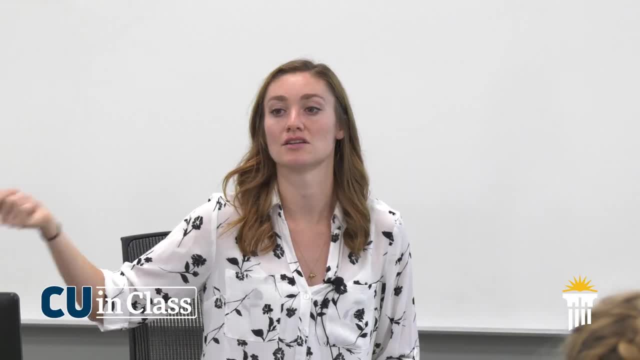 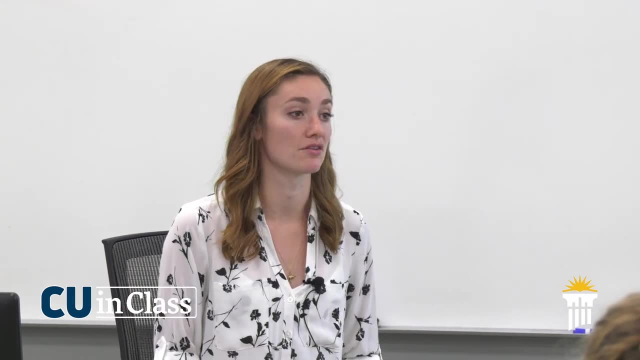 Speaker 53 Speaker 54 Speaker 53 Speaker 53 Speaker 54 Speaker 53 Speaker 54 Speaker 55 Speaker 56 Speaker 56 Speaker 56 Speaker 57 Speaker 58 Speaker 58 Speaker 58 Speaker 59 Speaker 51. 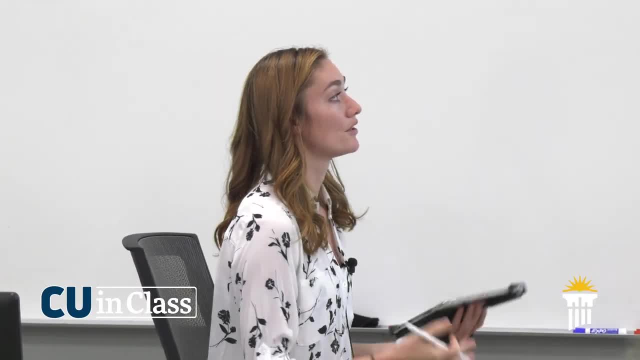 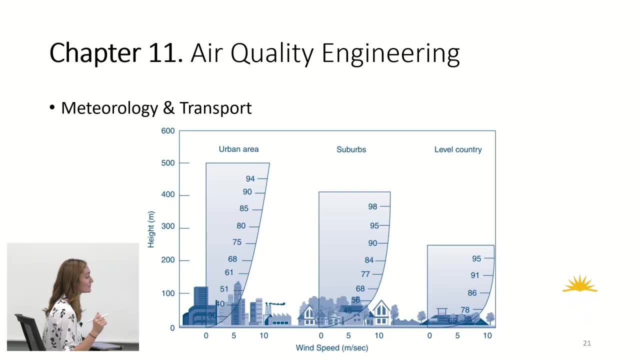 Speaker: 52 Speaker, 53 Speaker, 53 Speaker, 54 Speaker, 54 Speaker, 55 Speaker, 56 Speaker, 56 Speaker, 57 Speaker, 58 Speaker, 58 Speaker, 58 Speaker, 59 Speaker, 51 Speaker, 52 Speaker, 53 Speaker 53. 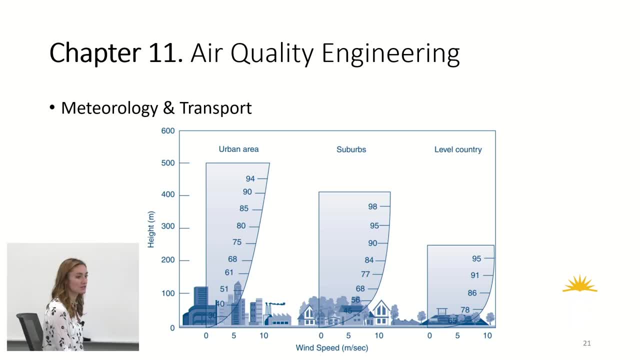 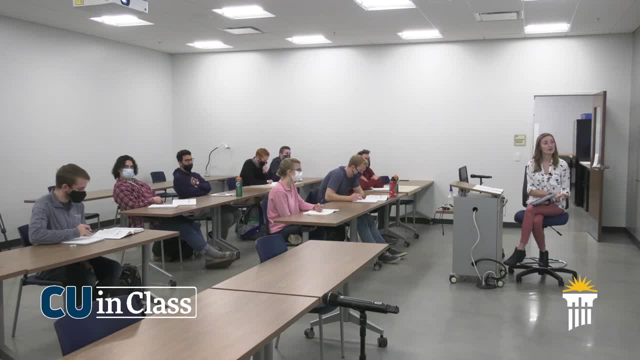 Speaker: 52 Speaker 53 Speaker, 53 Speaker, 53 Speaker. 54 Speaker, 53 Speaker. 54 Speaker, 55 Speaker. 56 Speaker 56 Speaker, 56 Speaker 57 Speaker. 57 Speaker 58 Speaker 56 Speaker. 57 Speaker 57. 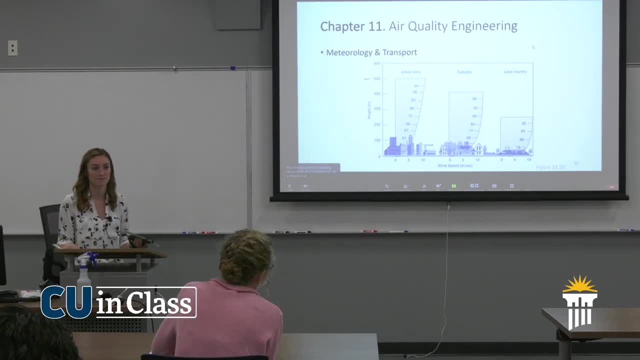 Speaker 58 Speaker 58 Speaker 58 Speaker 59 Speaker 52 Speaker 53 Speaker. 54 Speaker 56 Speaker 57 Speaker 58 Speaker 56 Speaker 57 Speaker 58 Speaker 58 Speaker 58 Speaker 59 Speaker 51. 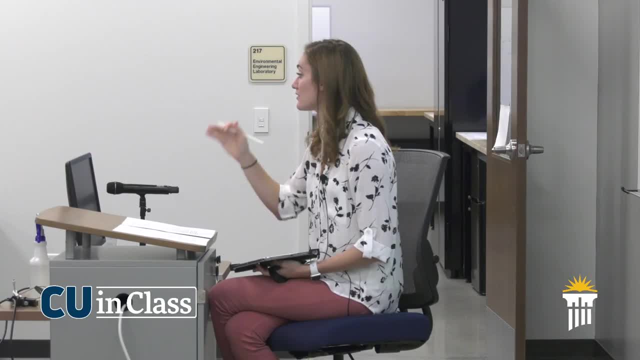 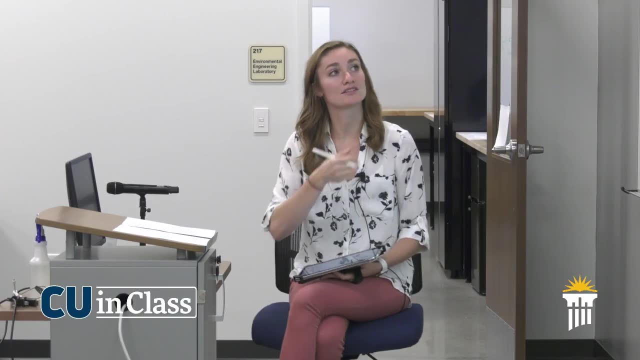 Speaker 52 Speaker 53 Speaker 53 Speaker. 54 Speaker 53 Speaker 54 Speaker, 54 Speaker, 55 Speaker. 56 Speaker 57 Speaker 56 Speaker 58 Speaker 58 Speaker 56 Speaker 58 Speaker. 49 Speaker 49. 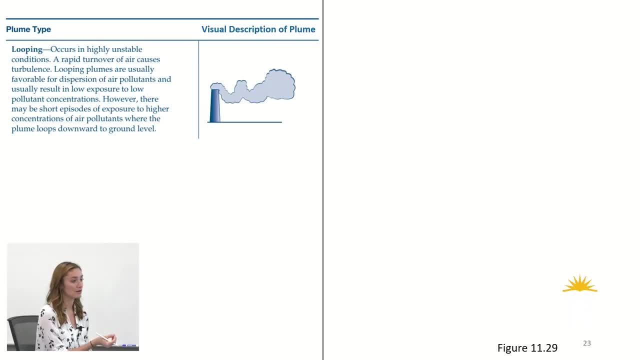 Speaker: 50 Speaker, 52 Speaker, 53 Speaker, 54 Speaker, 55 Speaker, 56 Speaker, 56 Speaker, 56 Speaker, 57 Speaker, 58 Speaker, 58 Speaker, 59 Speaker, 51 Speaker, 52 Speaker, 53 Speaker, 53 Speaker 54. 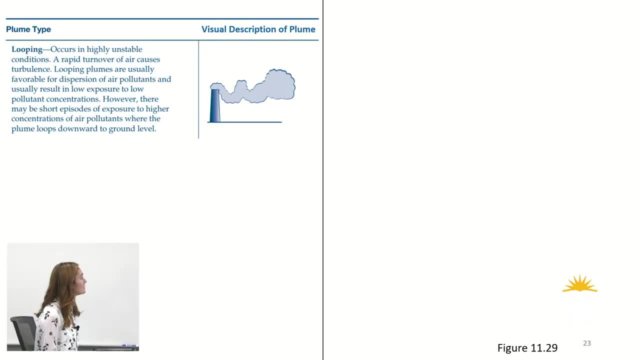 Speaker: 54 Speaker, 55 Speaker, 56 Speaker, 56 Speaker, 56 Speaker, 57 Speaker, 58 Speaker, 58 Speaker, 58 Speaker, 59 Speaker, 51 Speaker, 52 Speaker, 53 Speaker, 53 Speaker, 54 Speaker, 55 Speaker 56. 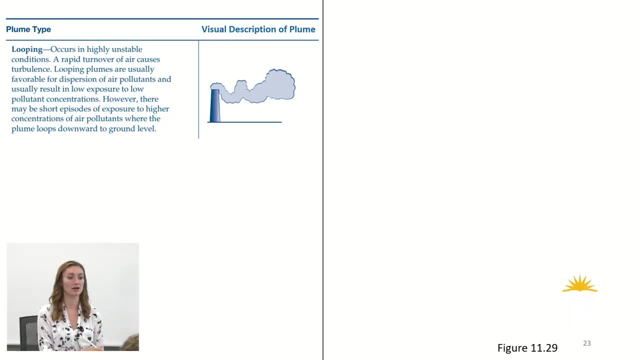 Speaker 56 Speaker 56 Speaker, 57 Speaker, 58 Speaker, 58 Speaker, 59 Speaker, 51 Speaker, 52 Speaker, 53 Speaker 53 Speaker 53 Speaker, 54 Speaker, 54 Speaker, 55 Speaker, 56 Speaker, 56 Speaker 56. 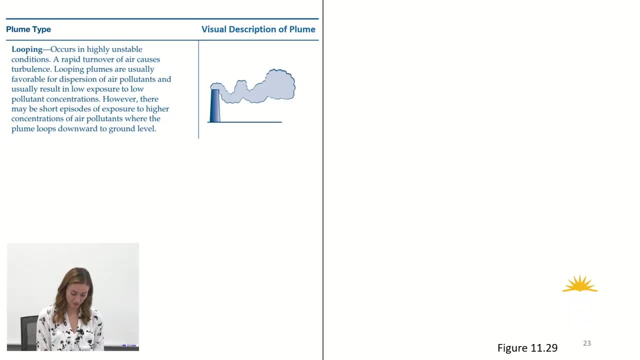 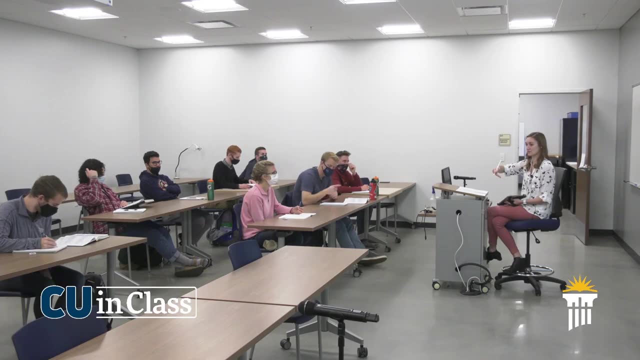 Speaker 57 Speaker 56 Speaker 57 Speaker, 58 Speaker, 58 Speaker, 58 Speaker, 59 Speaker, 52 Speaker. 53 Speaker 54 Speaker 55 Speaker 56 Speaker 56 Speaker 56 Speaker 57 Speaker, 58 Speaker 58. 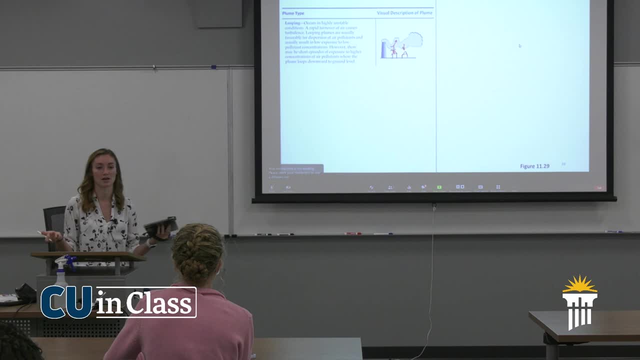 Speaker: 58 Speaker 59 Speaker, 51 Speaker, 52 Speaker, 53 Speaker, 53 Speaker, 54 Speaker, 53 Speaker, 54 Speaker 55 Speaker 56 Speaker 56 Speaker 56 Speaker 57 Speaker 57 Speaker, 58 Speaker 56. 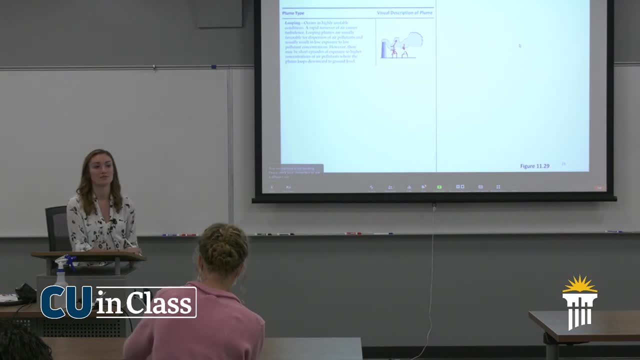 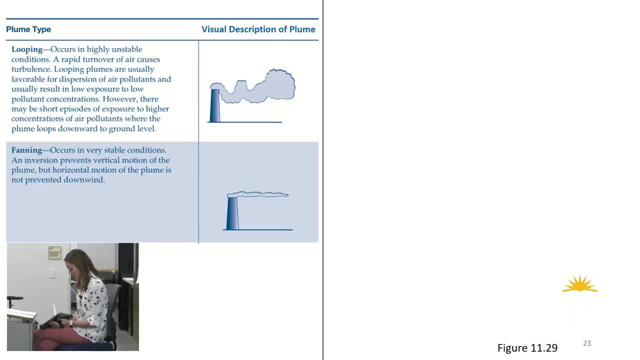 Speaker: 69 Speaker, 70 Speaker, 71 Speaker, 72 Speaker, 73 Speaker, 74 Speaker, 75 Speaker, 76 Speaker, 76 Speaker, 77 Speaker, 78 Speaker, 79 Speaker, 79 Speaker, 80 Speaker, 92 Speaker, 92 Speaker 93. 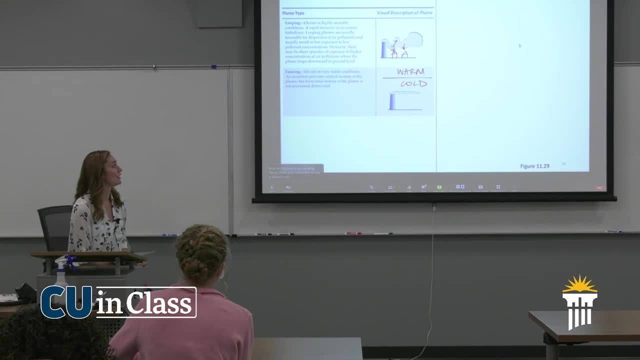 Speaker: 93 Speaker 93 Speaker, 94 Speaker, 94 Speaker, 95 Speaker, 96 Speaker, 97 Speaker, 98 Speaker, 99 Speaker, 100 Speaker, 100 Speaker, 12 Speaker, 12 Speaker, 13 Speaker, 13 Speaker, 14 Speaker 15. 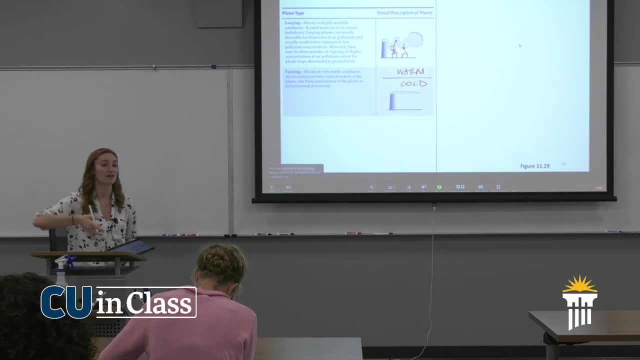 Speaker: 16 Speaker 17 Speaker 18 Speaker, 19 Speaker 21 Speaker 22 Speaker, 23 Speaker 24 Speaker. 25 Speaker 26 Speaker 27 Speaker 28 Speaker, 29 Speaker 30 Speaker 31 Speaker, 32 Speaker 33. 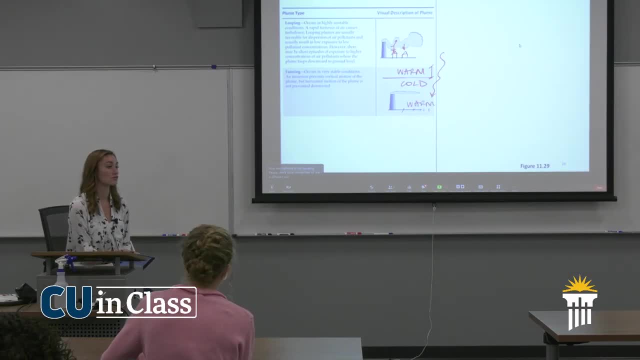 Speaker: 34 Speaker, 35 Speaker, 36 Speaker, 37 Speaker, 38 Speaker, 39 Speaker, 40 Speaker, 41 Speaker, 42 Speaker, 43 Speaker, 44 Speaker, 45 Speaker, 46 Speaker, 47 Speaker, 48 Speaker, 49 Speaker 50. 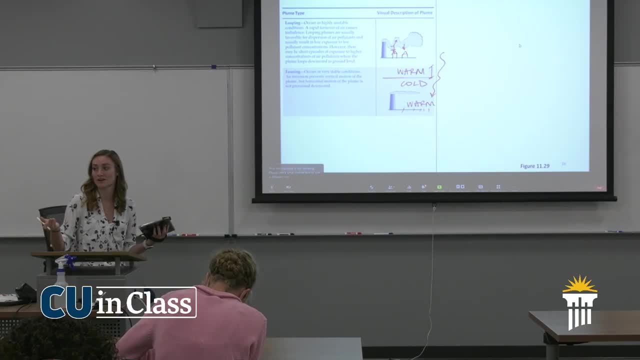 Speaker: 51 Speaker 52 Speaker, 53 Speaker, 54 Speaker, 55 Speaker, 56 Speaker, 56 Speaker, 57 Speaker, 58 Speaker 58 Speaker 51 Speaker, 52 Speaker, 53 Speaker, 54 Speaker, 55 Speaker, 56 Speaker 56. 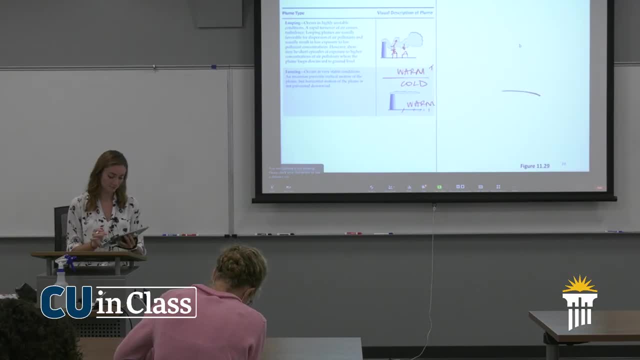 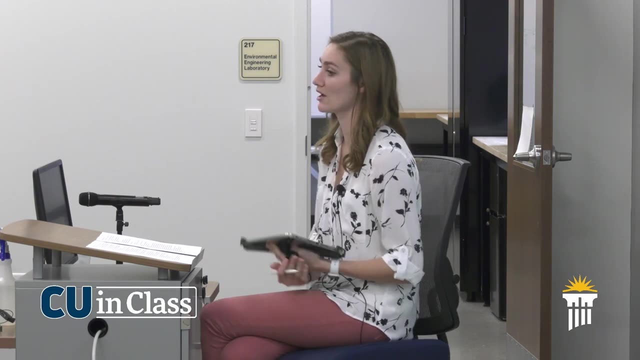 Speaker: 57 Speaker 58 Speaker, 49 Speaker, 50 Speaker, 51 Speaker, 52 Speaker, 53 Speaker, 54 Speaker. 55 Speaker 56 Speaker, 56 Speaker, 56 Speaker, 57 Speaker, 58 Speaker 51 Speaker, 52 Speaker 53. 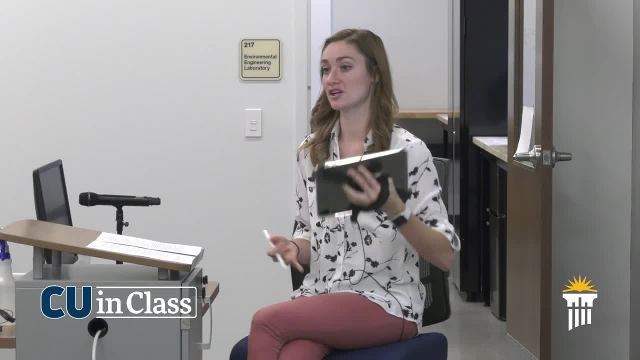 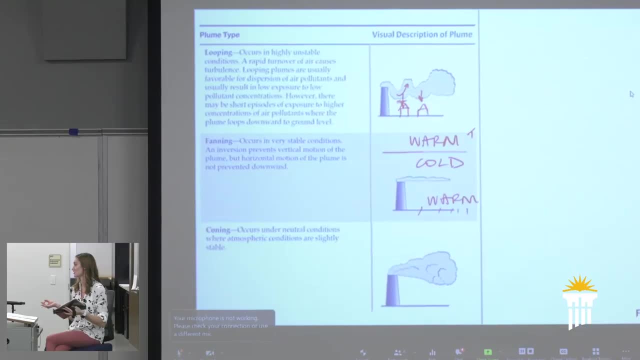 Speaker: 53 Speaker, 54 Speaker, 54 Speaker, 56 Speaker, 57 Speaker, 58 Speaker, 58 Speaker, 59 Speaker, 51 Speaker, 52 Speaker. 53 Speaker, 53 Speaker, 54 Speaker, 54 Speaker, 55 Speaker, 56 Speaker 56. 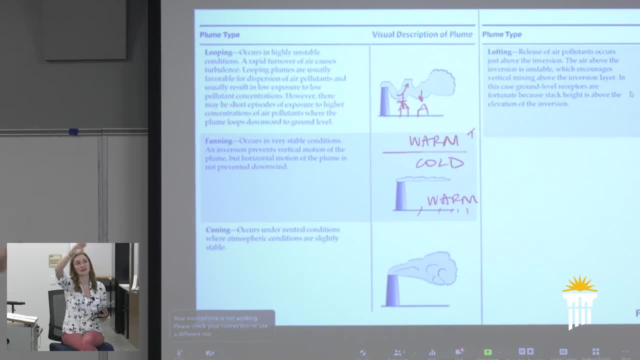 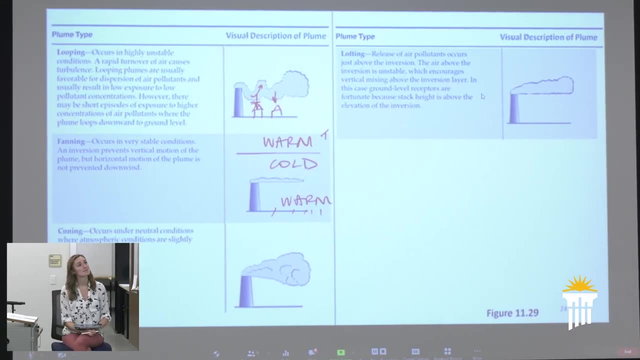 Speaker: 57 Speaker 58 Speaker, 59 Speaker, 51 Speaker, 52 Speaker, 53 Speaker. 53 Speaker. 54 Speaker. 54 Speaker. 56 Speaker, 56 Speaker, 57 Speaker, 58 Speaker, 58 Speaker, 51 Speaker, 52 Speaker 53. 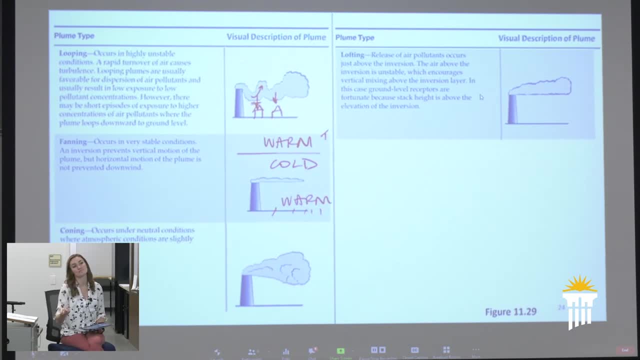 Speaker: 54 Speaker, 55 Speaker, 56 Speaker, 56 Speaker, 56 Speaker, 57 Speaker, 58 Speaker, 58 Speaker, 59 Speaker, 51 Speaker, 52 Speaker, 53 Speaker, 53 Speaker, 54 Speaker, 53 Speaker, 54 Speaker 54. 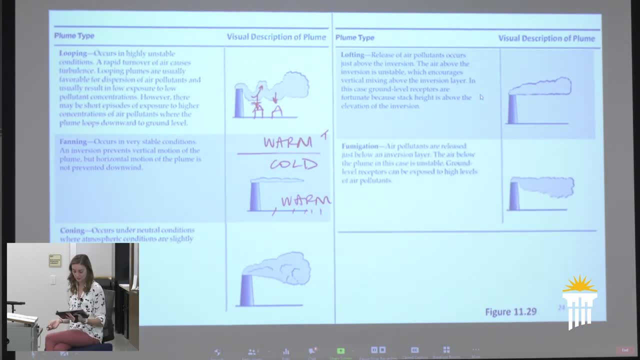 Speaker 55 Speaker 56 Speaker 56 Speaker 56 Speaker 57 Speaker 56 Speaker 57 Speaker, 58 Speaker 58 Speaker 58 Speaker 59 Speaker 52 Speaker 53 Speaker 56 Speaker 56 Speaker, 57 Speaker 58. 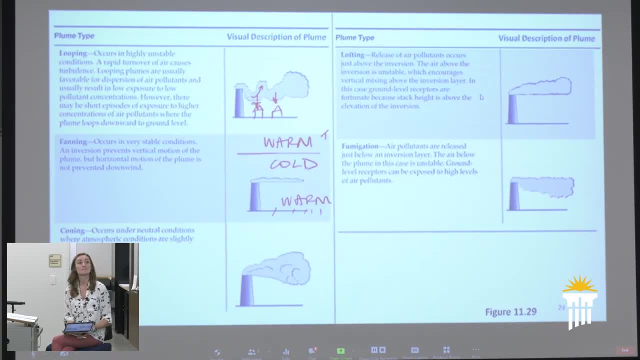 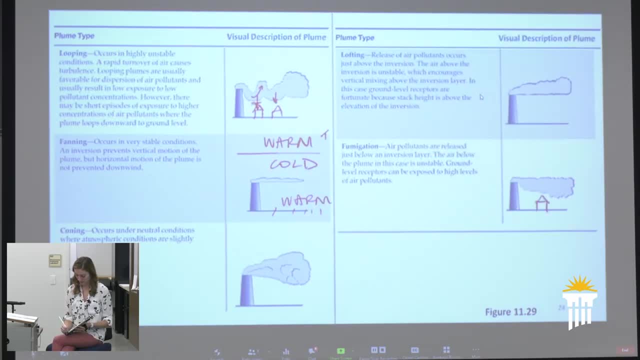 Speaker 57 Speaker 58 Speaker, 58 Speaker, 58 Speaker, 59 Speaker, 52 Speaker, 53 Speaker, 54 Speaker. 55 Speaker. 56 Speaker. 56 Speaker. 56 Speaker, 57 Speaker. 58 Speaker, 58 Speaker, 58 Speaker 59. 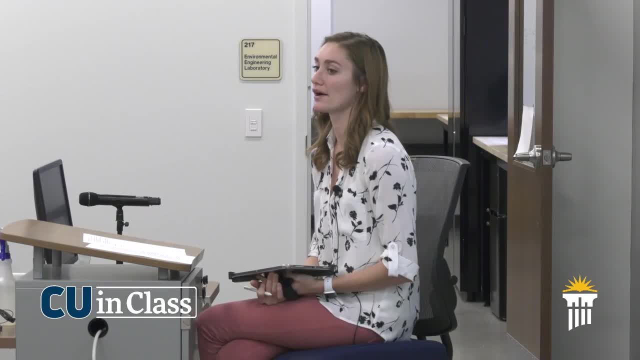 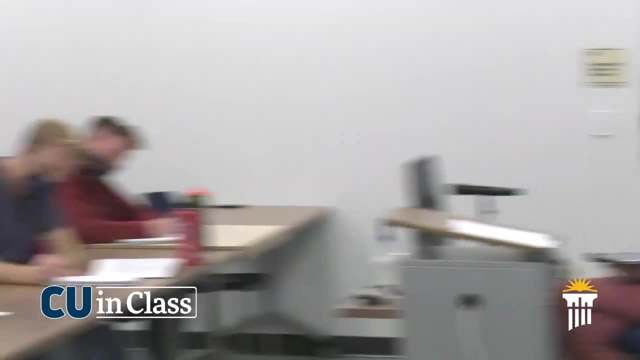 Speaker: 51 Speaker, 52 Speaker, 53 Speaker, 53 Speaker, 54 Speaker, 53 Speaker, 54 Speaker, 55 Speaker, 56 Speaker, 56 Speaker, 56 Speaker, 57 Speaker, 57 Speaker, 58 Speaker, 58 Speaker, 58 Speaker 59. 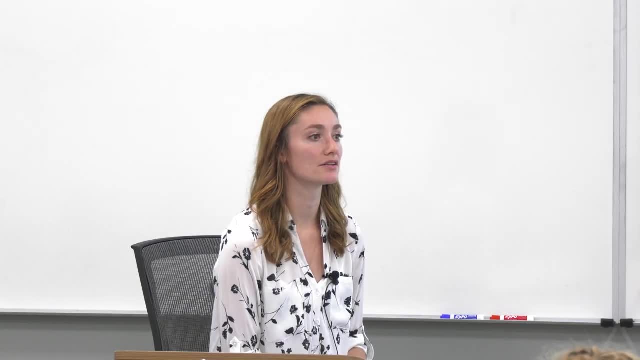 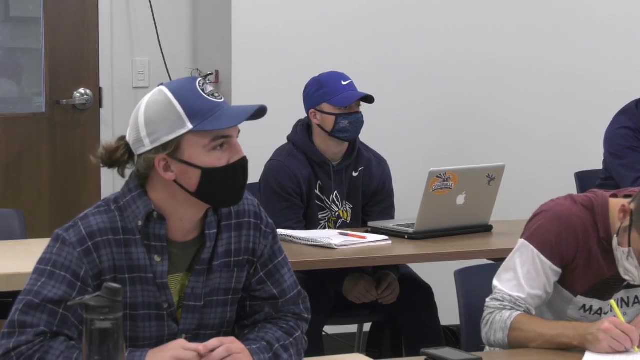 Speaker: 51 Speaker 52 Speaker, 53 Speaker, 53 Speaker, 54 Speaker, 54 Speaker, 55 Speaker, 56 Speaker. 56 Speaker. 56 Speaker, 57 Speaker, 58 Speaker, 58 Speaker, 59 Speaker. 51 Speaker, 52 Speaker 53. 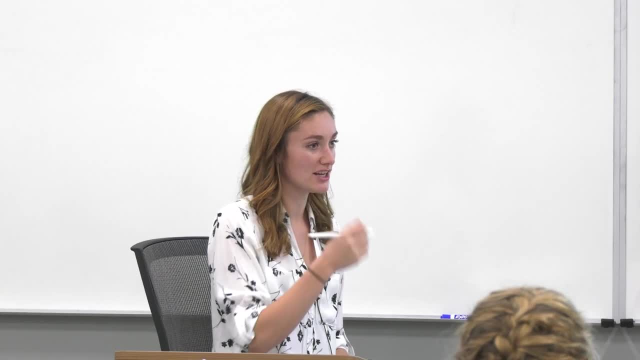 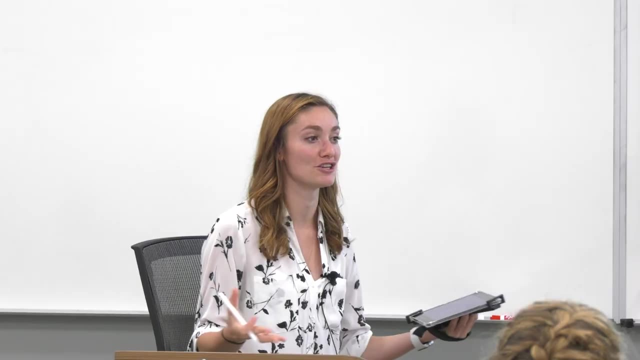 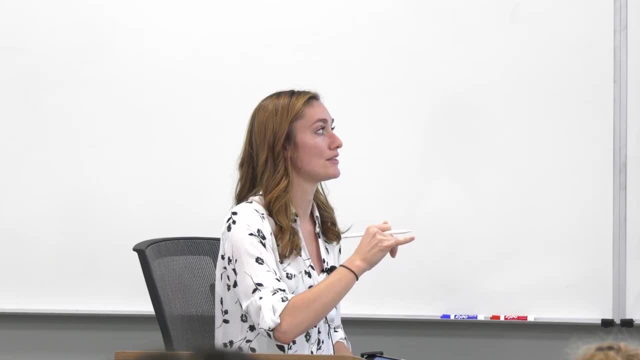 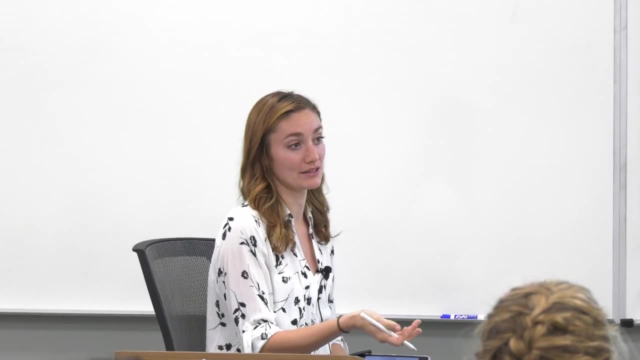 Speaker: 60 Speaker, 61 Speaker, 62 Speaker, 63 Speaker, 64 Speaker, 65 Speaker, 67 Speaker, 68 Speaker, 69 Speaker, 69 Speaker, 70 Speaker, 71 Speaker, 72 Speaker, 73 Speaker, 74 Speaker, 75 Speaker 76. 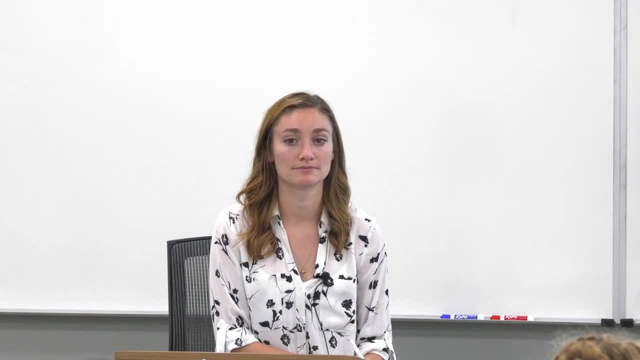 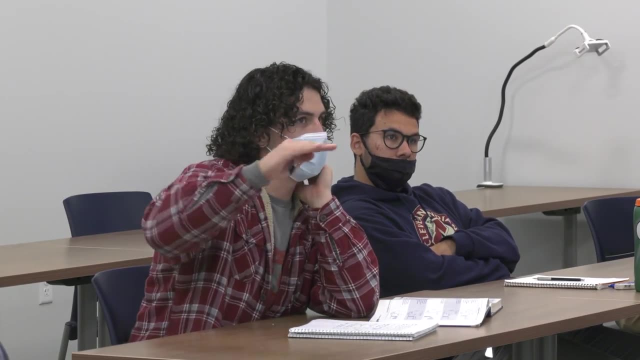 Speaker 76 Speaker 77 Speaker 78 Speaker 79 Speaker 79 Speaker 80 Speaker 92 Speaker 93 Speaker 93 Speaker 94 Speaker 94 Speaker 95 Speaker 96 Speaker 96 Speaker 96 Speaker 97 Speaker 98. 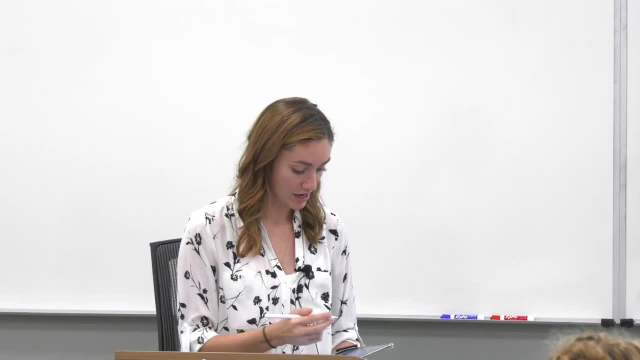 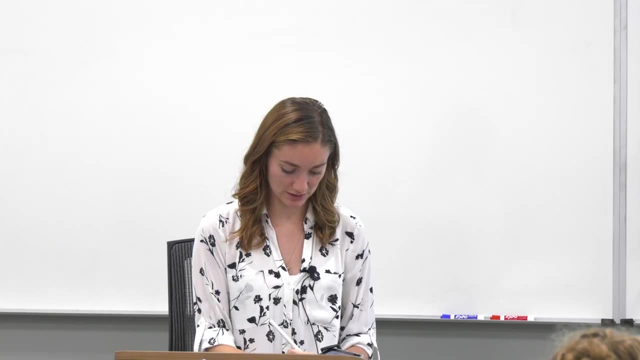 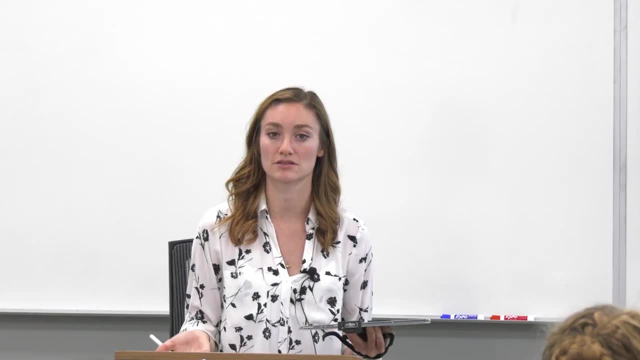 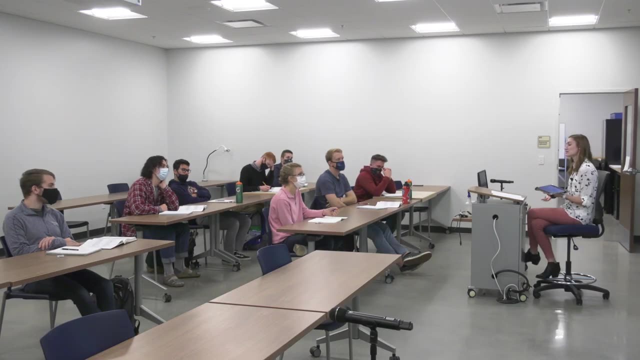 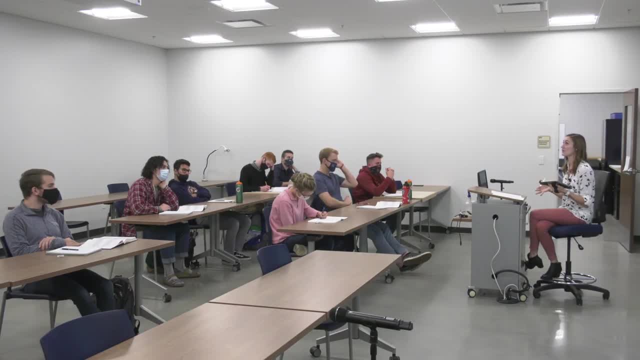 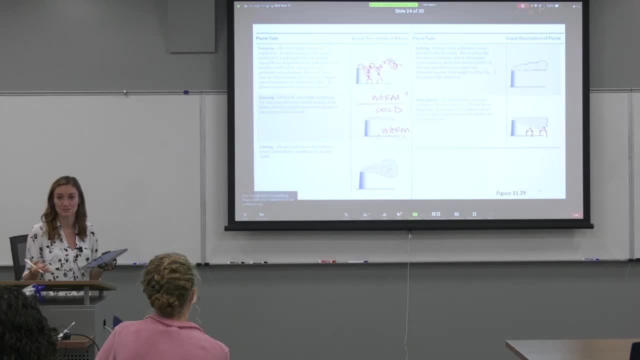 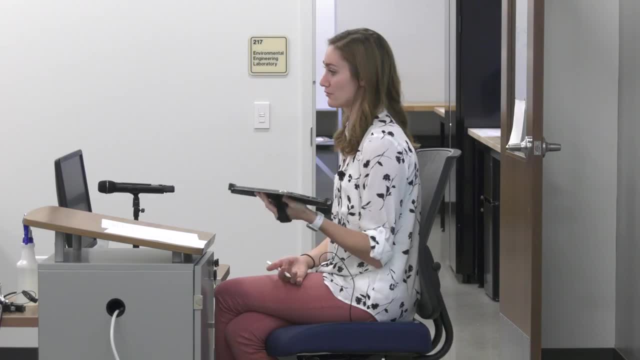 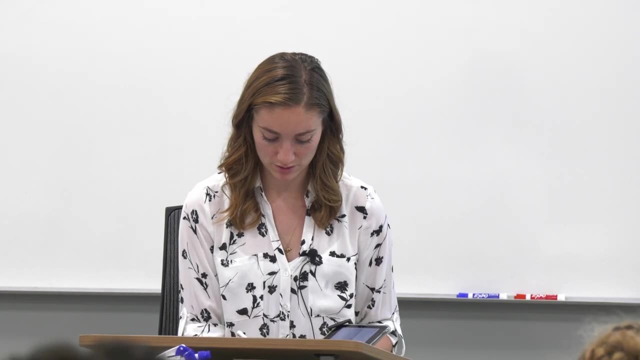 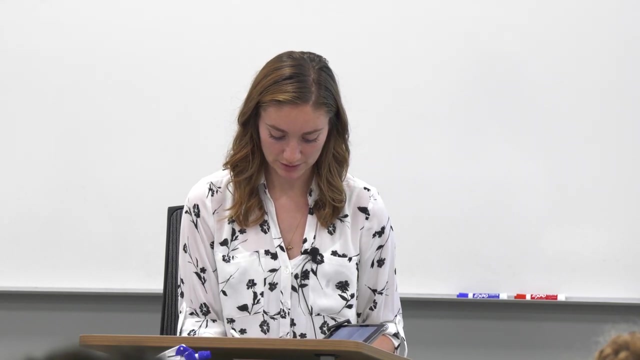 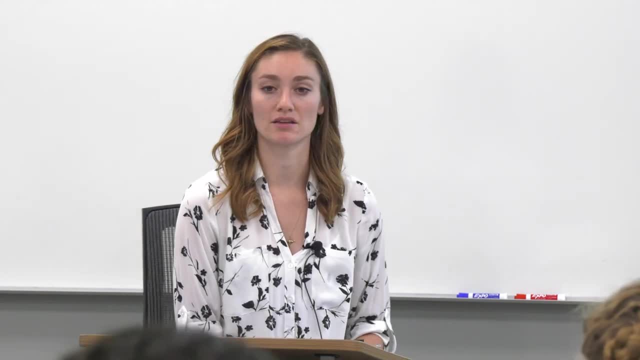 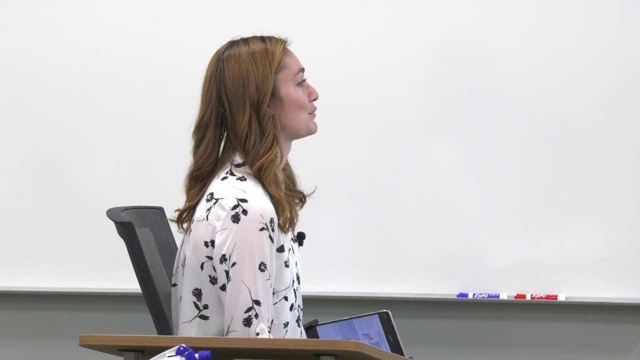 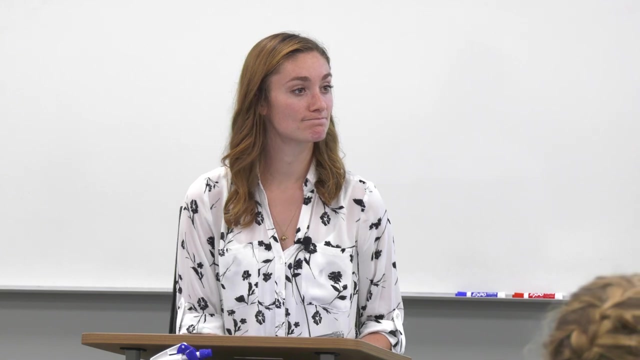 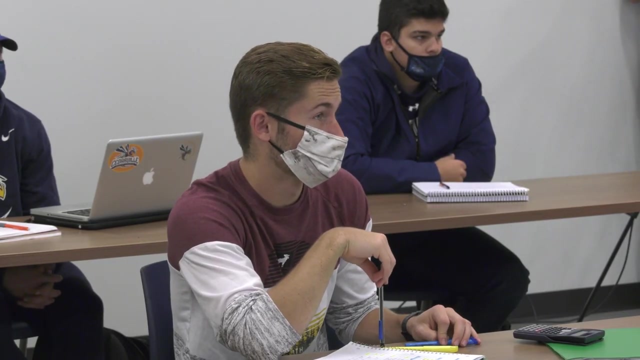 and our warmer air below, because as we're heating the earth with the Sun, we don't do it, the Lord does. it is that as the Sun heats the earth, we tend to have warm air below and cold air above. yes, so it kind of depends. it depends on where people's homes are or how big. 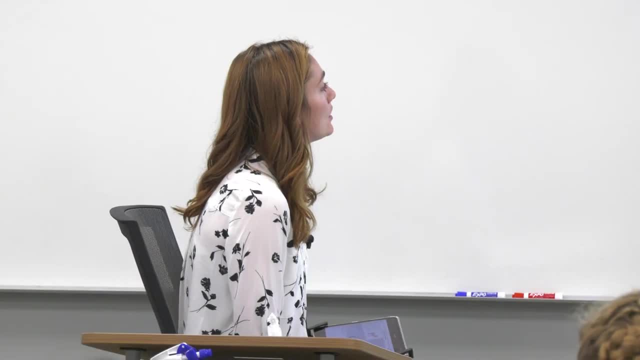 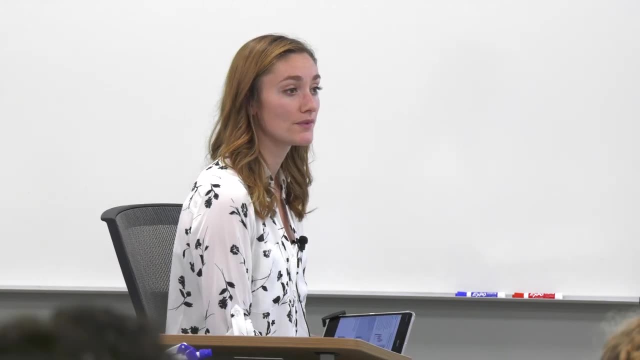 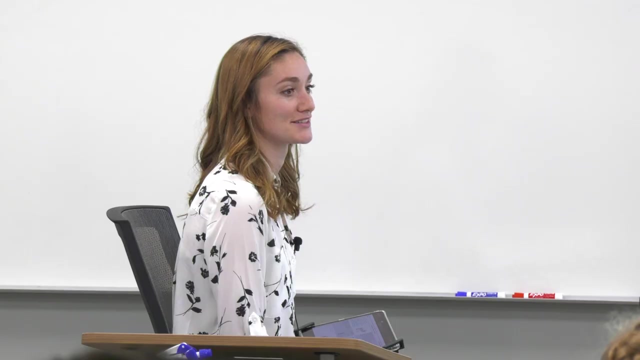 your city is kind of what you're dealing with. coning is the least favorable. coning and fumigation are probably the least favorable. coning mostly because it's uncertain, and fumigation because if people live close there's no chance for them to be like. there's no like out of sight, out of mind, it is in your face and 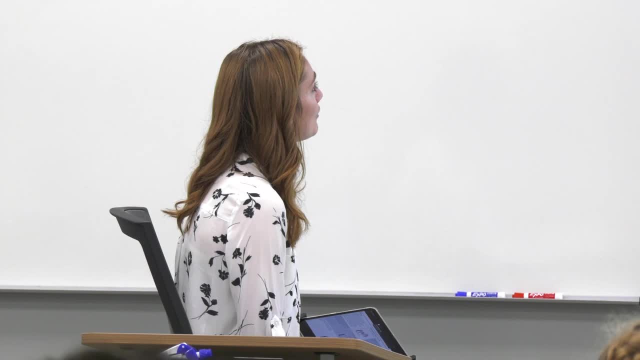 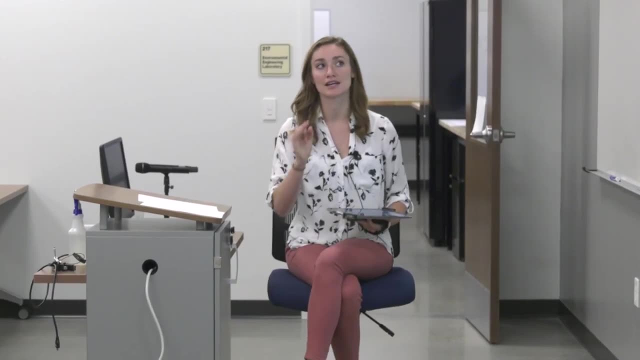 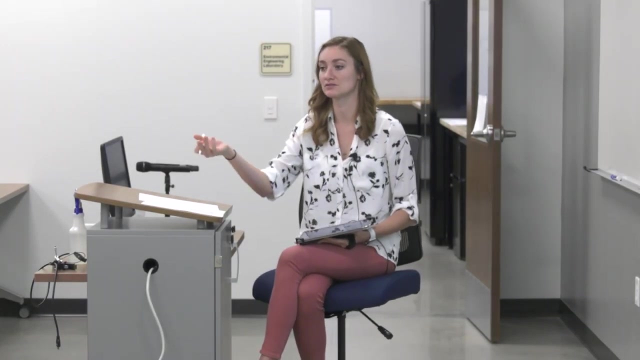 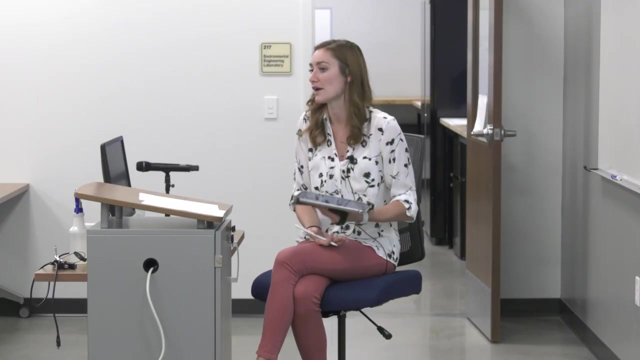 then fanning. fanning can be okay, it depends on how far it's gonna go, and fanning and lofting actually tend to look pretty similar, but I'd say probably looping is the most favorable, mostly because it hits everybody relatively equally, so nobody gets really high dosages of any particular concentration of particulate. 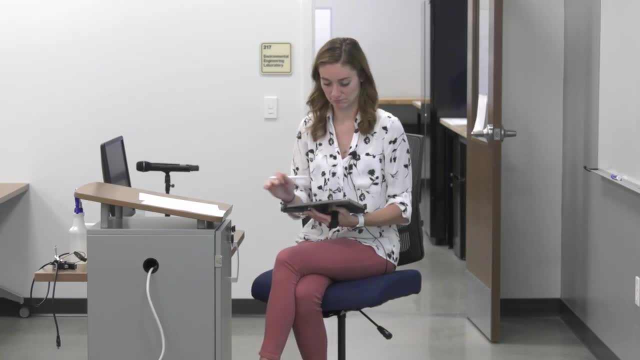 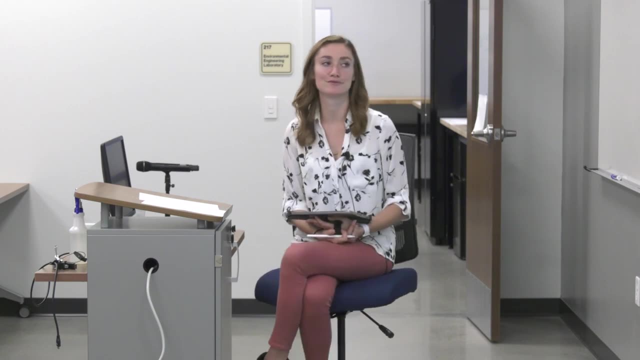 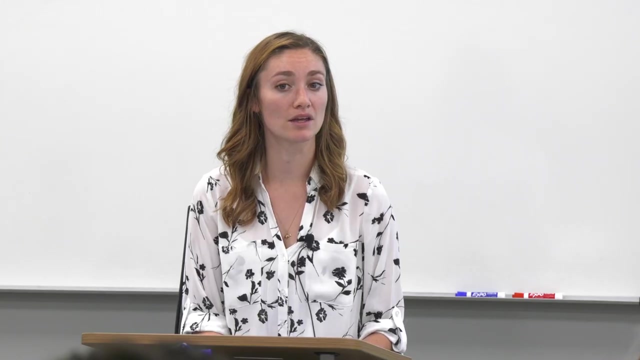 matter, something like that. so, yeah, I'd say that's looping is probably your most favorable, with fanning and lofting coming in kind of like a second place and then fumigation and coning coming in a definite last. yeah, so on Monday we will talk about how to do analysis and 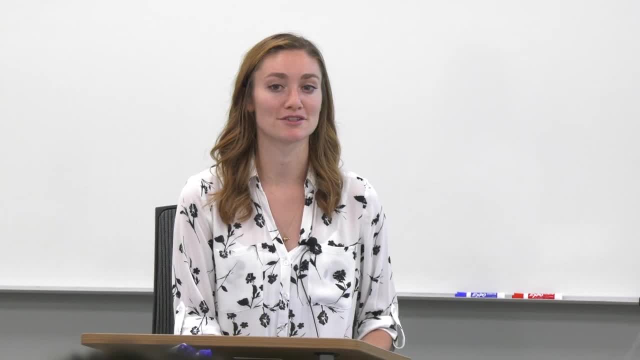 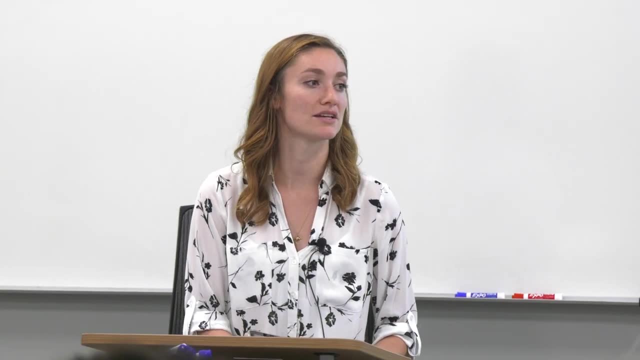 assessment. so we'll do Gaussian distributions so you can look forward to doing some math. could probably also look forward to doing a quiz on Monday, because we didn't get one in for solid waste, so that's something to look forward to. any other questions, any other online questions? I see you're chatting. 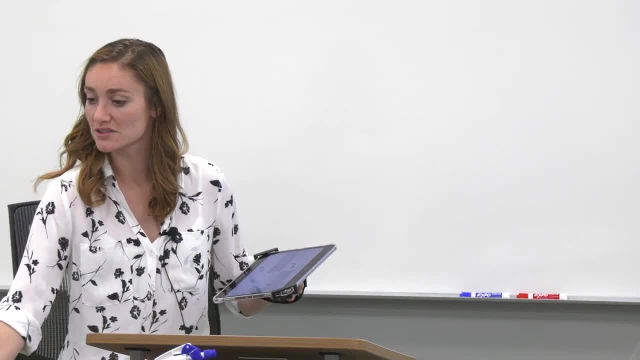 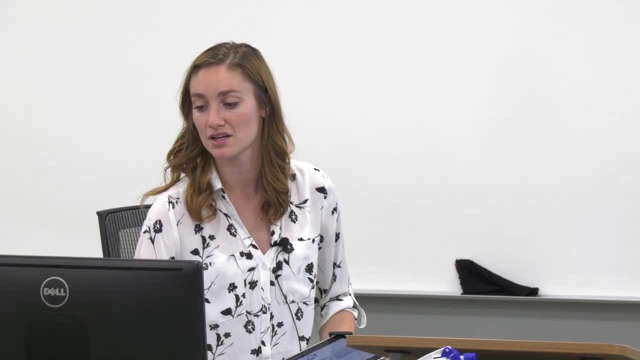 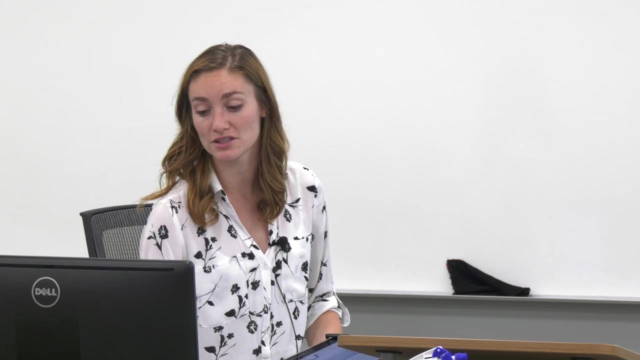 down here but I did not actually see them. most of Isaiah had as a and grace had comments on when we were talking about the co2 in the atmosphere. so grace called them the doldrums, which is true, and then most of the southern hemisphere is oceans and the oceans do absorb co2 that actually ends up contributing to.